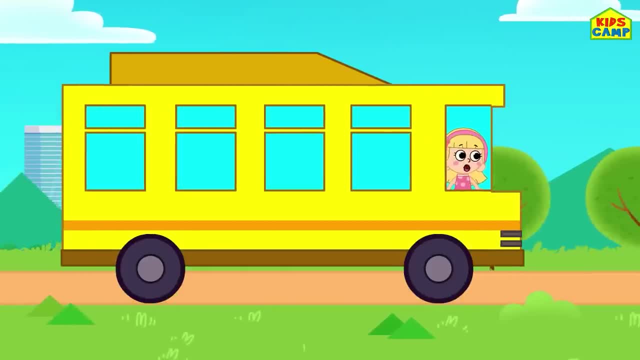 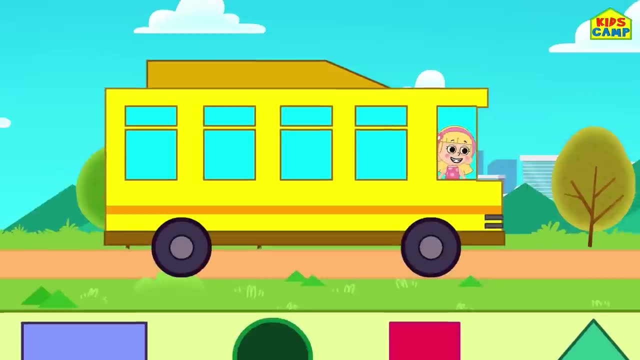 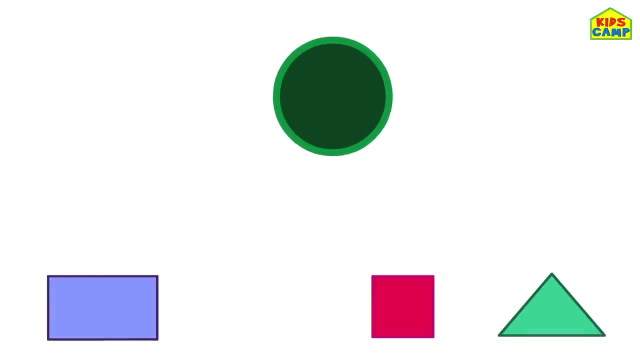 A bus, Just a one, bam. Wheels in the bus go Round and round, Round and round, Round and round. Wheels in the bus go Round and round. All-day long Circle goes round and round, Round and round, Round and round. 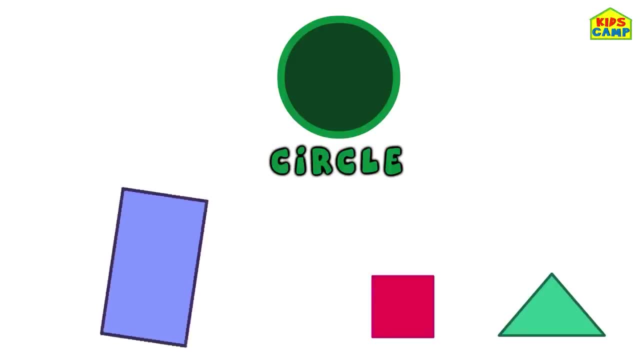 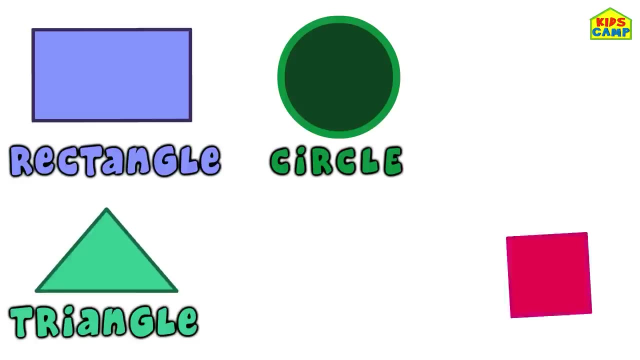 Rectangle. it has four sides. Opposites are the same. Triangle has three sides- Equals sides with three sides. Square has four equal sides- Equals sides with two sides. Rows doesn't change. It turns on only when it's in motion. 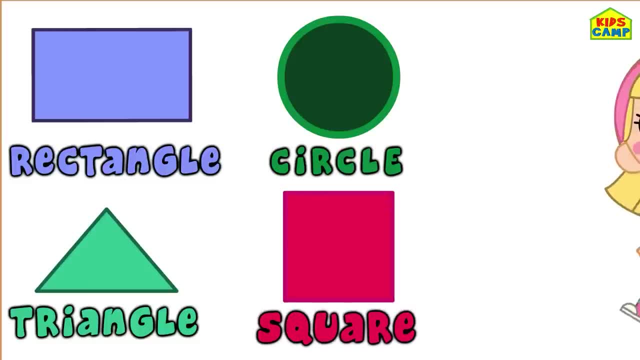 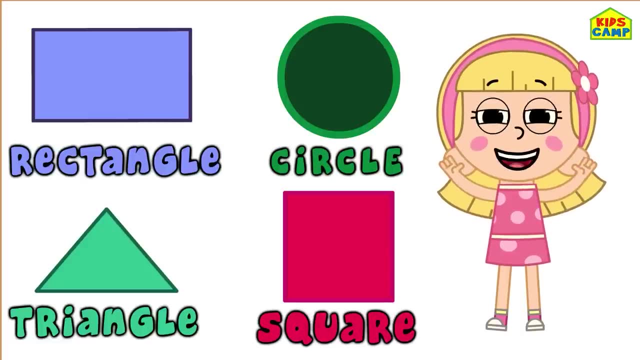 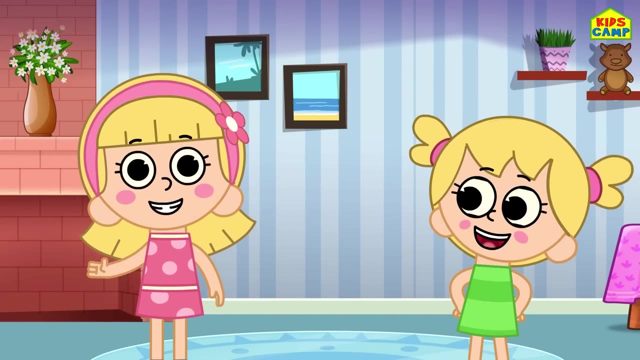 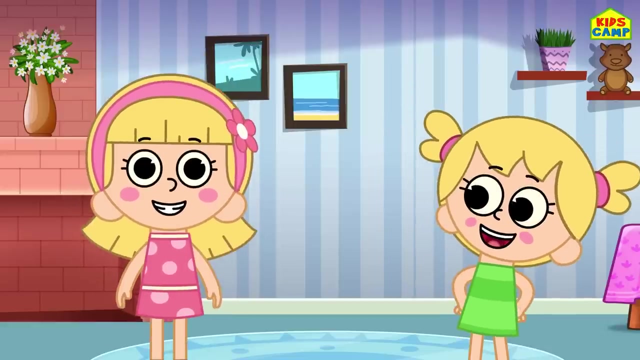 All the sides are same. Yay, I love the shapes. Hope you love them too. This was super fun. Bye-bye, Hi kids. I'm Ellie and this is Eva, And today we are going to have a party. Yay. 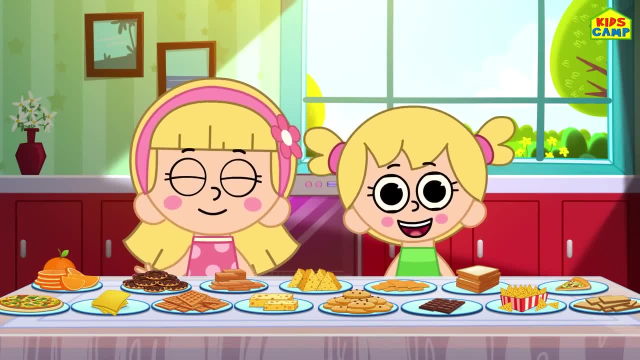 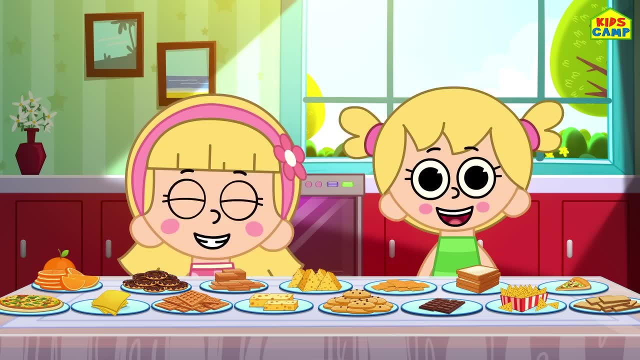 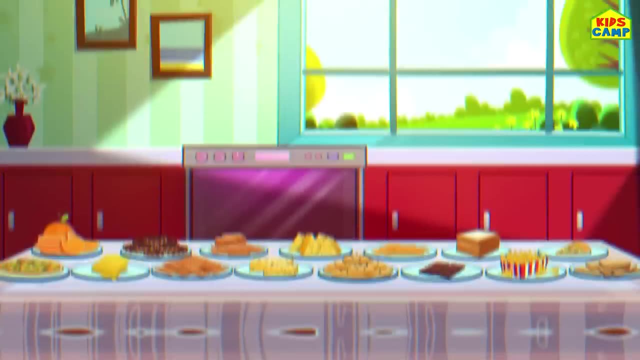 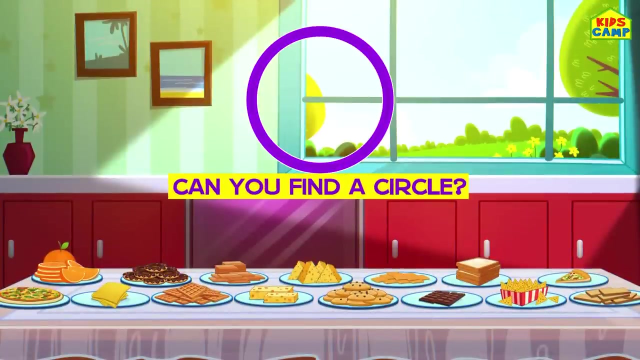 Ooh, Look at all this food- So delicious. We are also going to learn our shapes. Ready, Eva. Let's match the shapes with the food Circle. Can you find a circle? Where's a circle? What food is the shape of a circle? 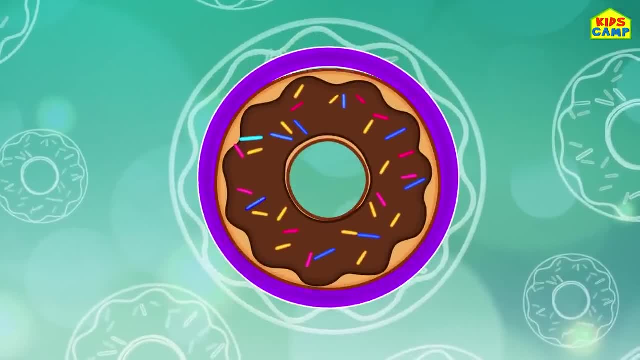 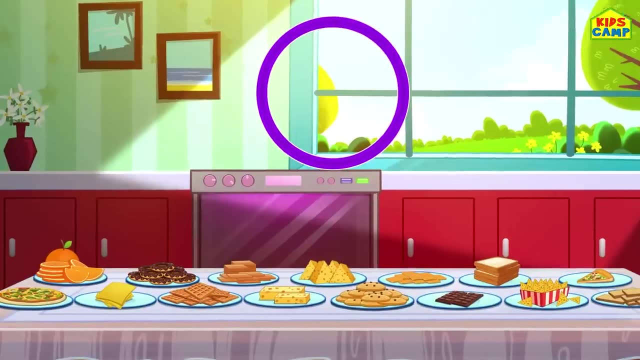 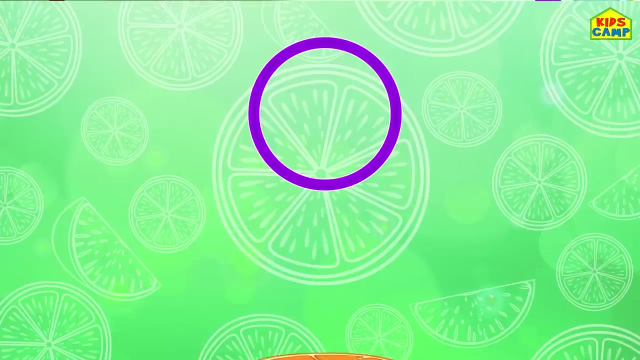 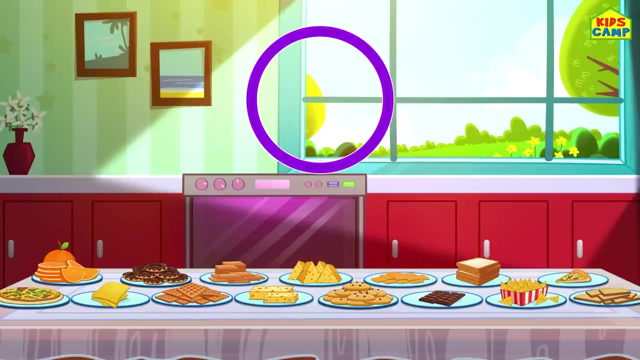 That's right, A doughnut. A doughnut is in the shape of a circle. What else? Hmm, That's right, An orange slice. Woohoo, An orange slice is also a circle. What else can we find? That's a circle. 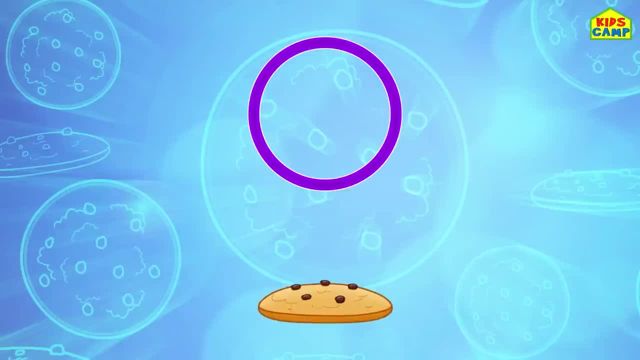 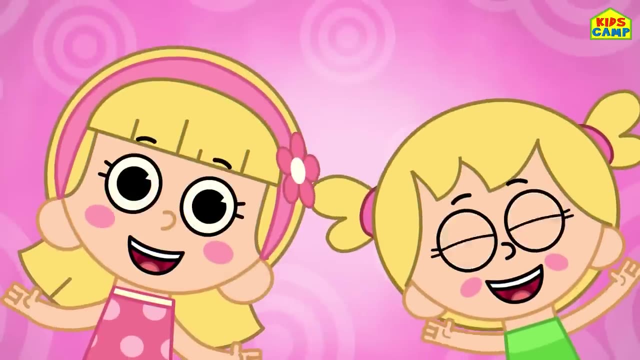 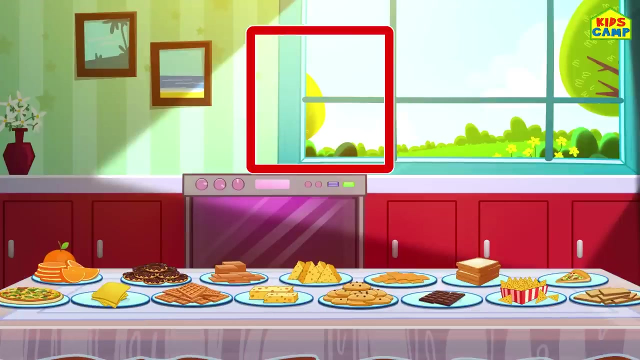 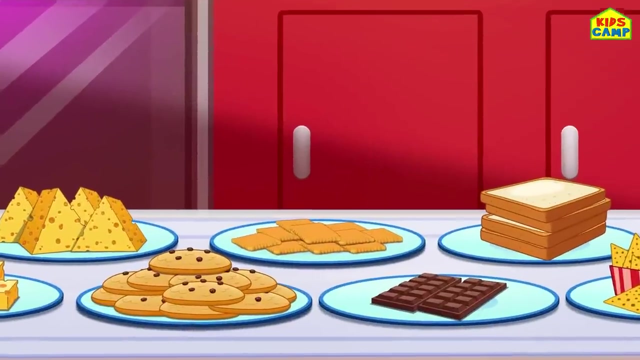 Hmm, A cookie. Yummy, A cookie is also a circle. Yay, What's the next shape? A square. Hmm, Can you find a square? kids, What food is in the shape of a square? Hmm, That's right, A craggle. 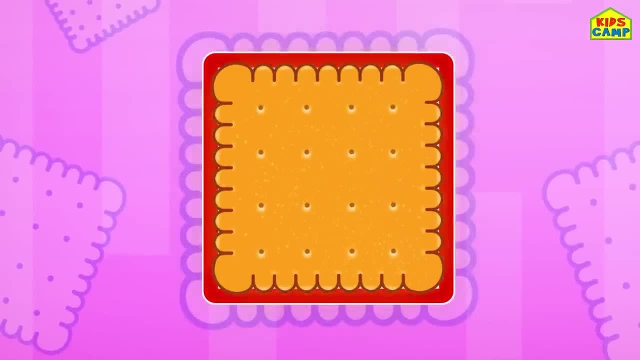 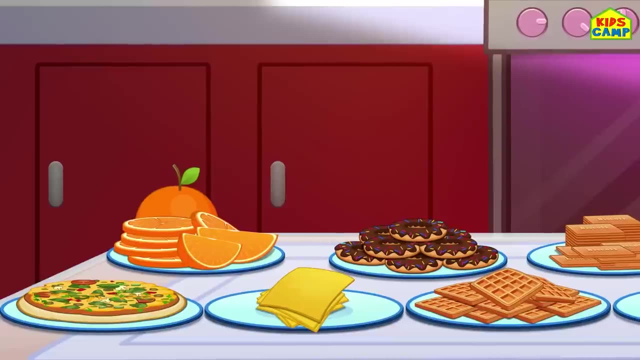 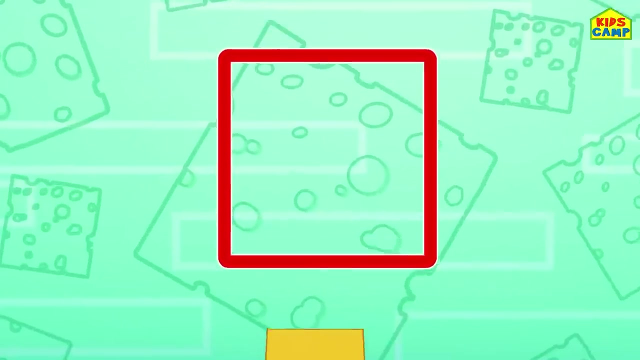 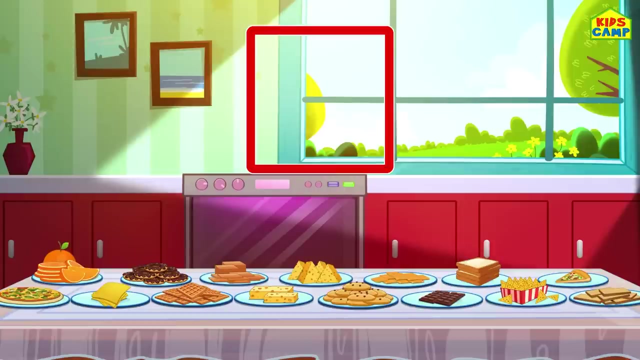 Yummy, That's the shape of a square. What else can we find That's a square? Uh-huh, A slice of cheese, That's right, A slice of cheese is also a square. What else is a square? Uh-huh? 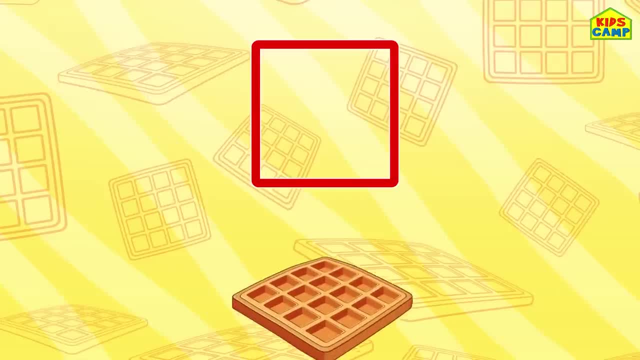 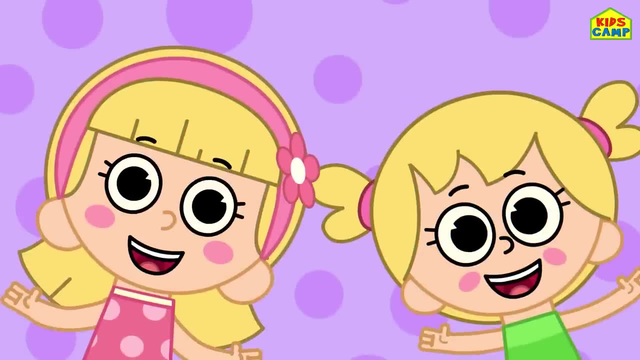 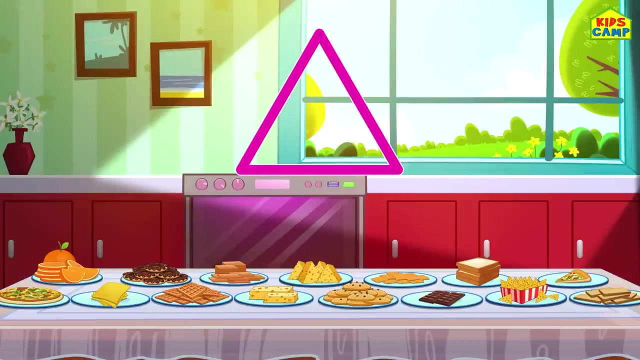 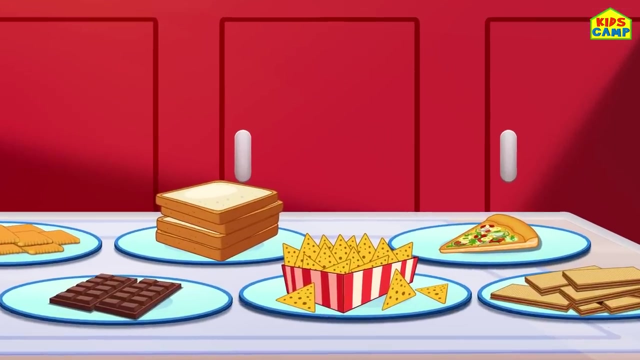 I see it. A waffle- Yay, A waffle is in the shape of a square- Yay. What's the next shape? A triangle. Can you find a triangle? Hmm, Do you see it? I see it too. 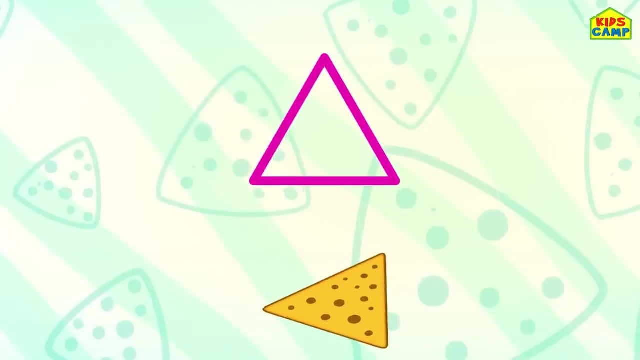 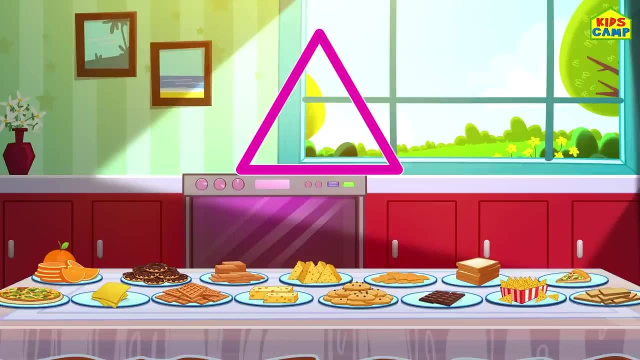 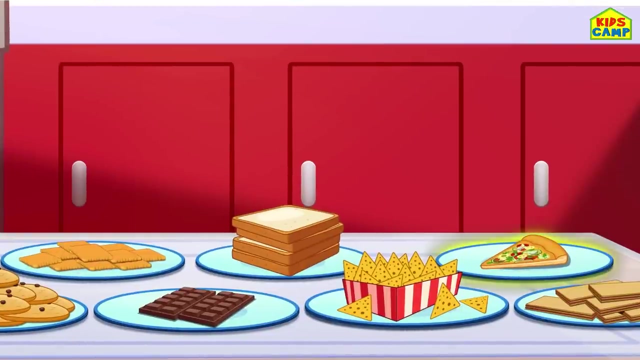 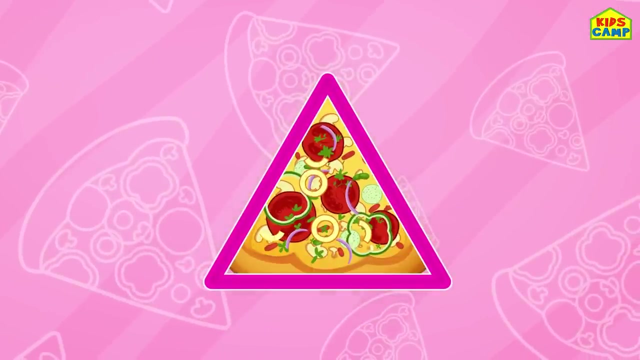 Nachos- Yay, A nacho is in the shape of a triangle. What else, That's right? Everyone's favourite. A slice of pizza? Yay, Woohoo, That sure is a triangle. Yay, What's the next shape? 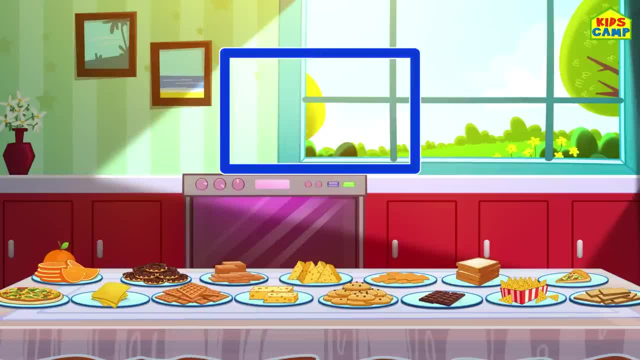 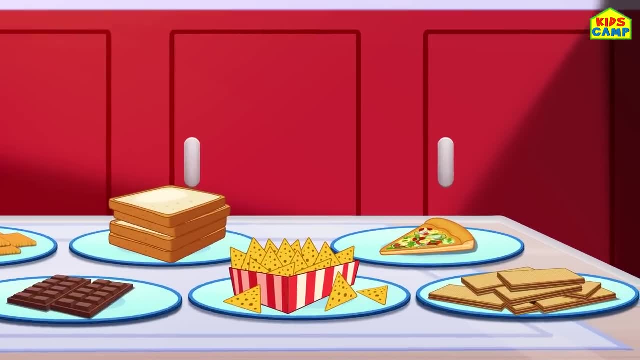 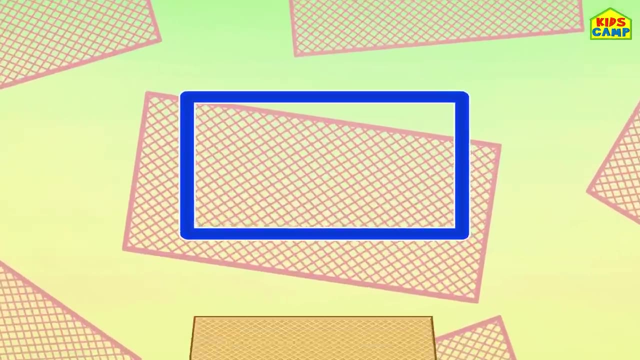 A rectangle, That's right. That's a slice of pizza, Yay, What else A rectangle? Can you find a rectangle, kids? Hmm, Ah, I see it too. A chocolate wafer. That's right, That also is a rectangle. 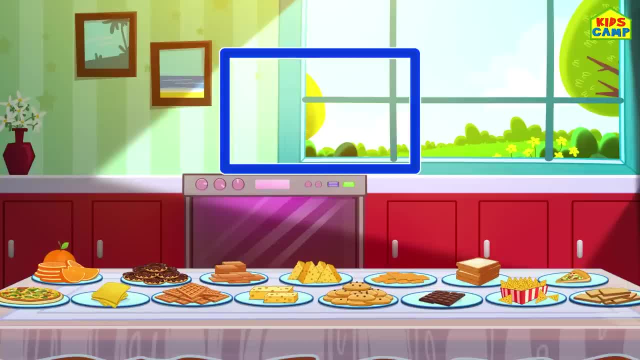 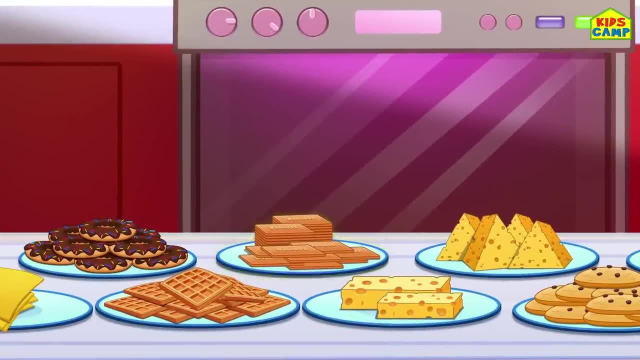 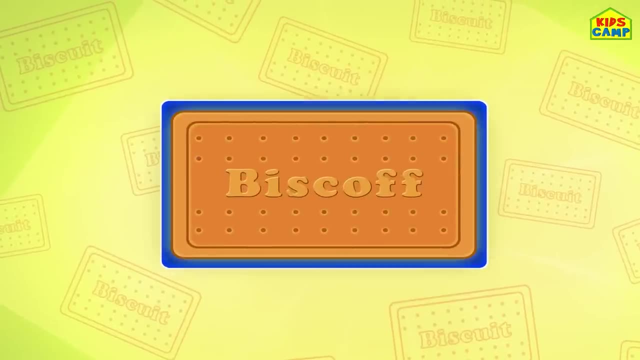 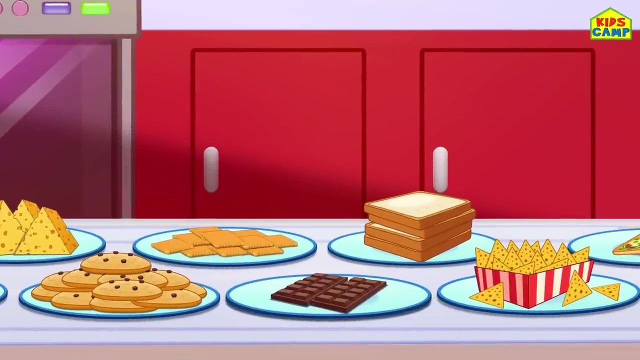 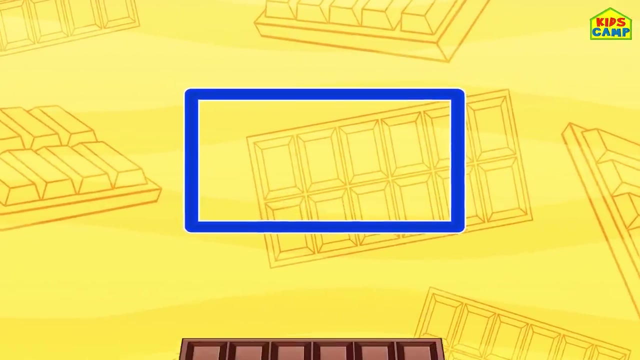 Yay, What else? Hmm, What's that? Yummy Biscuit? That sure is the shape of a rectangle. Anything else? Uh-huh, Chocolate, Woohoo, A bar of chocolate. That's right, kids. 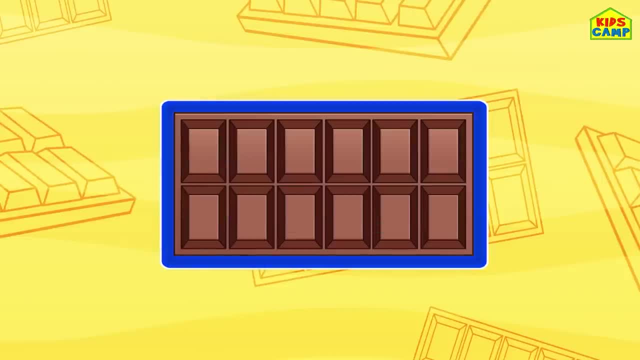 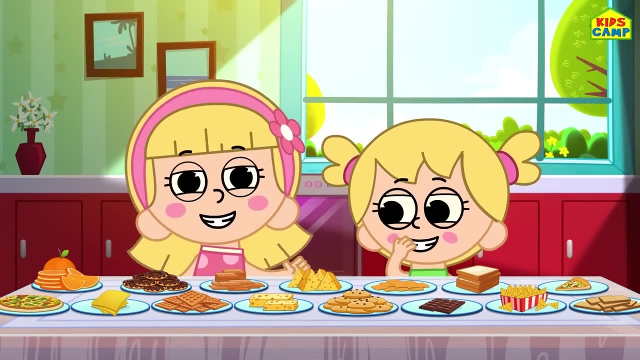 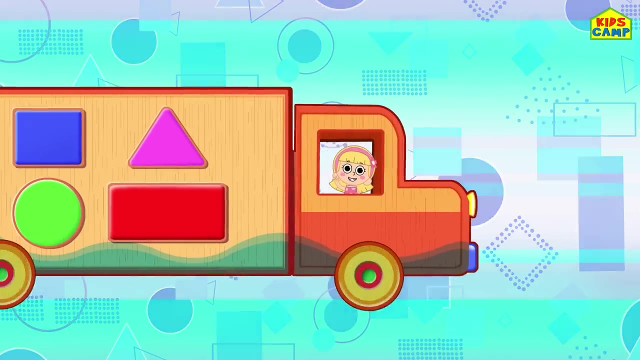 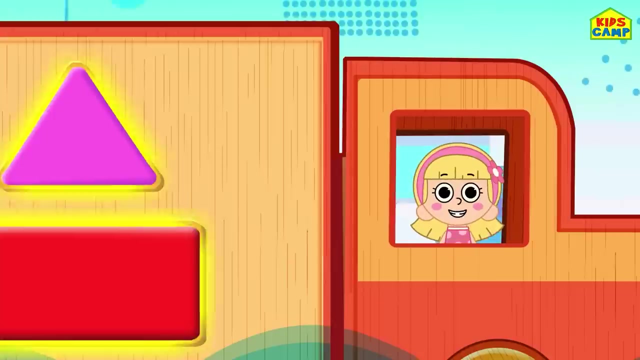 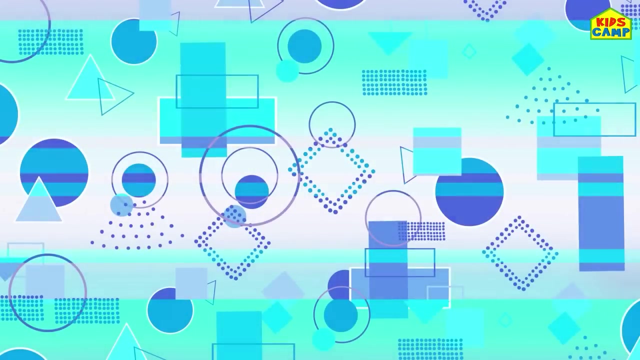 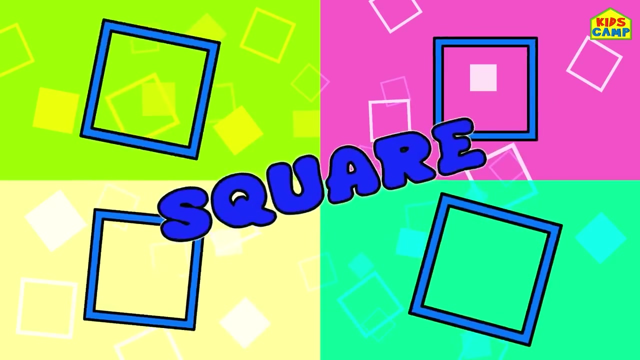 We did it. This all looks so good And we found all the shapes. Good job, Eva. Good job kids. Bye-bye. What kind of shape is this? What kind of shape is this Square? Square? This window is a square. 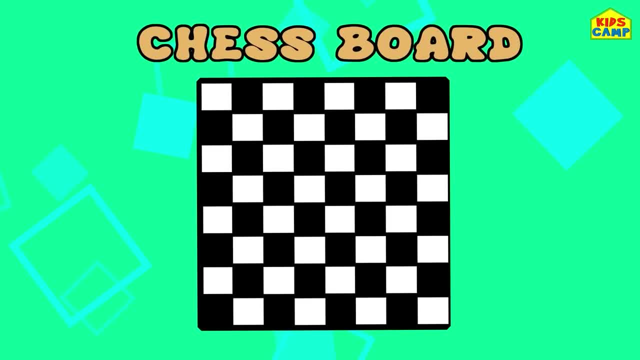 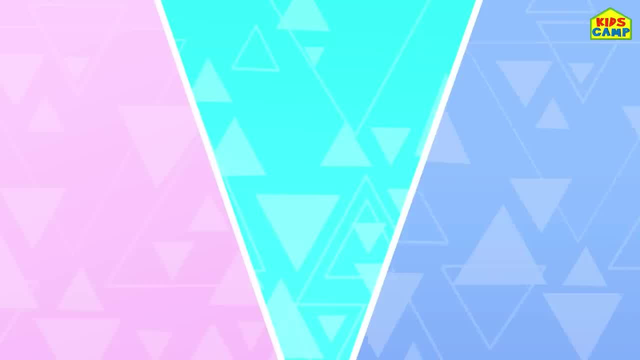 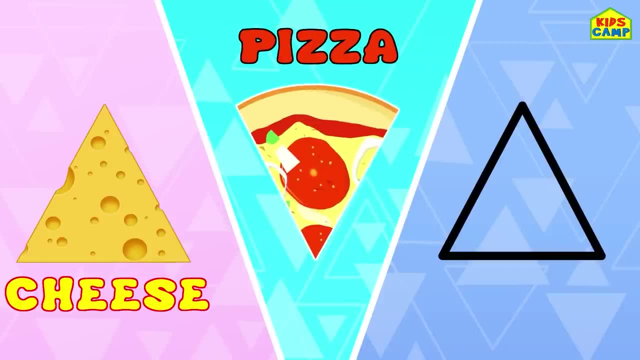 Like a cracker And a chessboard. This is a square. Squares are everywhere. What kind of shape is this? What kind of shape is this Triangle Triangle? This cheese is a triangle, Like a pizza, Like a rooftop. 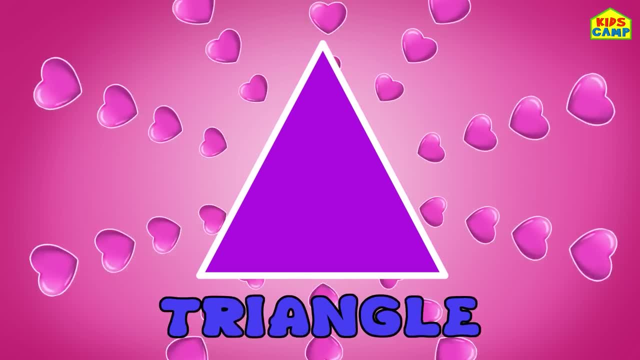 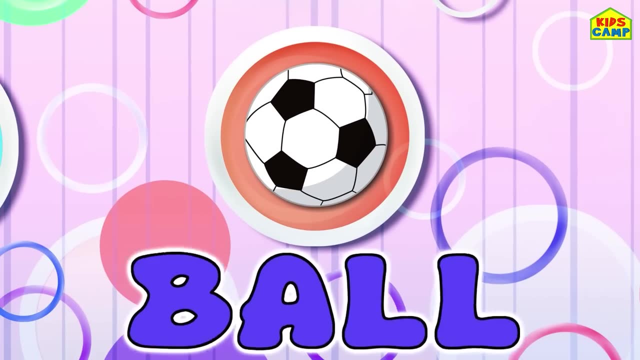 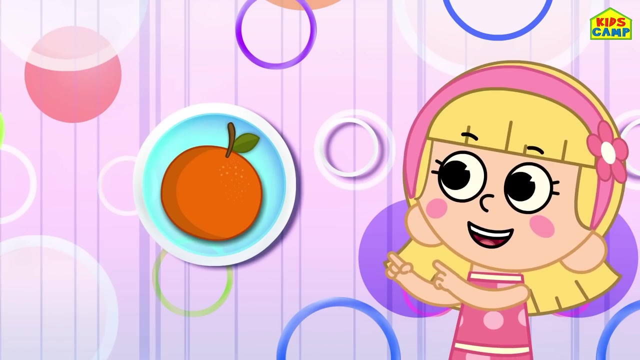 It has three sides. We love triangles. What kind of shape is this? What kind of shape is this? Circle, Circle, The ball is a circle, Like a clock, Like an orange. This is a circle. Shapes are wonderful. What kind of shape is this? What kind of shape is this? 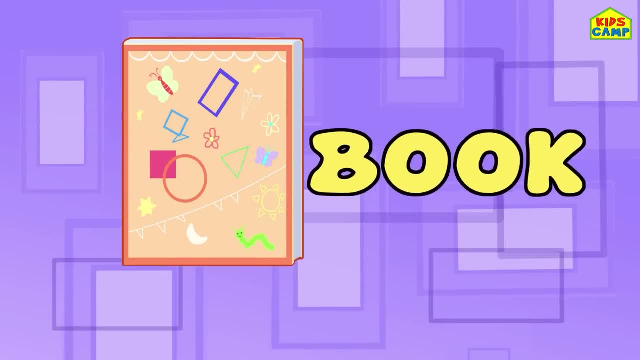 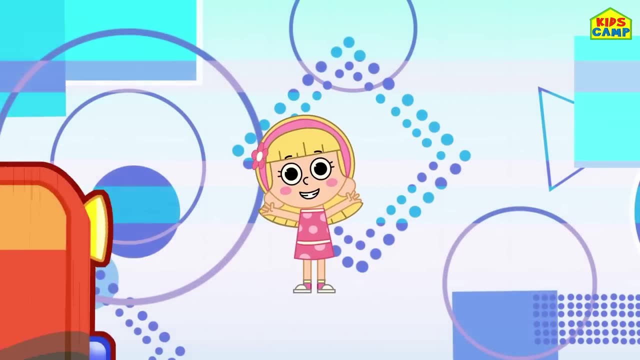 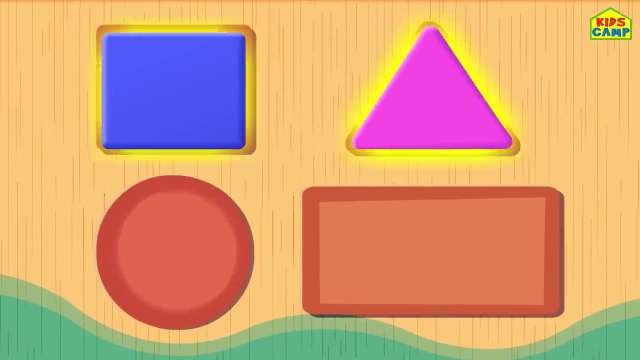 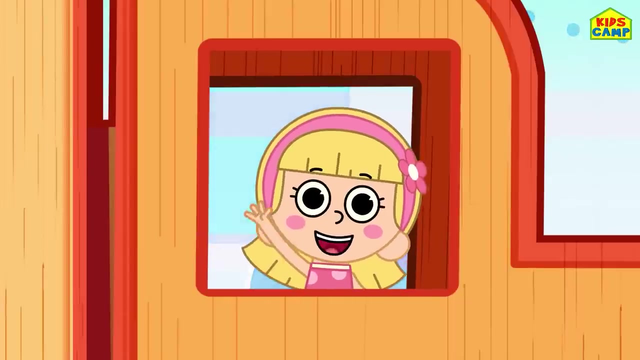 Rectangle, Rectangle. This book is rectangle, Like a blackboard, Like a door. Shapes are easy. Sing along with me. Wow, We learned shapes. Square, Triangle, Circle, Rectangle. Wow, We did it. Bye-bye. 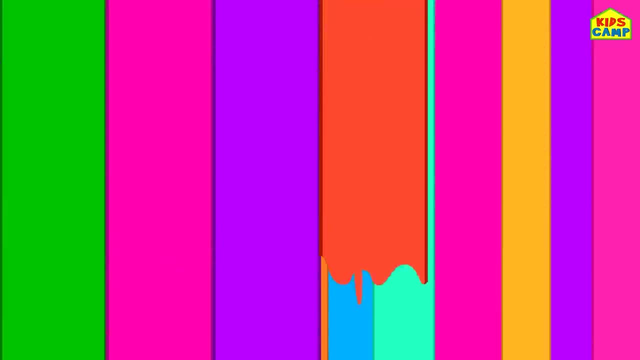 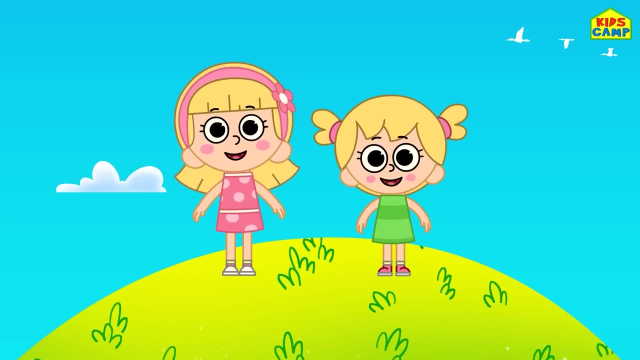 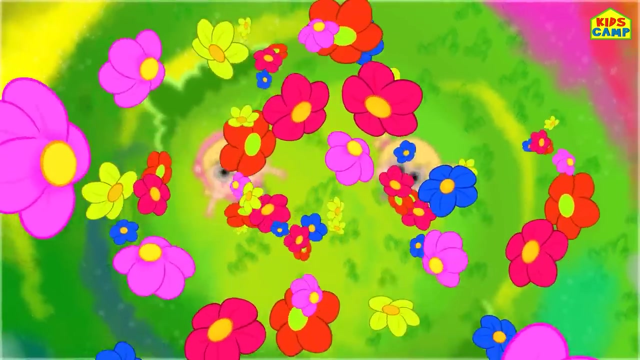 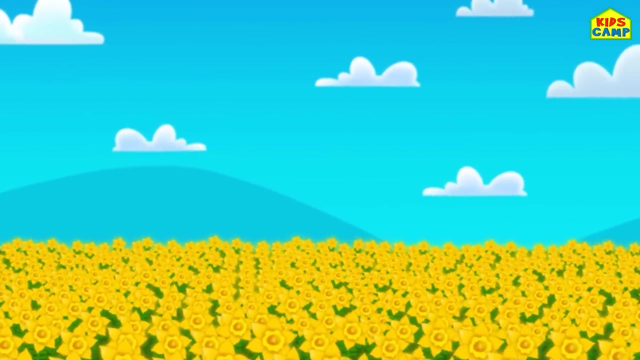 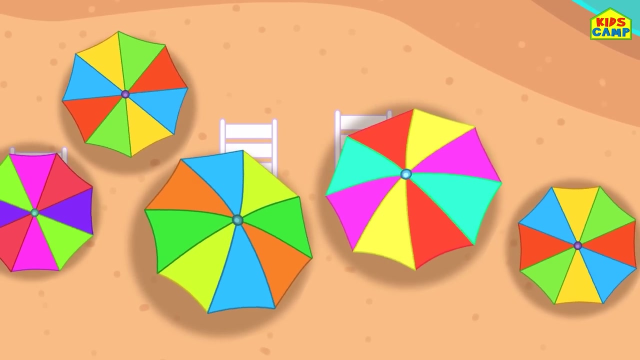 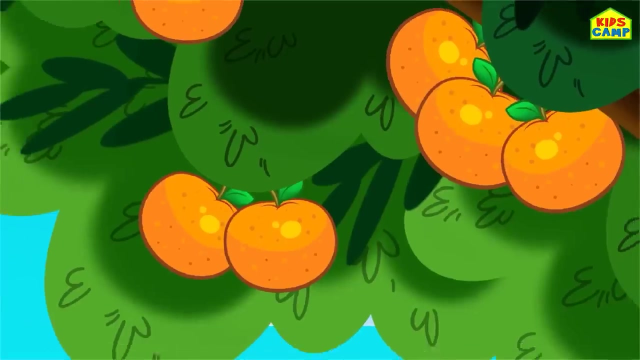 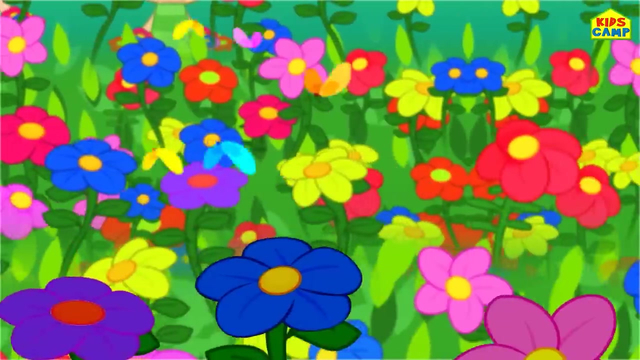 All around the world. you will see. Colors are everywhere for you and me. Yellow are the daffodils and blue is the sea. Colors are so wonderful for you and me: Orange are the oranges and green are the leaves. Colors are so beautiful for you and me. 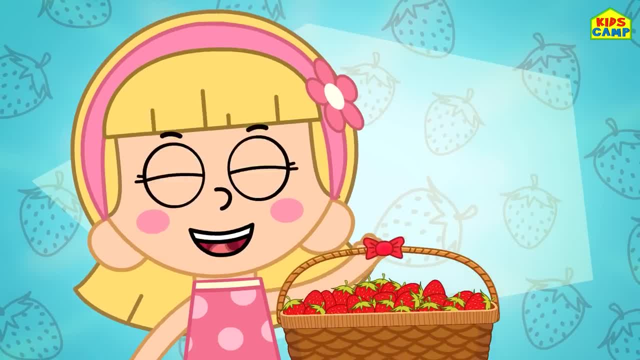 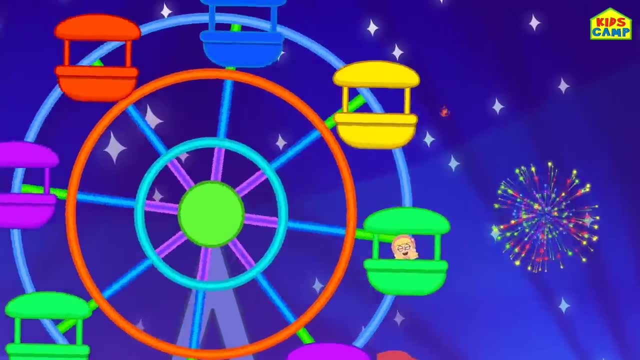 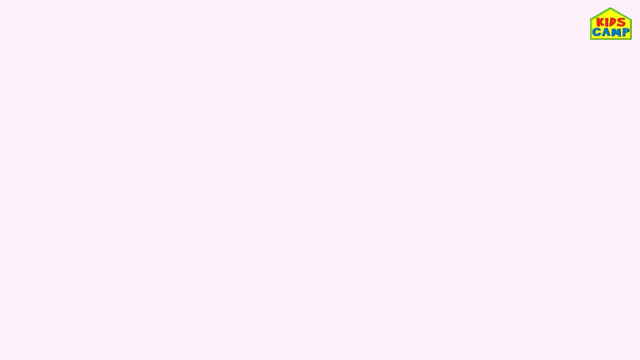 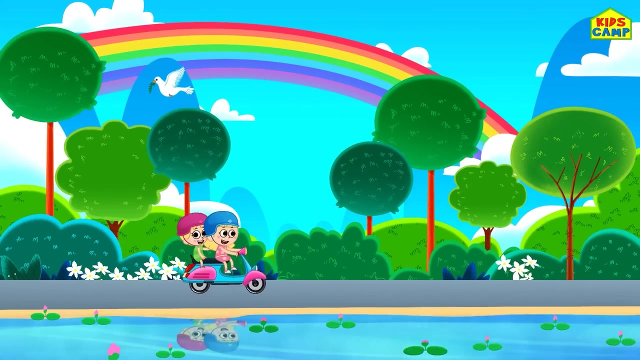 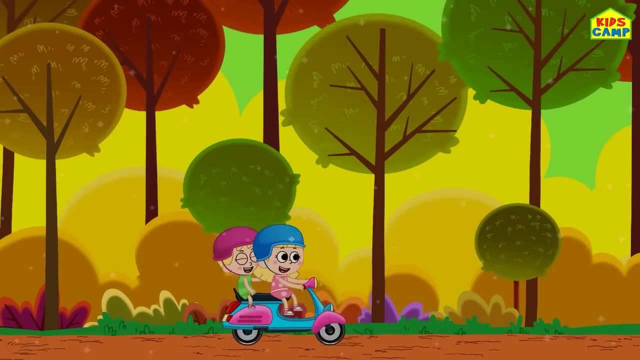 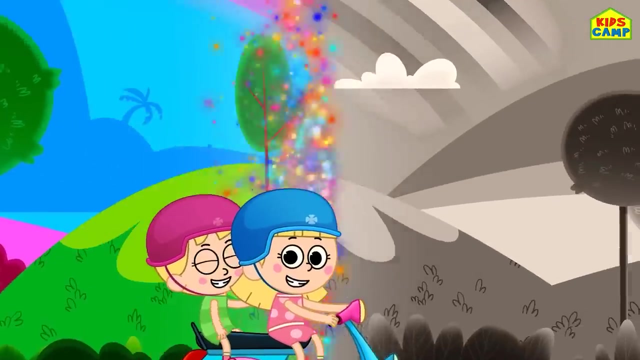 Purple are the orchids and red are the strawberries. Wow, Colors are so magical for you and me. Pink are the hearts, White stands for peace. Colors are so powerful for you and me. Black is the night and brown are the trees. Colors are everywhere, can you see? 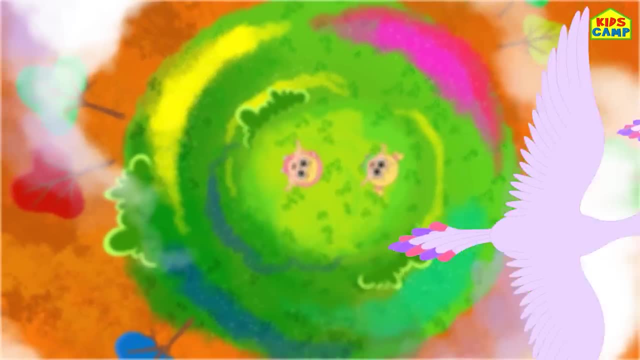 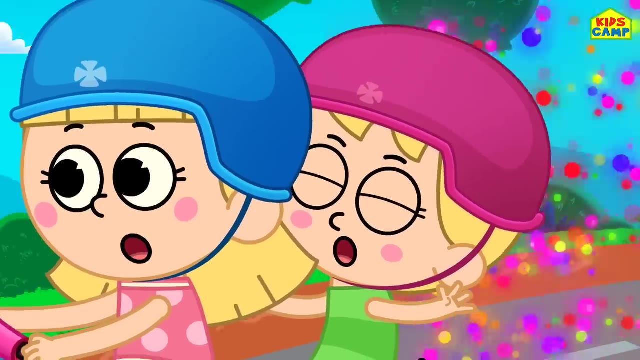 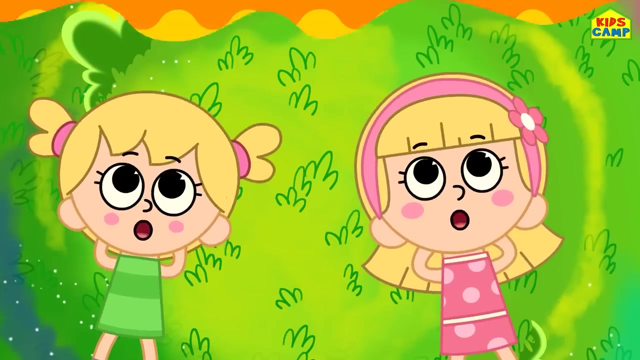 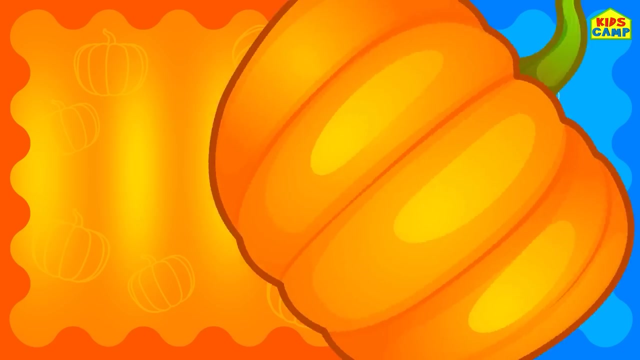 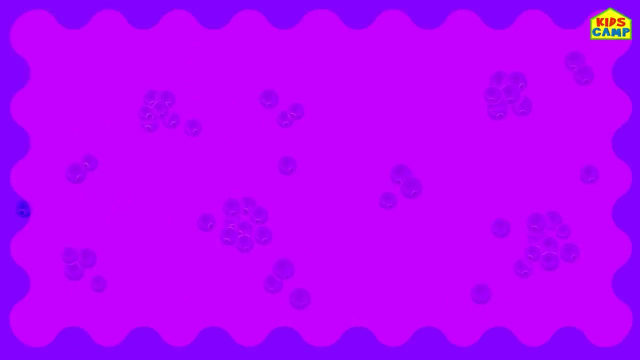 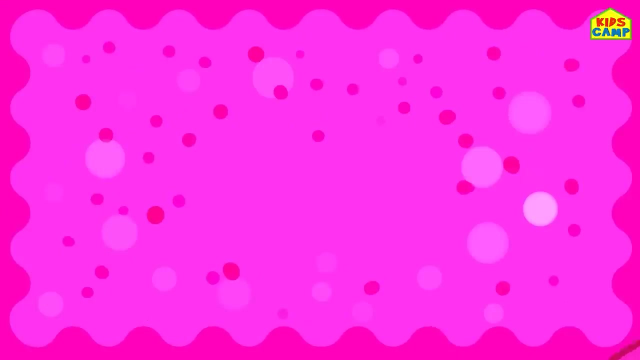 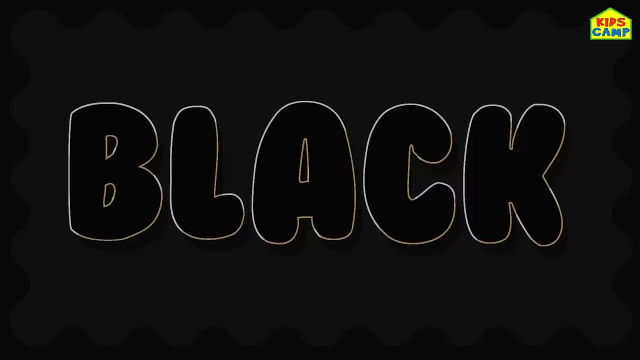 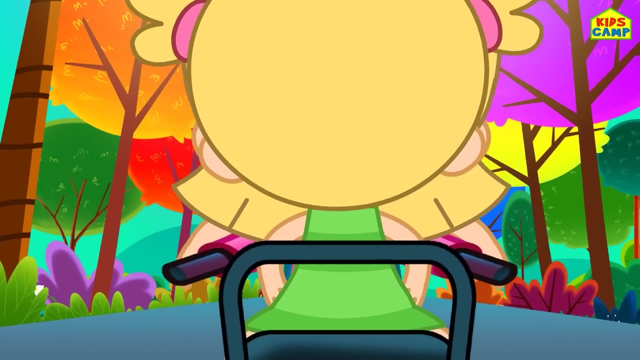 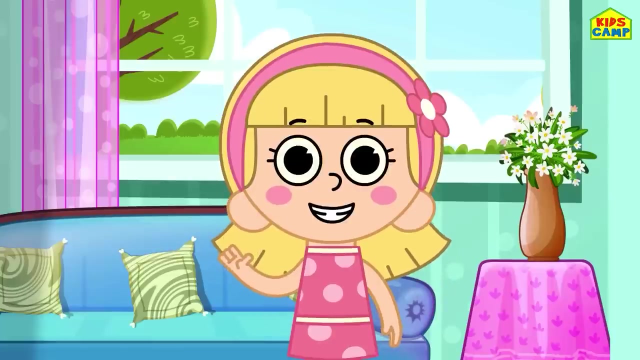 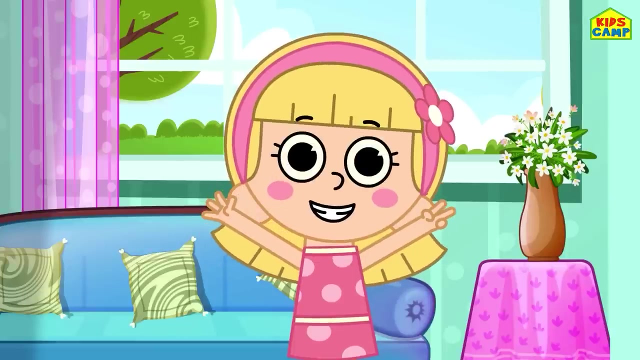 All around the world come paint with me. These colors are so beautiful for you and me: Yellow, Blue, Orange, Green, Purple, Red, Pink, White, Black And Brown, Blue, Blue, Blue, Green, Orange, Blue. 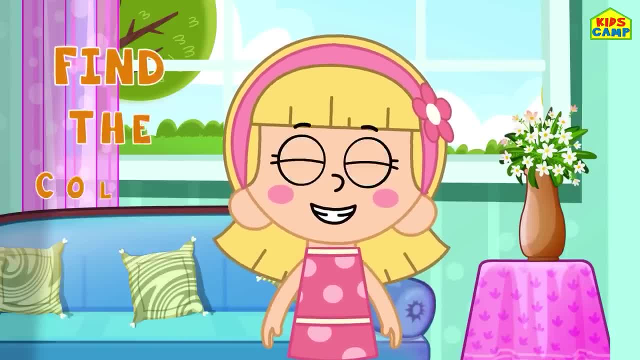 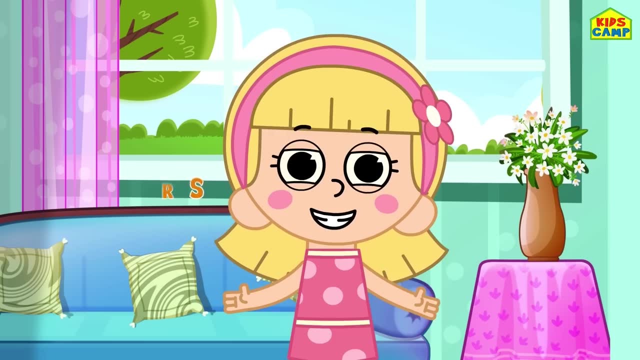 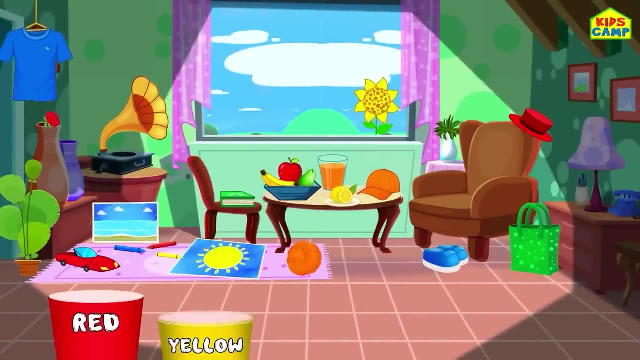 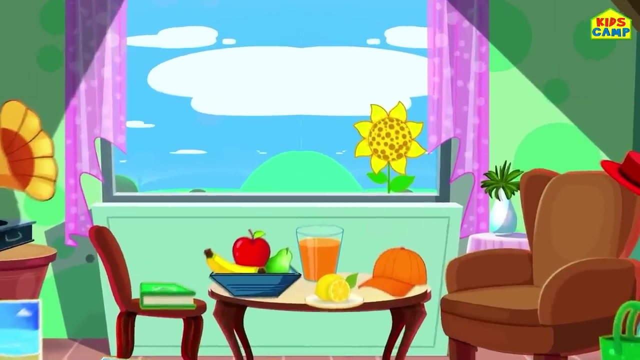 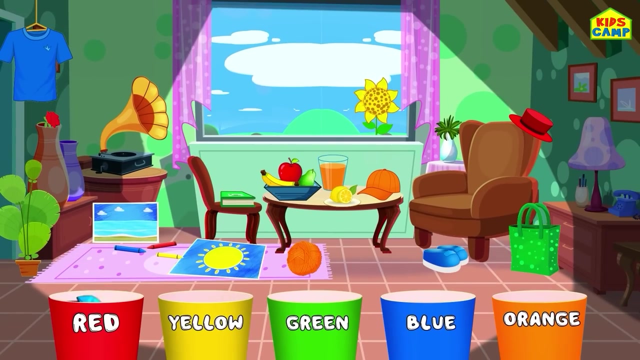 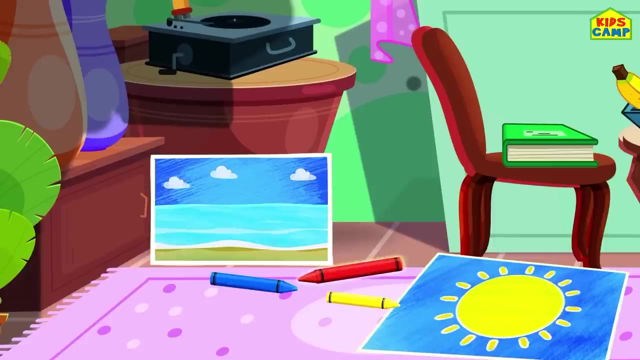 Blue, Blue, Red, Pink, Green, Orange, Blue, Green, Blue. can you spot everything red? let's get started. can you find anything red? um, that's right, a toy car. yes, it's red. let's add it to the red bucket. what next? what else is red? uh-huh, i see a red crayon. 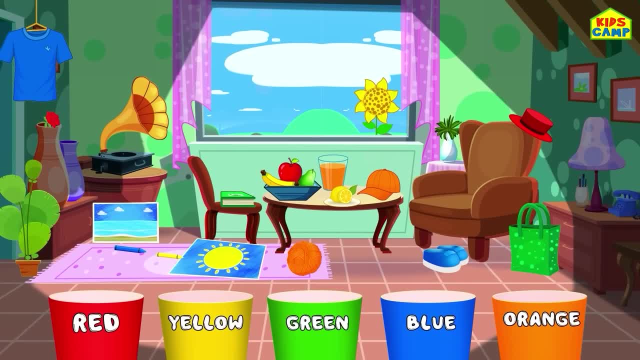 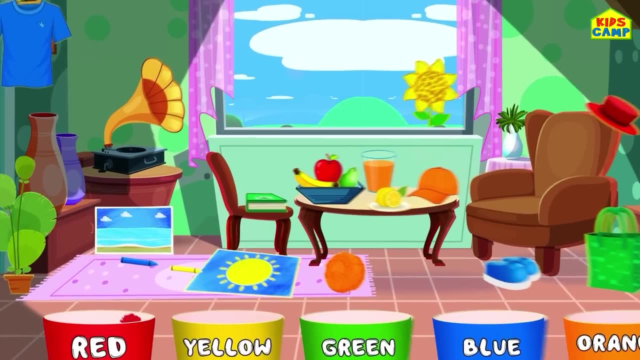 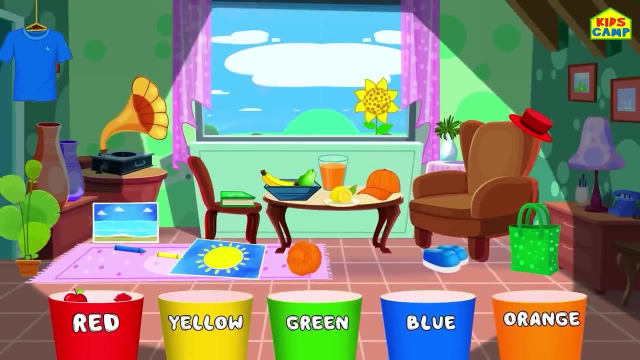 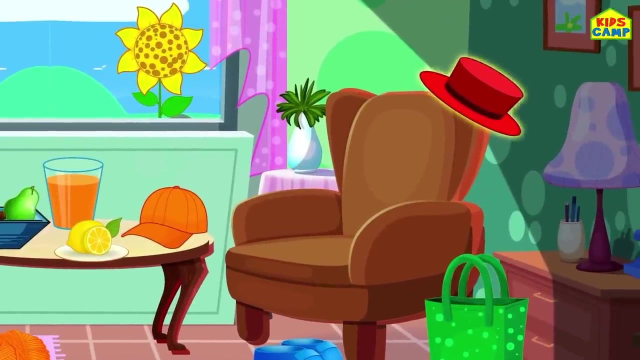 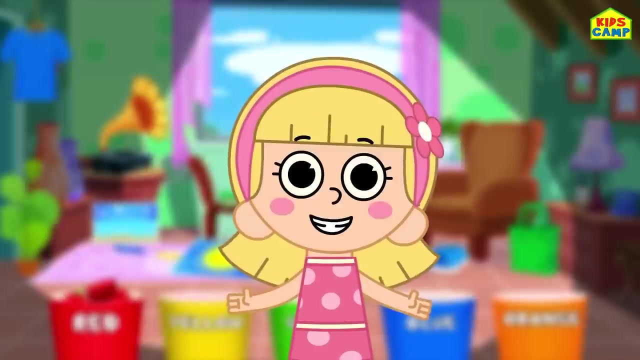 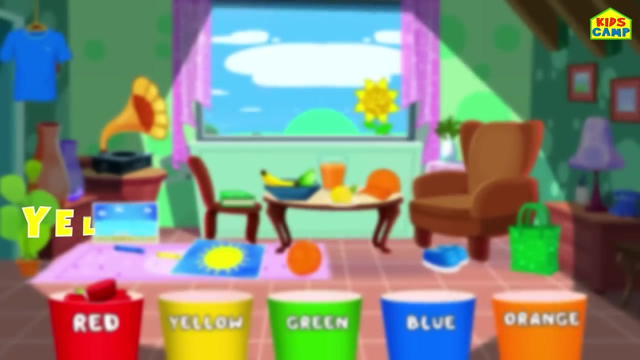 that's right. wow, a red rose. what else is red? an apple. we'll add that to our red bucket. keep looking for something else that's red. that's right. a red hat. we found everything that was red. what's the next color? yellow, my favorite. what do you see that's yellow? 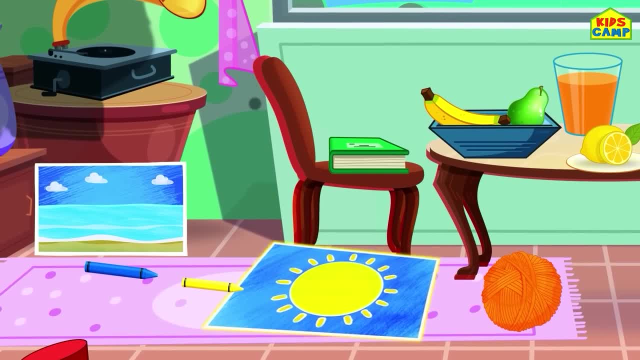 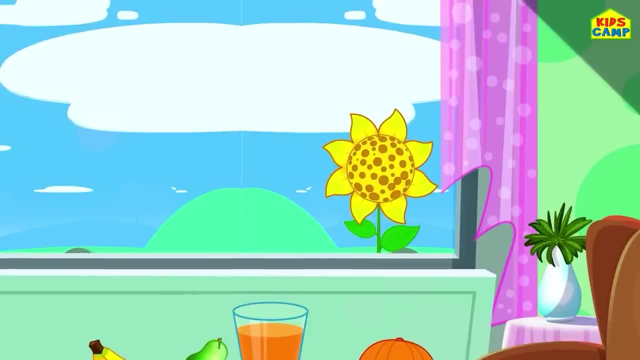 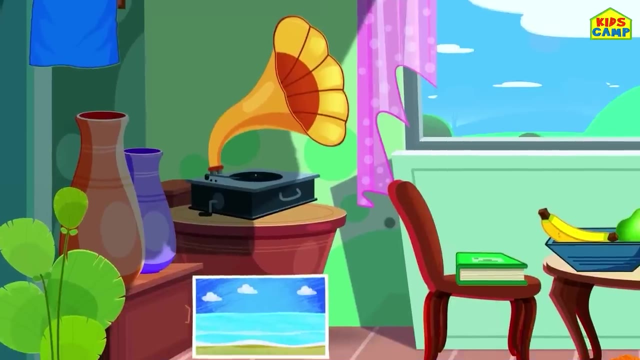 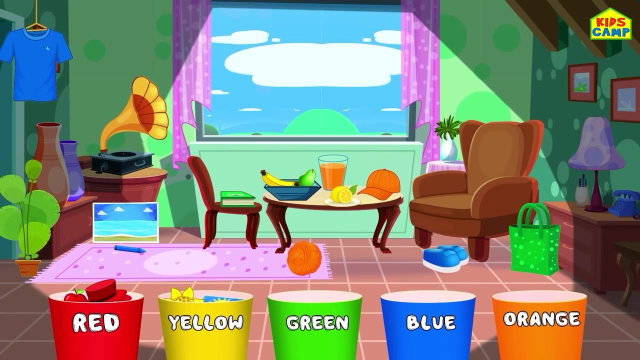 uh-huh, my drawing of the sun, the sunflower, that's yellow too- into the bucket. good job, friends. what else is yellow? a yellow crayon, that's right. what else do you see? uh-huh, lemons, wonderful. what else? uh-huh, a banana, the banana. 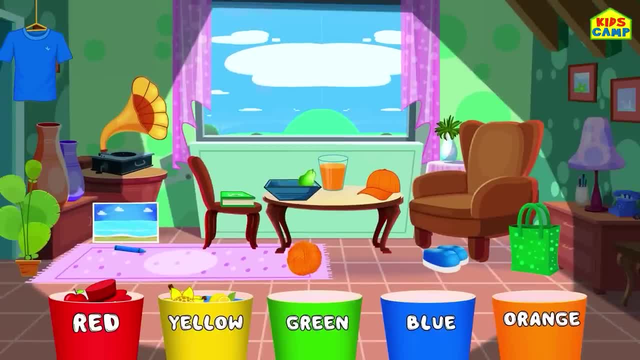 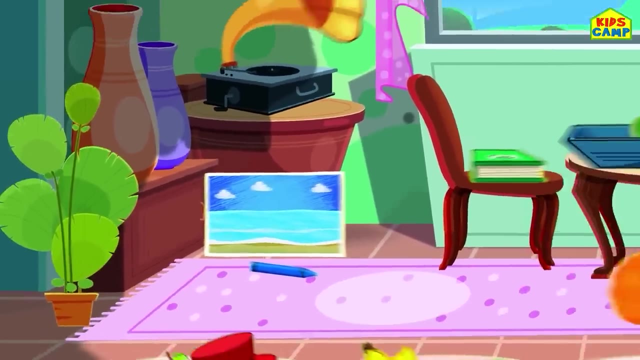 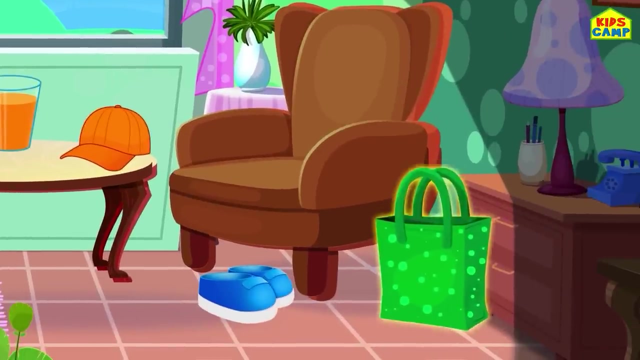 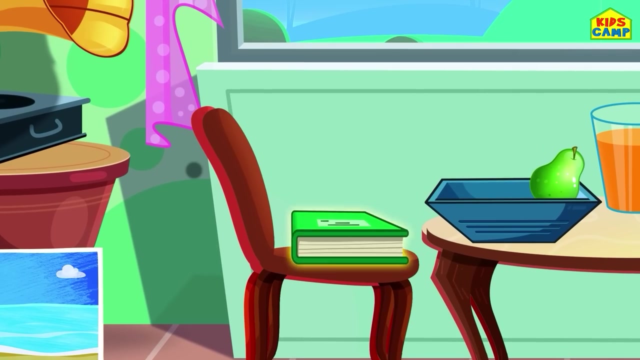 is yellow: into the yellow bucket, it goes. let's go to the next color, which is green. yay, can you look for something that is green in my room? uh-huh, i see it. the plant into the bucket, it goes. what else is green? that's right, the green bag. anything else? i see it too. the green book. 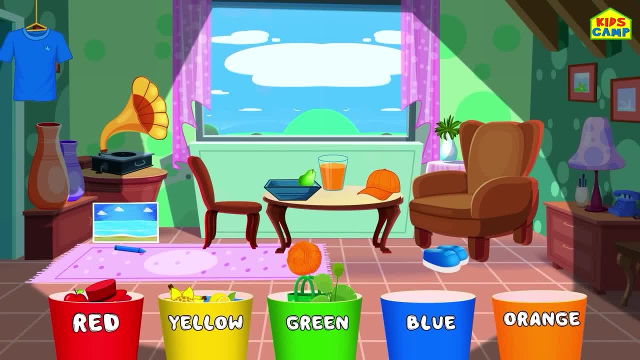 what else? the pear that's green too, Into the green bucket. Yay, Let's move on to the next color. It's blue. Woohoo. What's blue colored here? The blue crayon. Anything else? My drawing of the blue sky. 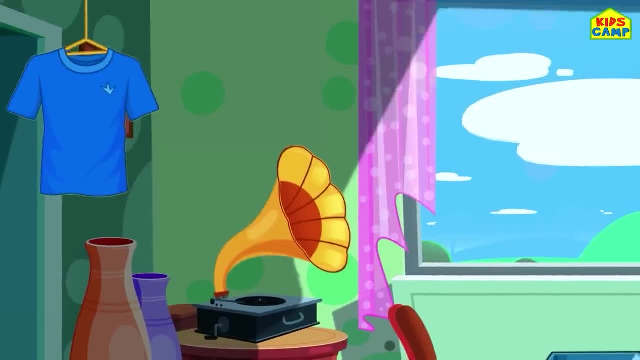 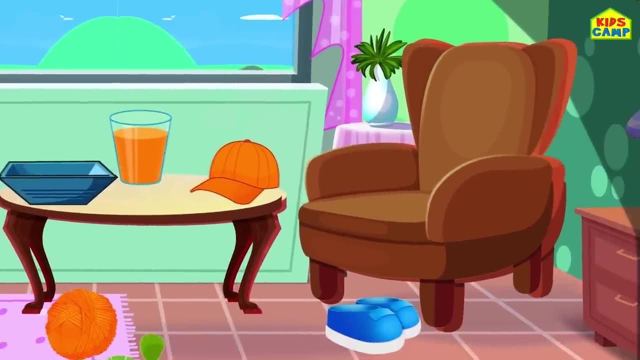 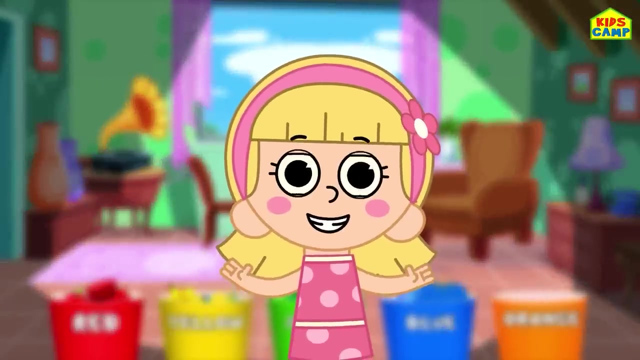 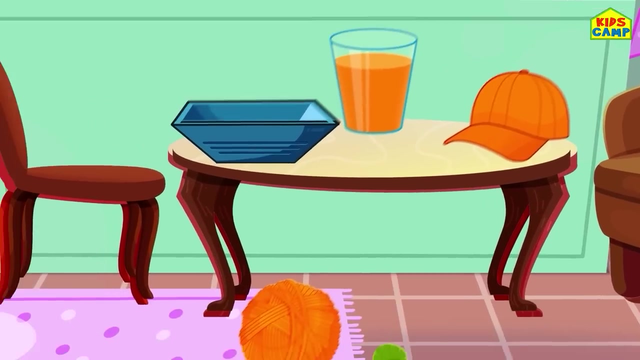 What else? The blue t-shirt Into the bucket? Uh-huh, I see My pair of blue shoes. We found everything blue. What's next? It's orange. That's right. Can you spot something orange? An orange yarn of wool. 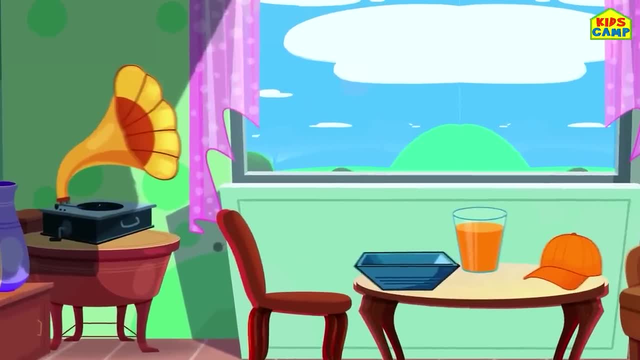 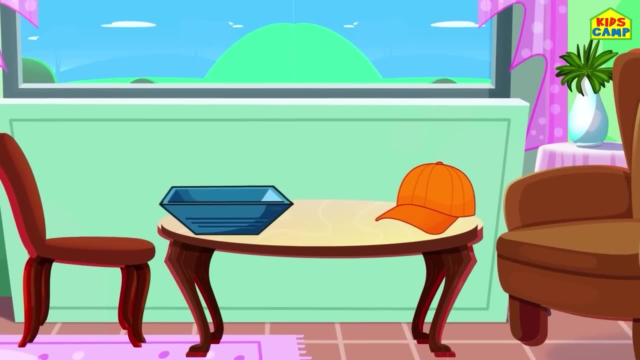 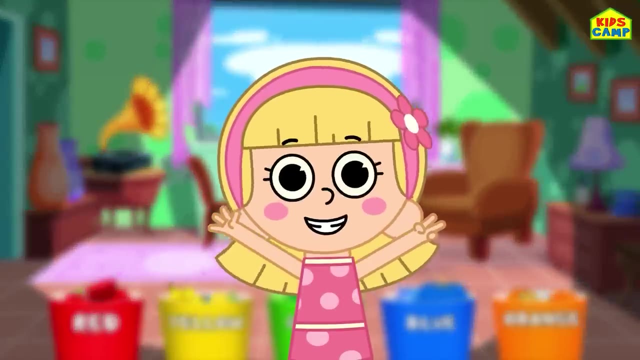 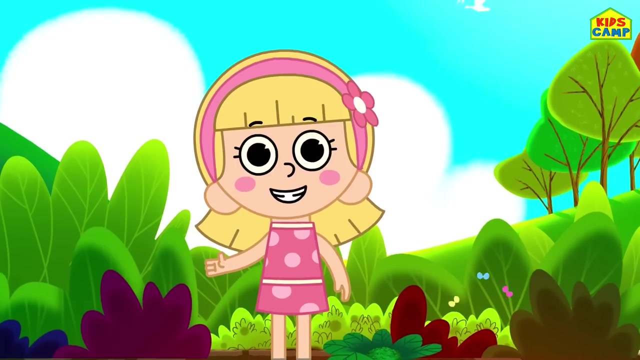 That's right. What next? I see it: A glass of orange, Orange juice And an orange cap. Yay Into the orange bucket. it goes. Wonderful kids, We found all the colors. Bye, Let's have fun learning. 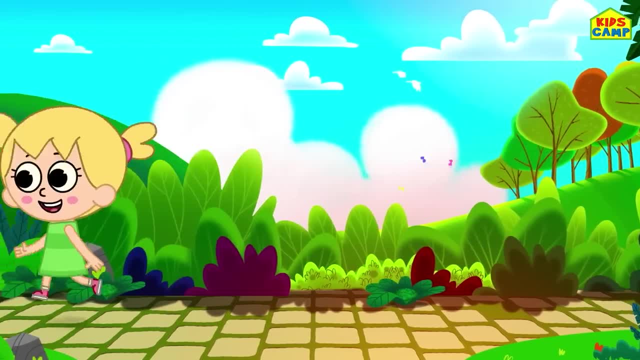 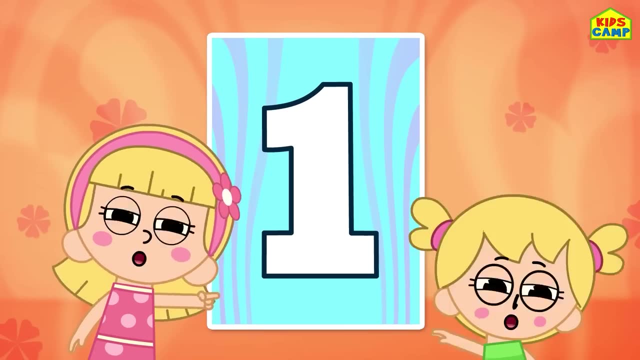 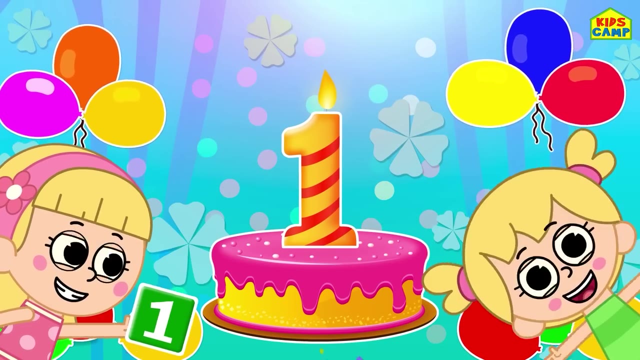 Yay, I'm so excited. Let's draw number one. Let's draw number one. One, One, One, One is so much fun, Like a candle To celebrate Number one. Yes, It's so much fun. Let's draw number two. 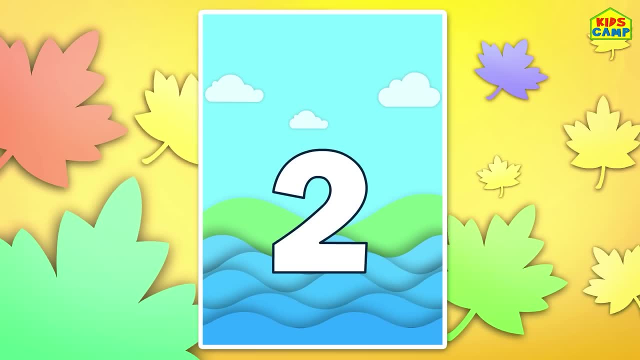 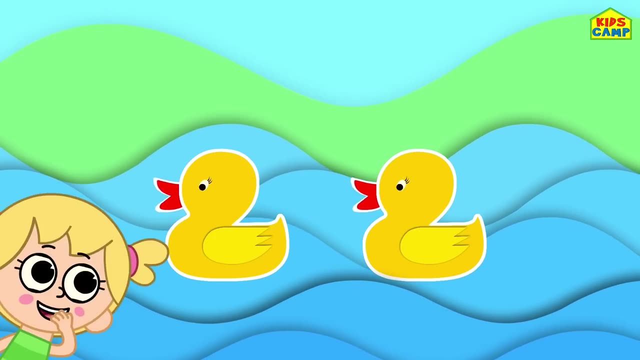 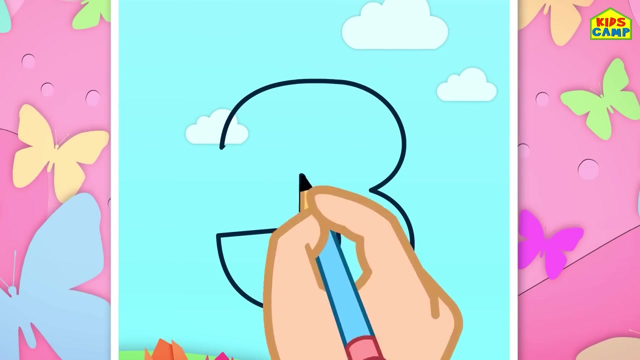 Let's draw number two. Two, Two. Let's draw number two. Two lovely ducks. They go quack, quack. Such cute ducks. There are two cute ducks. Let's draw number three. Lovely ducks. Lovely number three. Three. 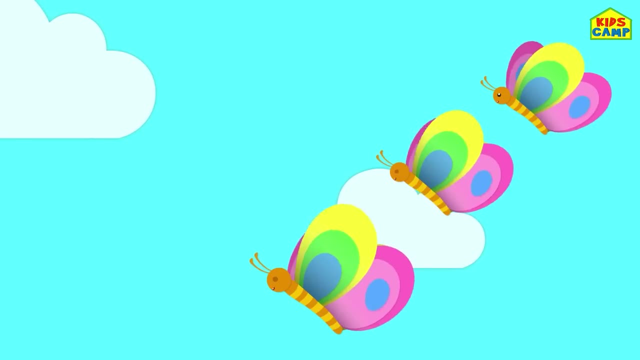 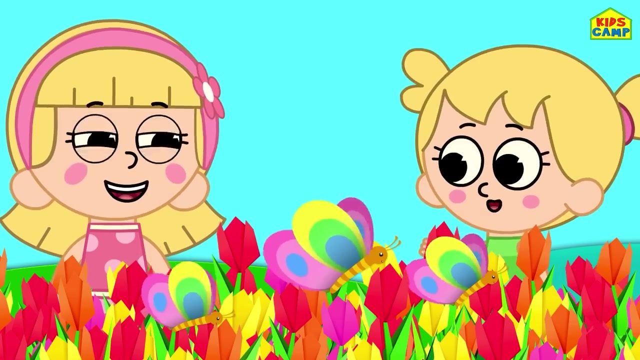 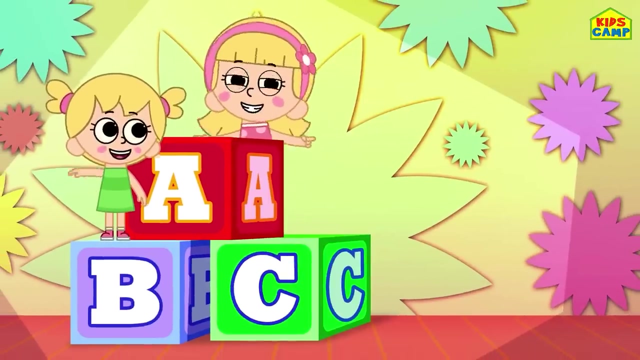 Three, Three butterflies you'll see, In the sky, On the flower: Three, Three, Three butterflies you'll see. Let's learn A B C. Let's learn A B C To learn, To learn, To learn with A B C. 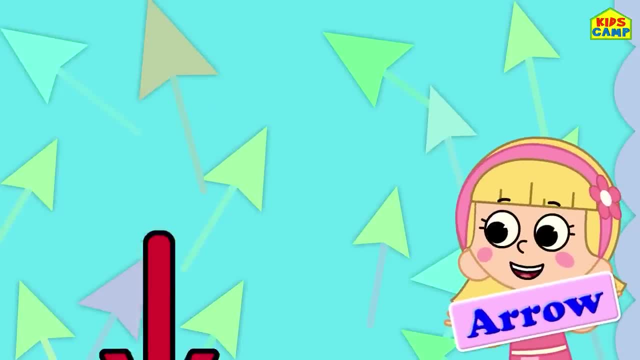 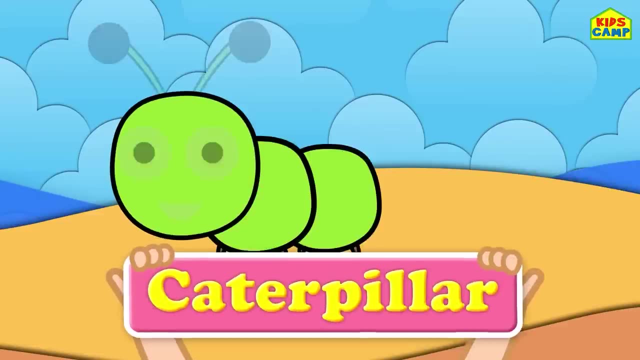 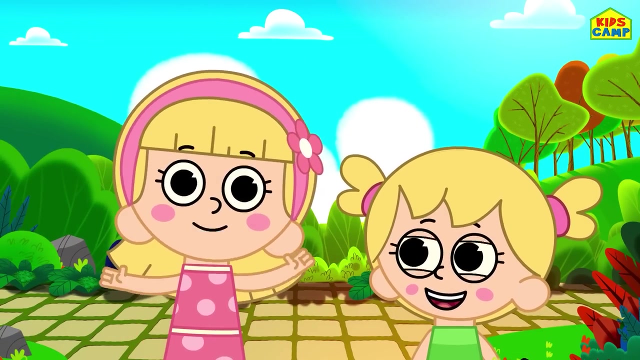 Letter A Like an arrow, Letter B Like a bird Letter C A caterpillar. This was so much fun. This was so much fun. Yes, We learned 1,2,3 and A, B, C's. Yes, We learned 1,2,3 and A, B C's. 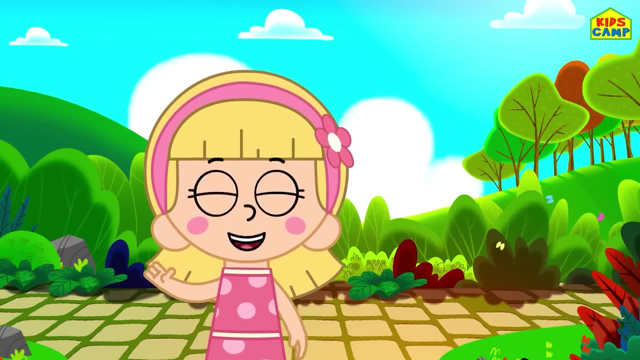 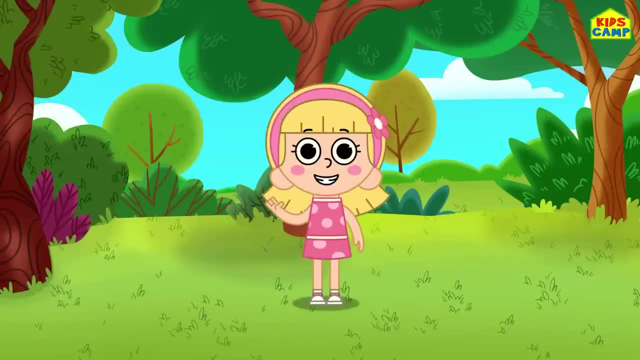 Yay, Yippee, Hope you liked it too. Bye Bye, Hope you liked it too. Bye, Bye. Hi, I'm Ellie, And we are going to play a fun game. We have to spot the differences, And this is going to be such a fun game. 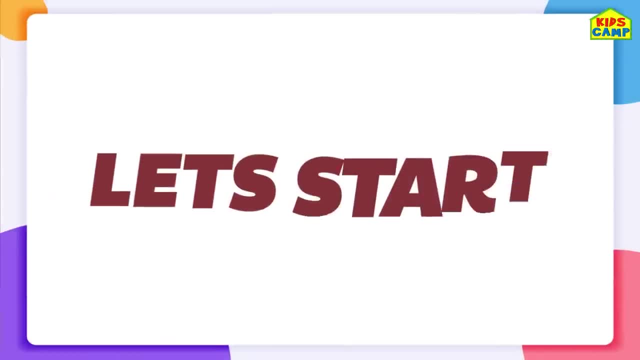 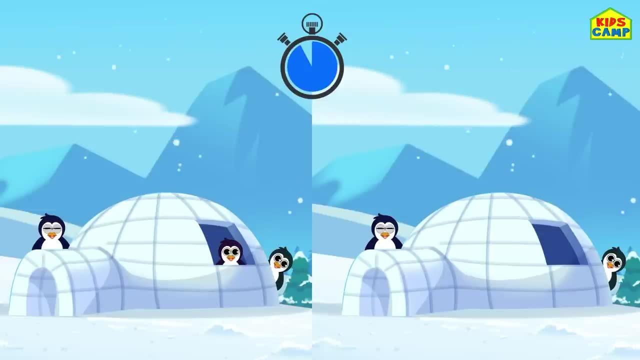 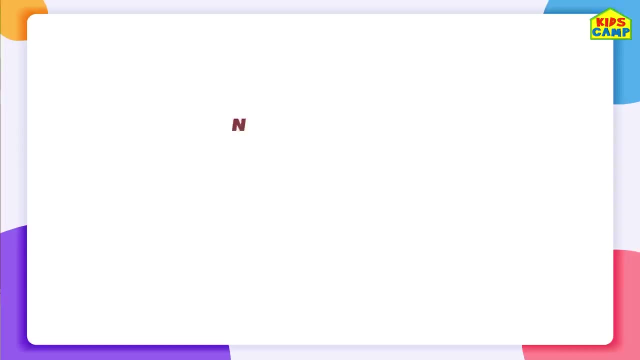 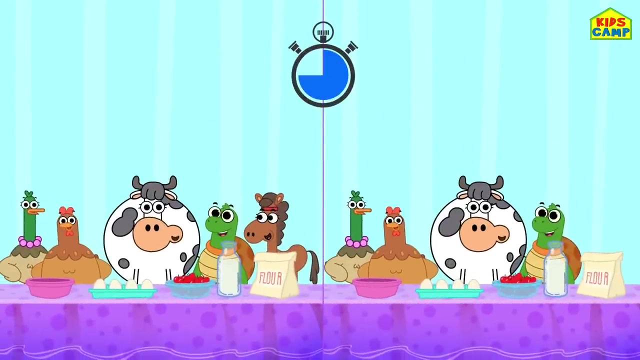 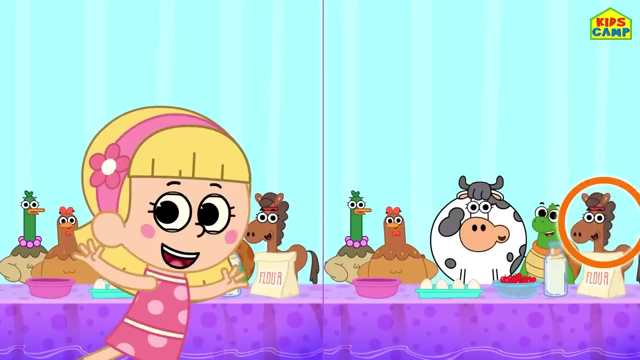 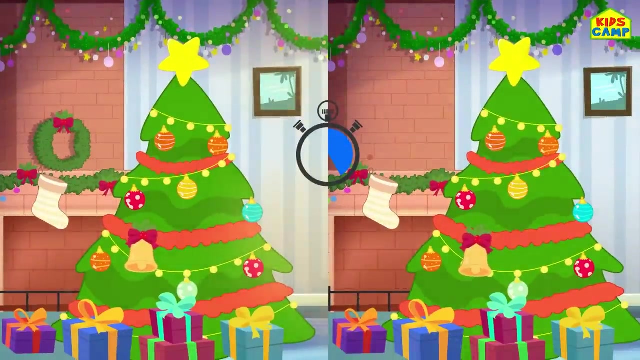 Ready, Let's start. Can you spot the difference? Time's up? That's right. Next one: Can you spot the difference? Time's up? That's right. Yay, Can you spot the difference? Time's up? Keep looking. 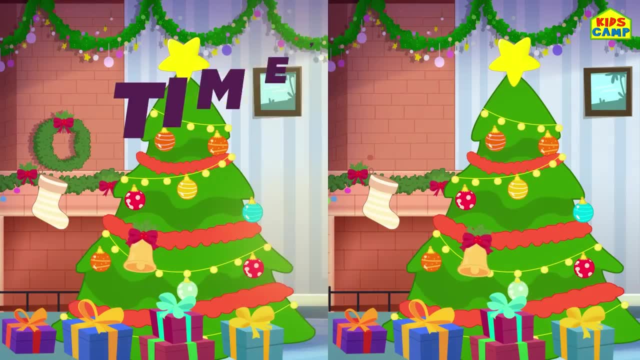 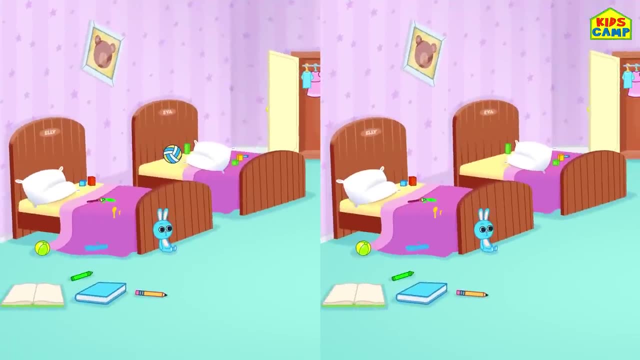 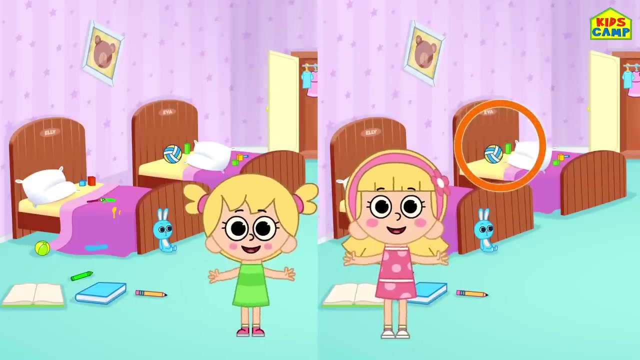 Time's up, Time's up. That's right. Yay. Next one, Next one. Can you spot the difference? Can you spot the difference? Keep trying Wa- circulation. You've been having fun, That's right. Times out. 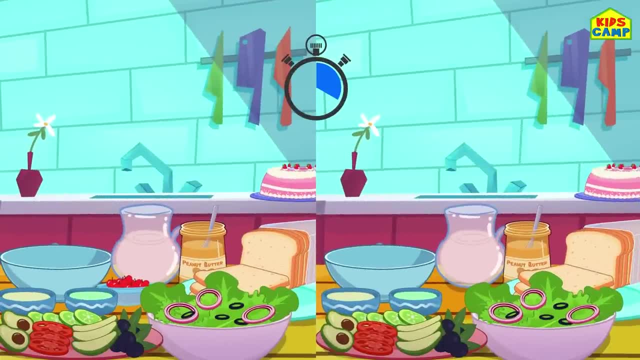 Oh, He made it a second time. Woohoo, Did you guys try? Yippee, Yay, You guys did rock it, Yay. Next one: Can you spot the difference? Next one: Can you spot the difference? 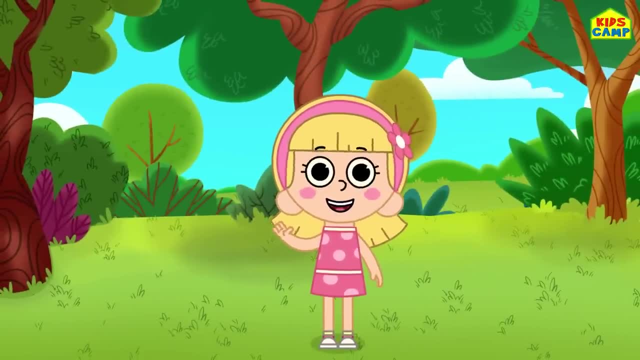 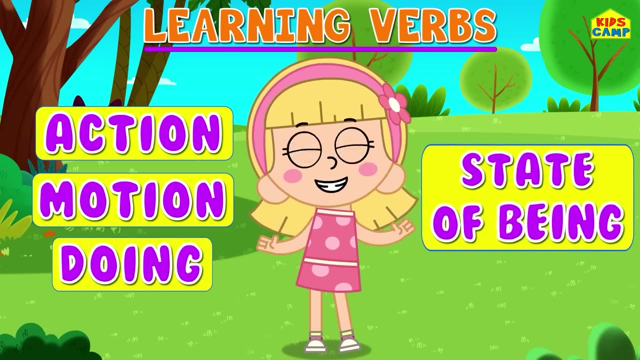 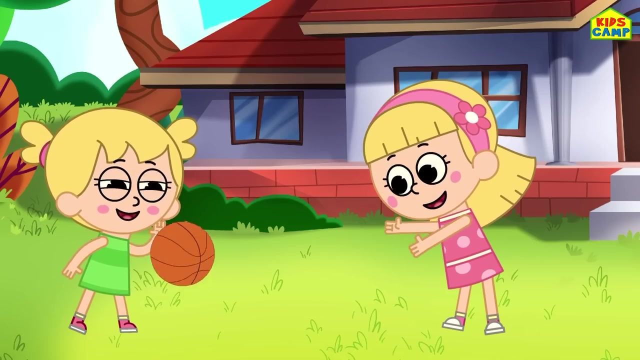 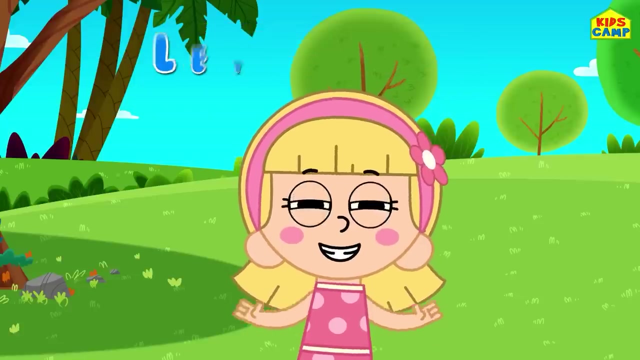 Keep trying. bye, hi. verbs are words that show action, motion, doing or a state of being. and i am on a playground and i'm playing with eva. what we are going to do today is find verbs. are you ready? let's get started right away. we have to look for the verb. 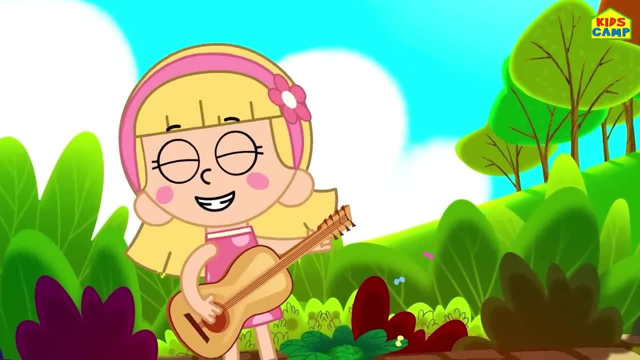 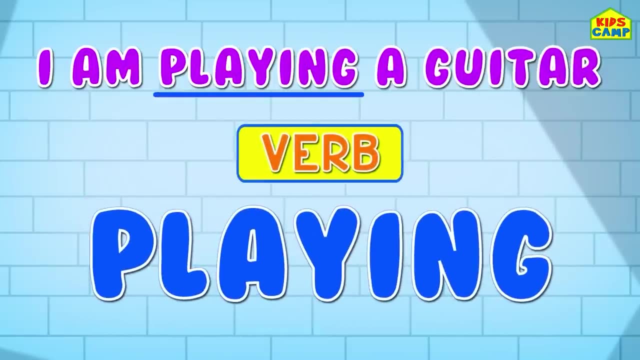 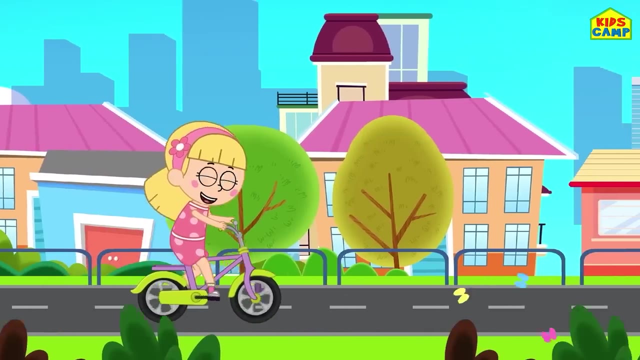 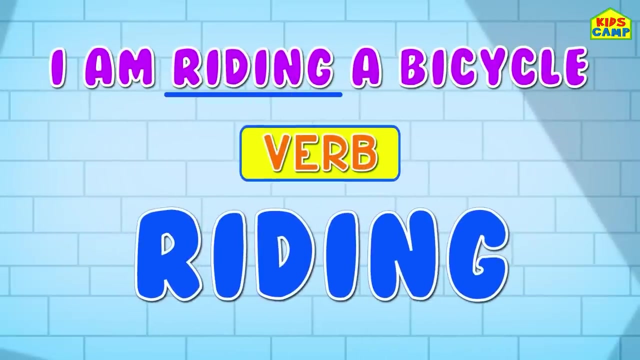 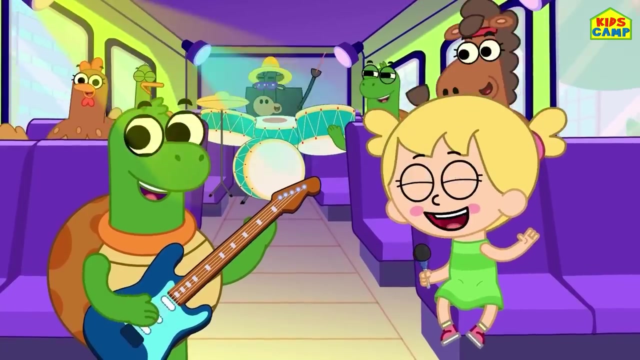 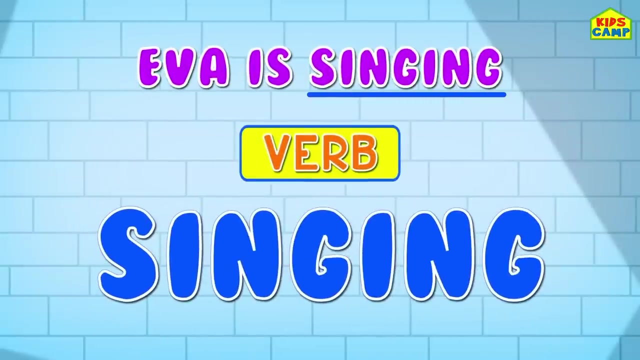 can you find what's the verb in the sentence? i am playing the guitar. playing is the verb here. that's right. what's the activity i'm doing here? i am riding a bicycle, that's right. writing is a verb. look at my little sister, eva. she loves to sing, that's right. eva is singing. singing is the word here. good job, friends. 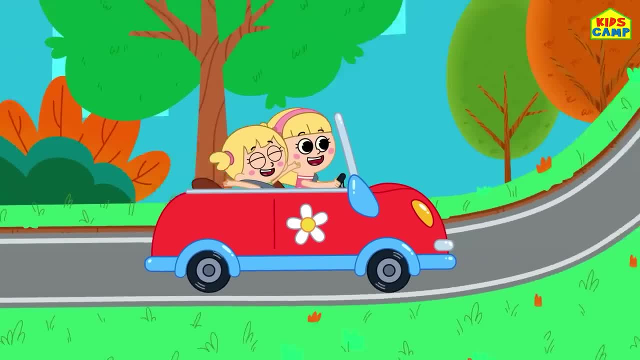 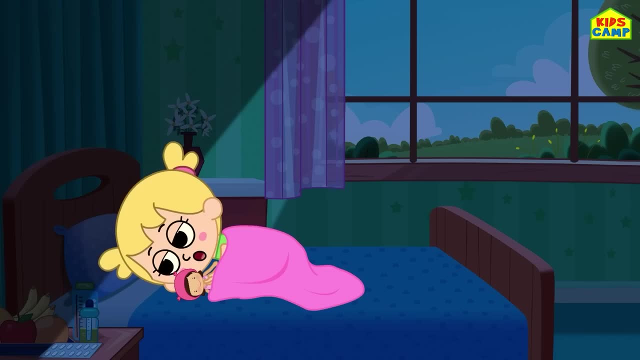 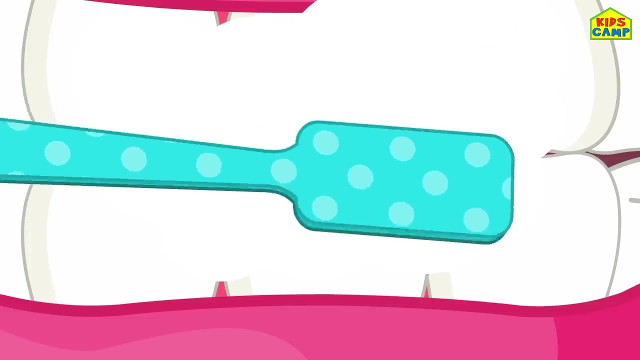 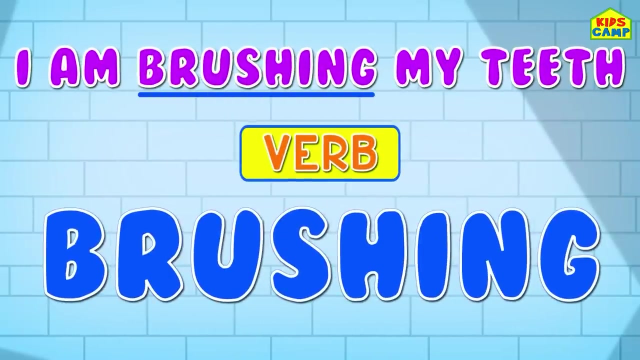 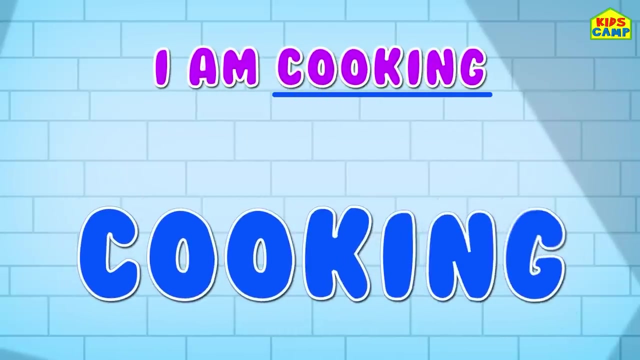 look at me: i am driving- yay, that's right, driving is the verb here. and what is it that we do the first thing when we get up in the morning? that's right. we brush our tea. i am brushing my teeth- brushing is the verb here, eva- and i love to cook. i am cooking. cooking is the world here. 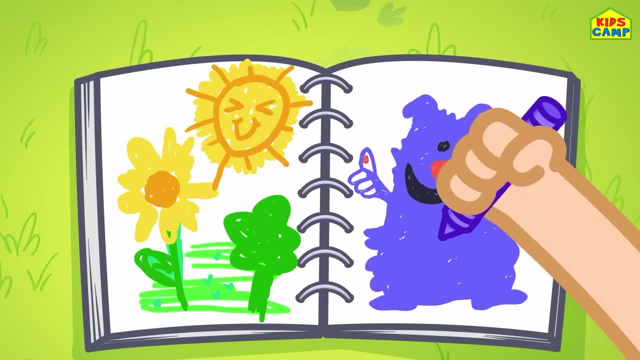 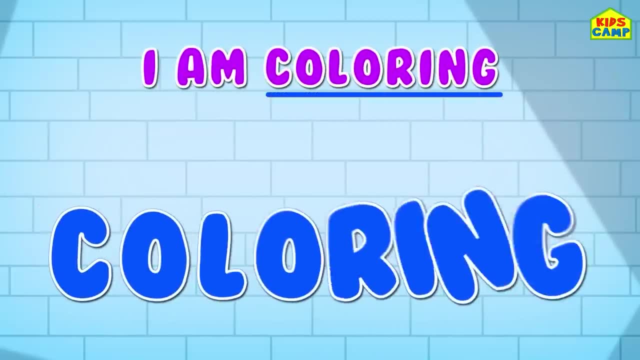 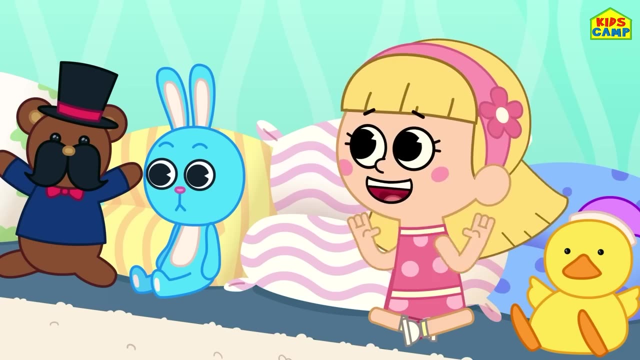 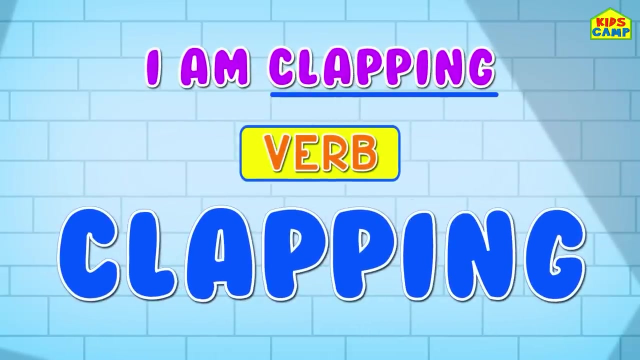 and i've got a new box of crayons. i love to use my crayons to draw and color. i am coloring. coloring is the word here. Woohoo, I am clapping. I am clapping. Clapping is the verb here. Woohoo, We are eating apples. 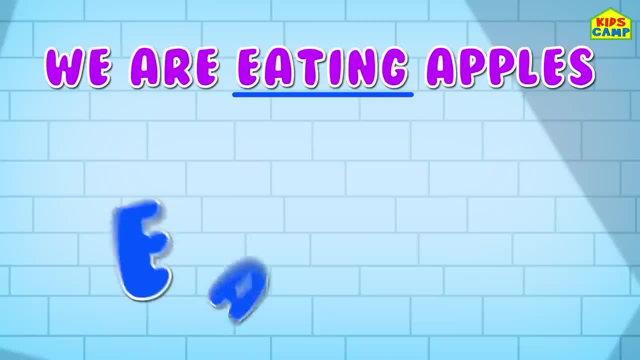 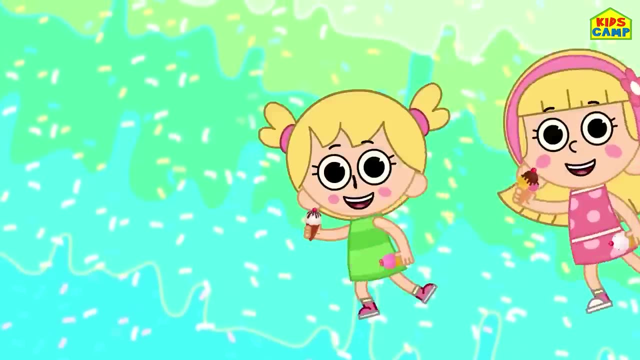 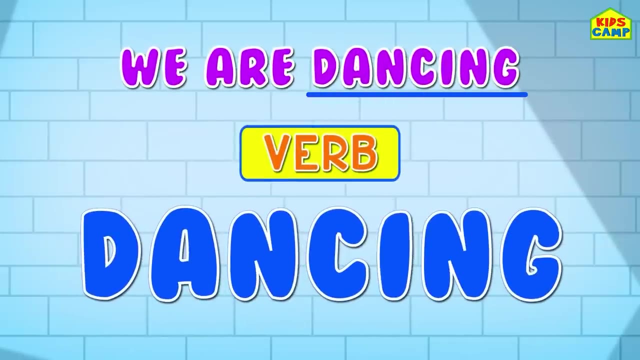 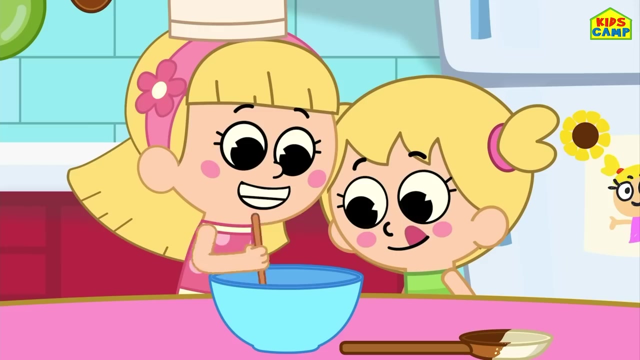 We are eating apples. Eating is the verb here. Woohoo, That's right. We are dancing. We are dancing. Dancing is the verb here. Wow, This was so much fun. What do you like to do? Do you like to cook, play guitar, paint, sing or ride a bike? 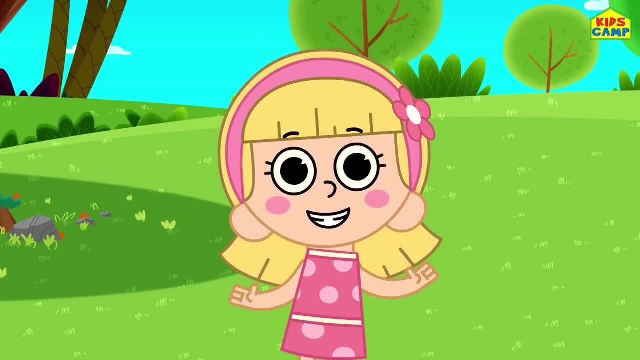 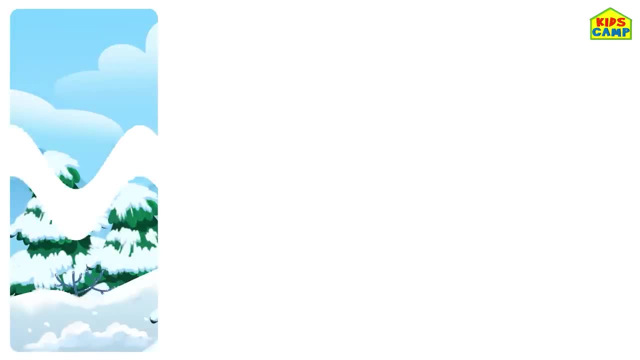 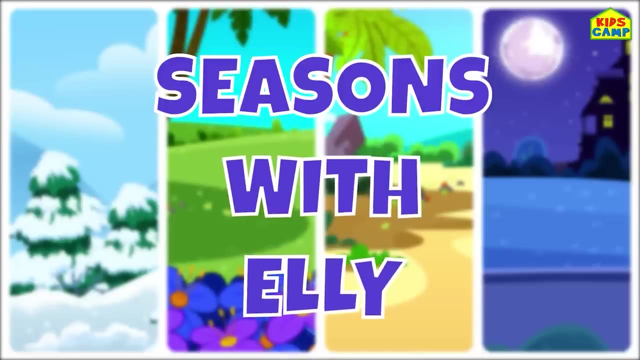 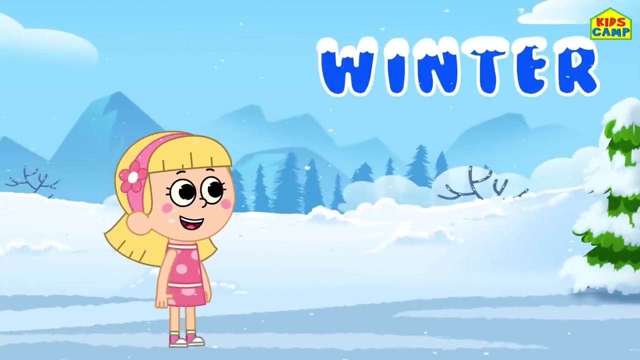 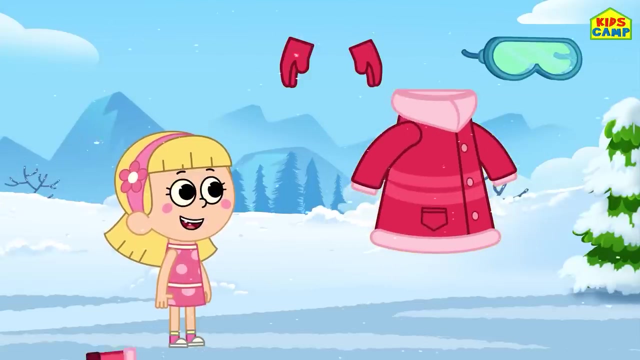 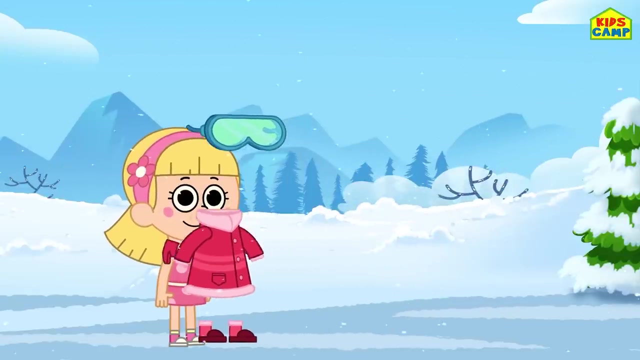 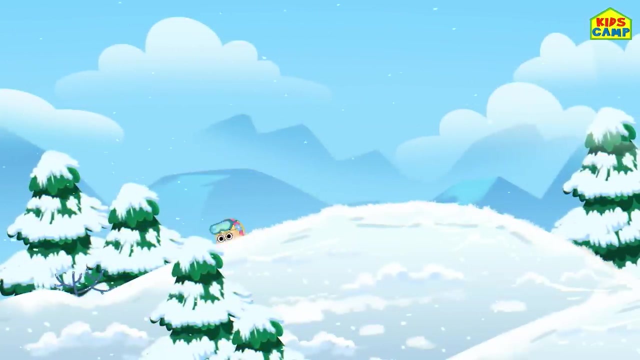 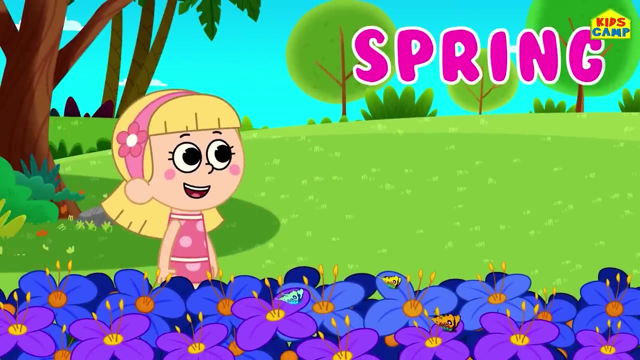 Let me know. Until then, keep watching Kids Camp. Bye-bye Seasons with Ellie. What season is this? Winter Gloves, Snow goggles, Coat, Boots, Yay, Woohoo, What season is this? It's spring. Flower headband, Wow. 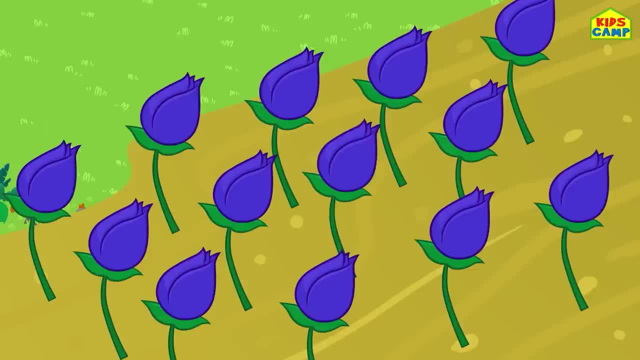 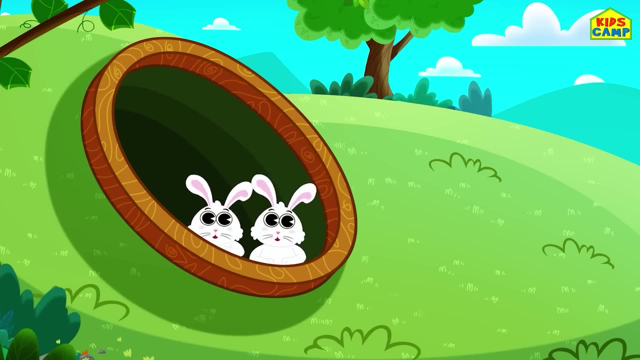 Wow, Look at: the flowers bloom And the birds sing, The bunnies have come out to play and the sun is shining bright. What season is this? It's summer. Swimsuit, Sarong, Sunglasses, Hat, Yay. 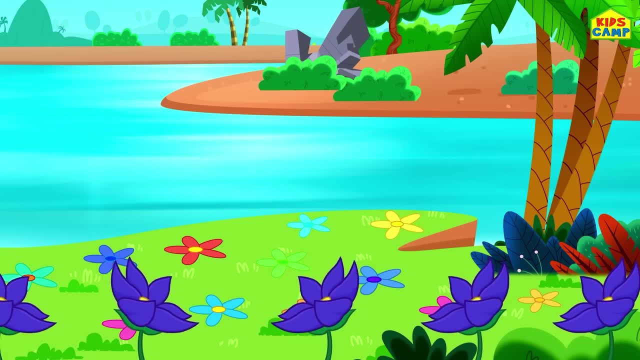 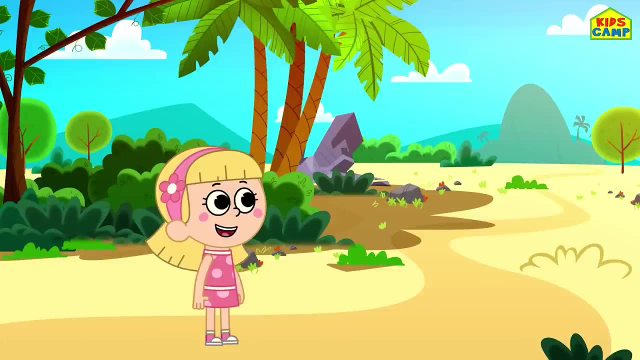 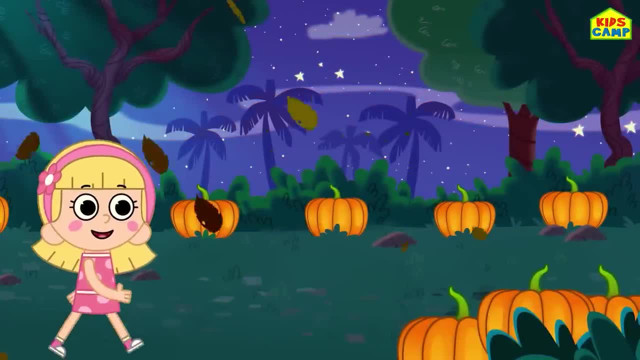 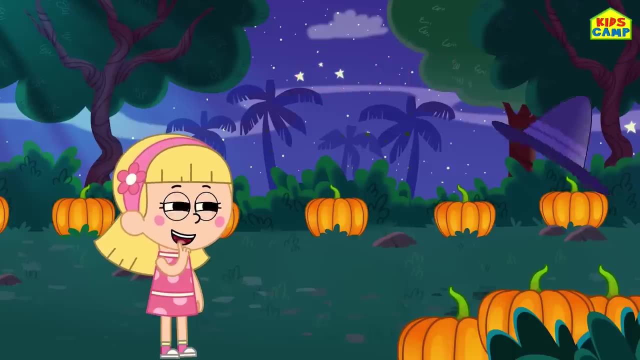 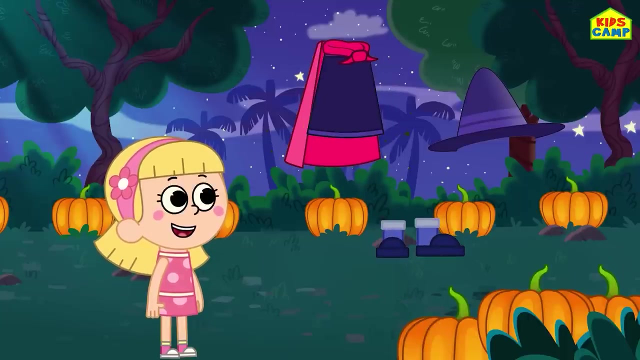 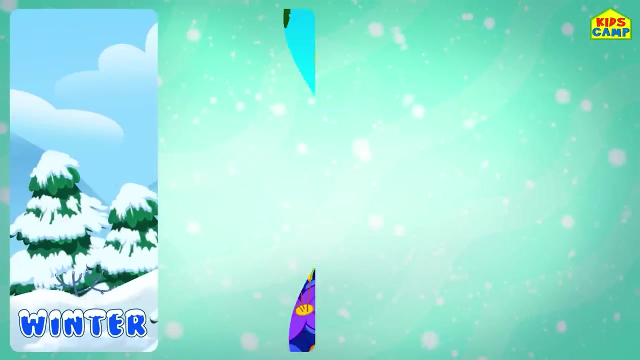 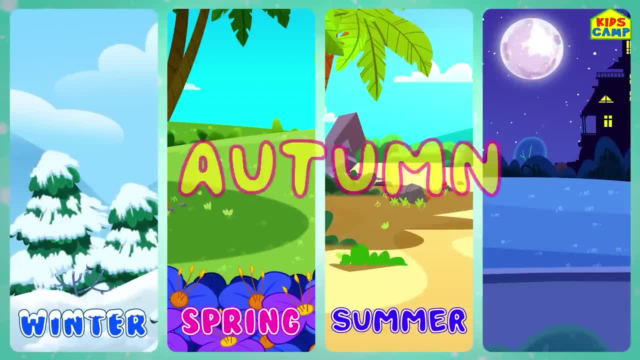 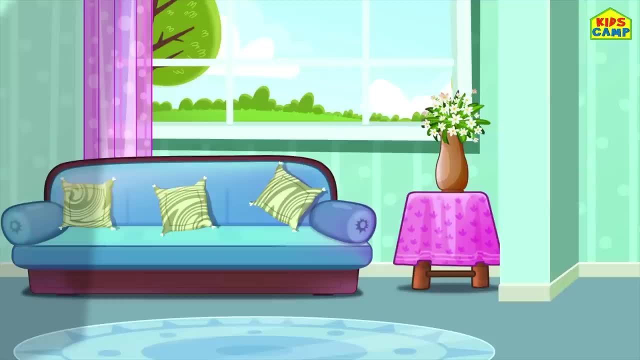 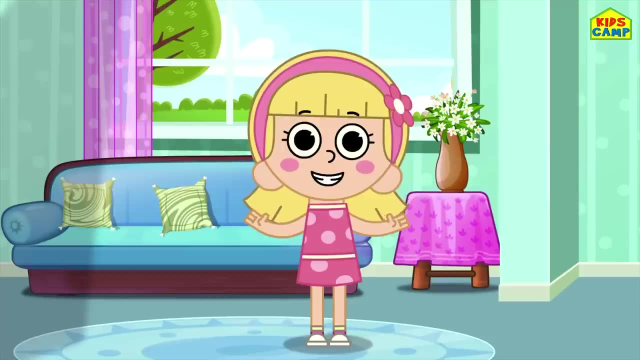 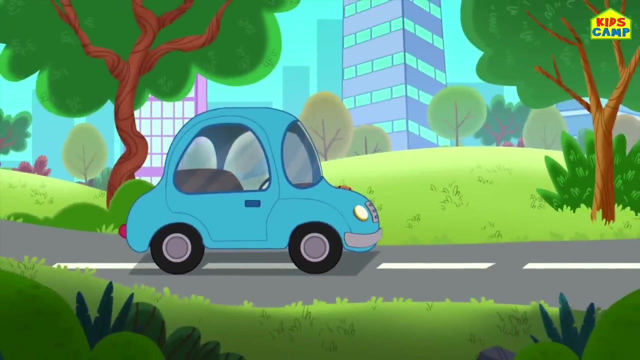 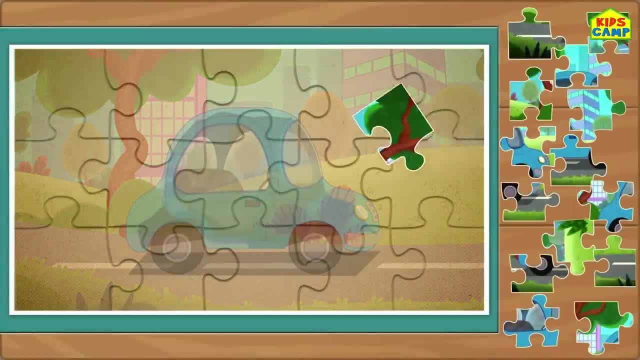 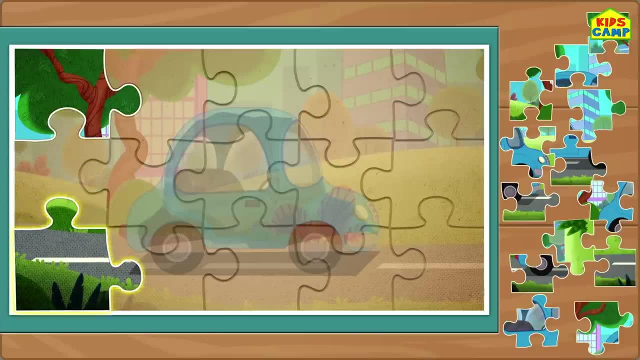 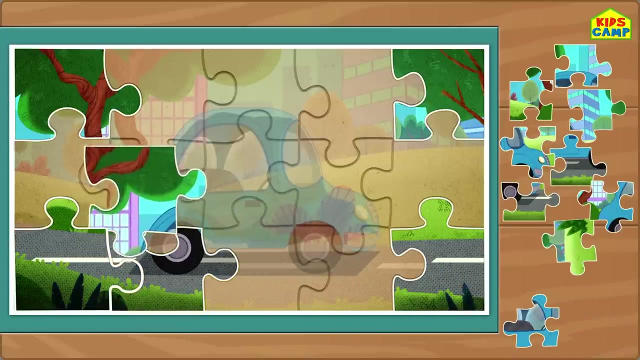 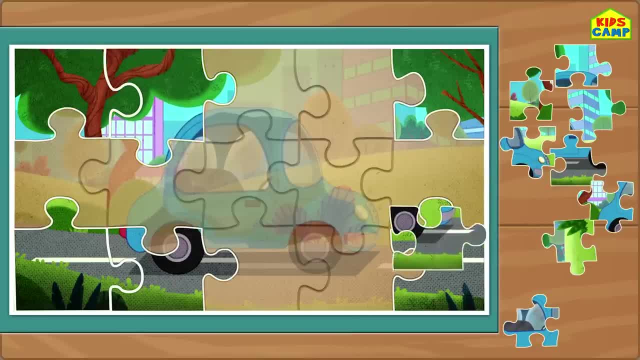 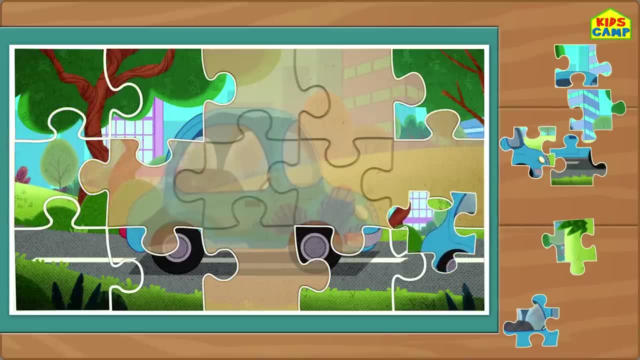 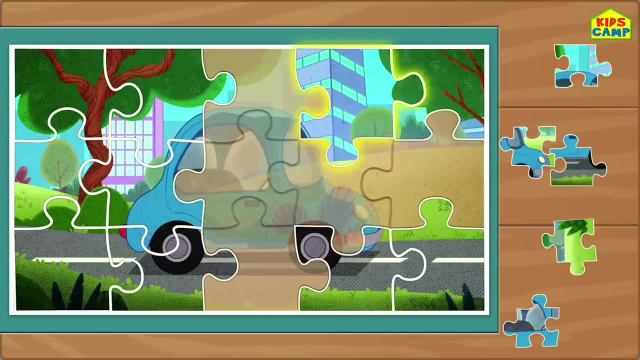 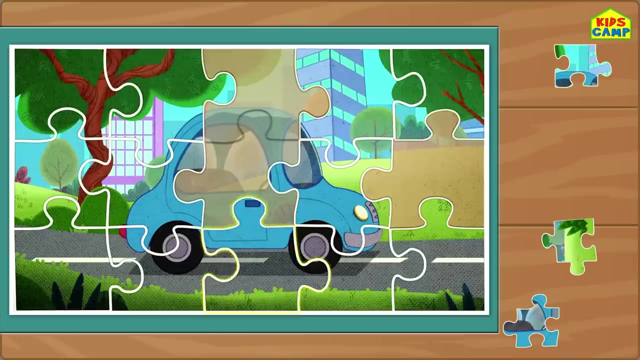 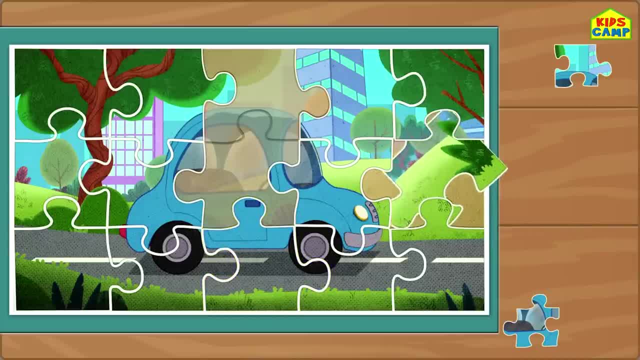 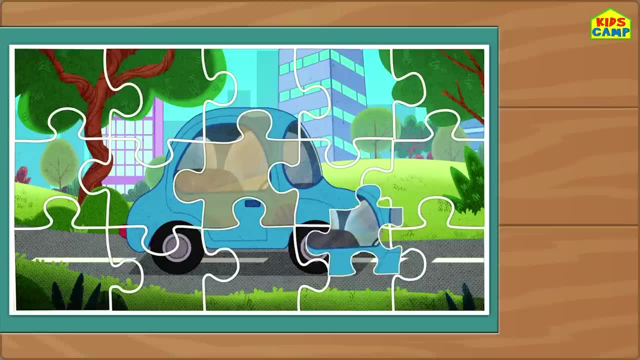 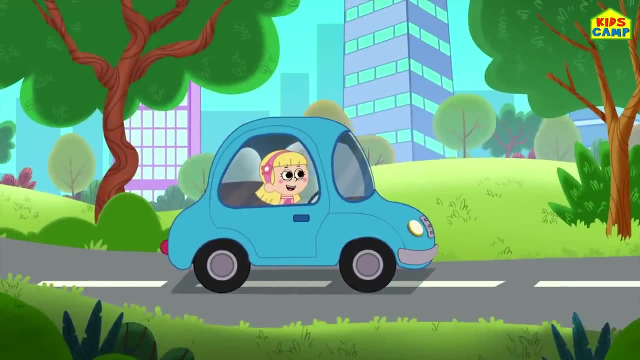 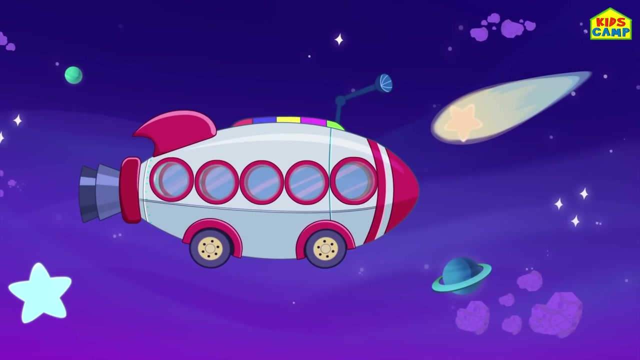 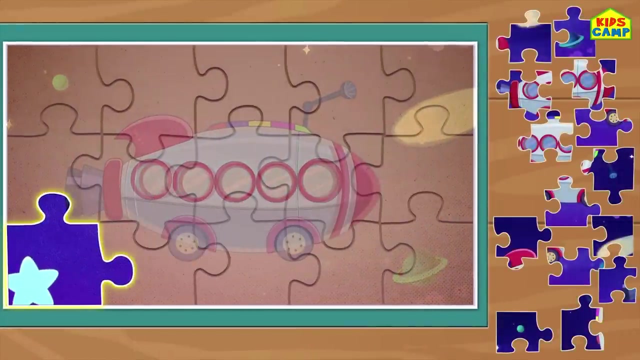 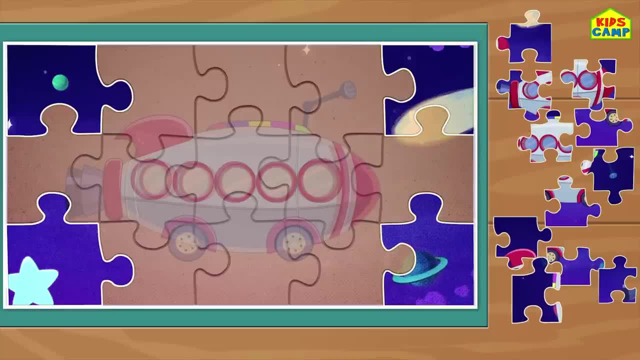 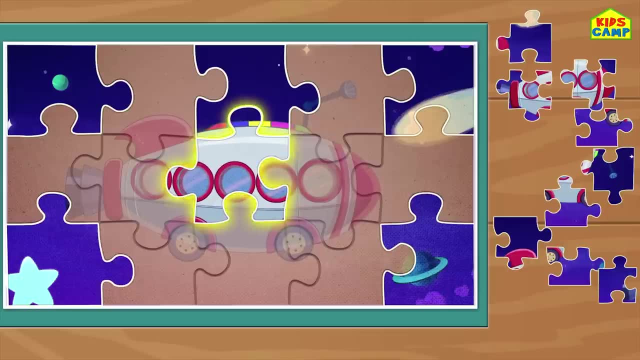 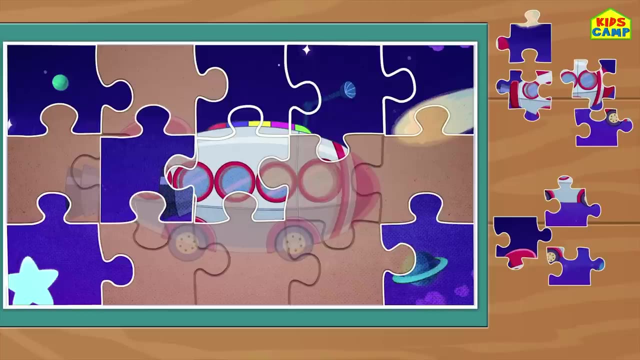 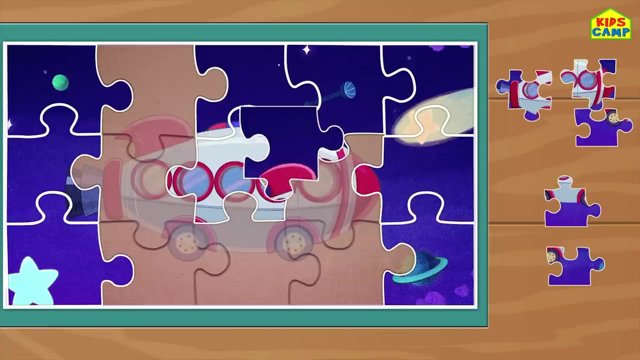 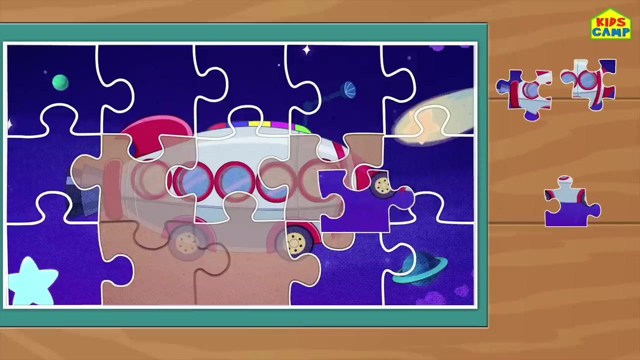 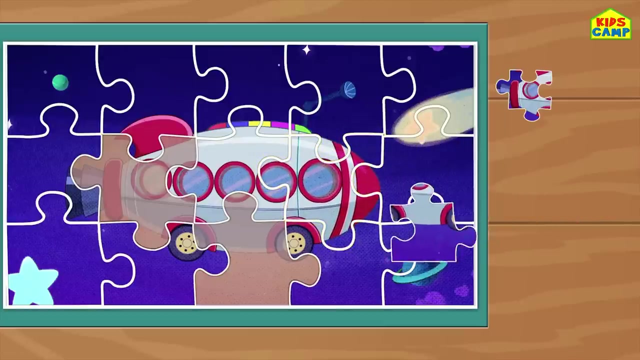 Yay, We got all the four corners. Yes, Wow, The windows Perfect. Woohoo, That's right, We are almost done. Just a few more corners And here to go, Perfect, A few more pieces. Wow, This looks so good. 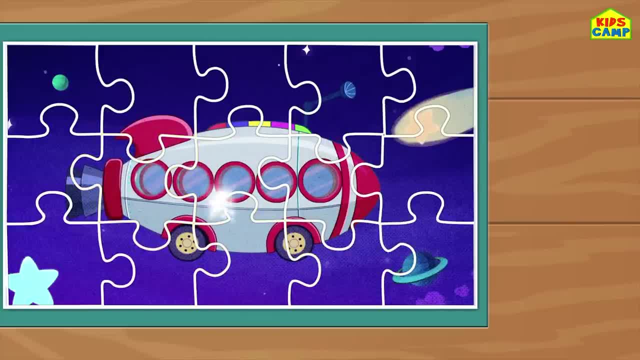 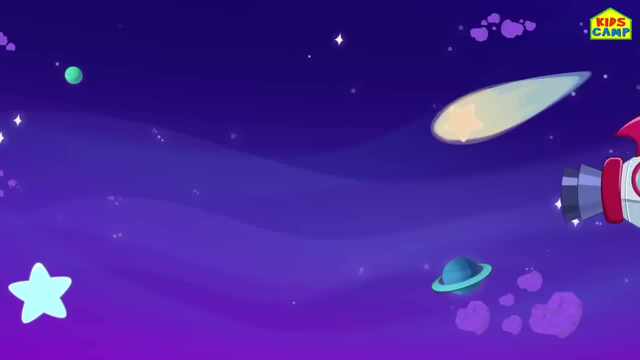 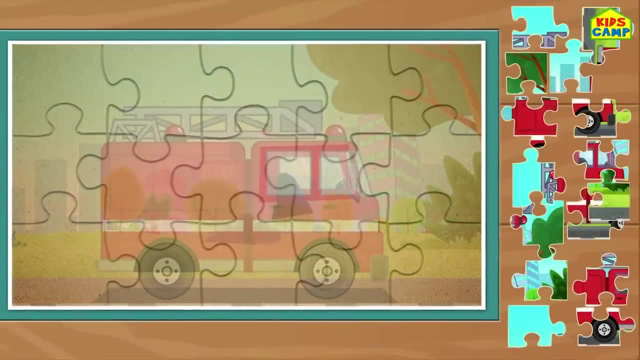 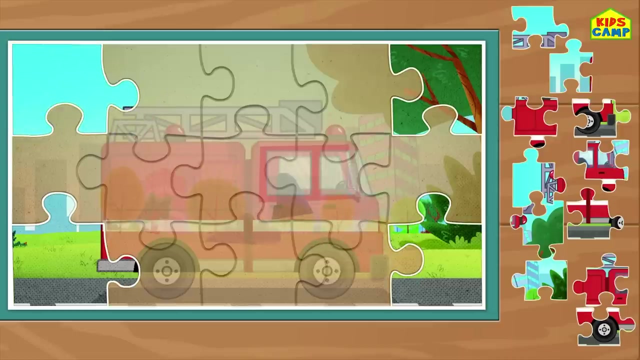 And the last piece: Our spaceship is completed, And here I go. Woohoo, A fire truck Once again. let's start with the four corners. All right, let's get started. A fire truck, And here to go. 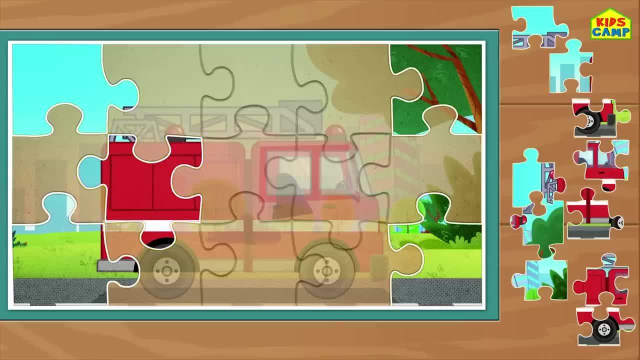 Good job, kids, We are learning. And here I go. All right, let's start with the four corners. Woohoo, The wheels, And here we go. And the second wheel, And here we go, And here we go. 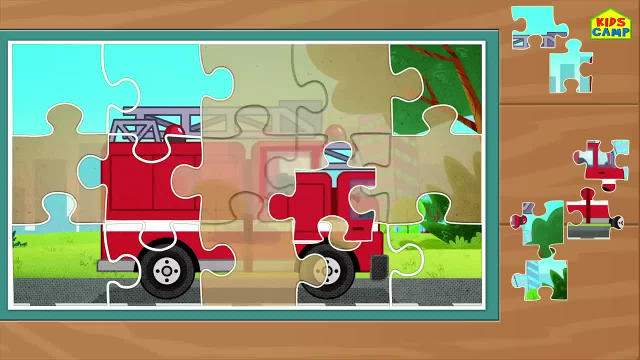 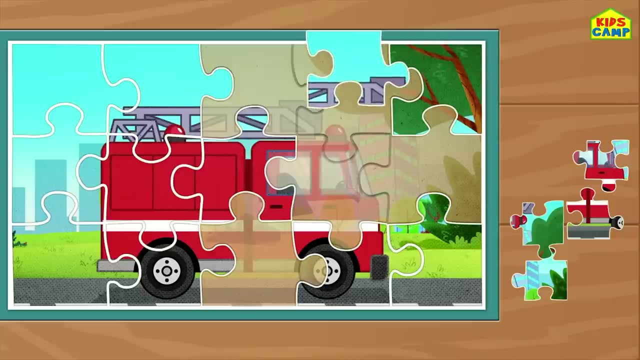 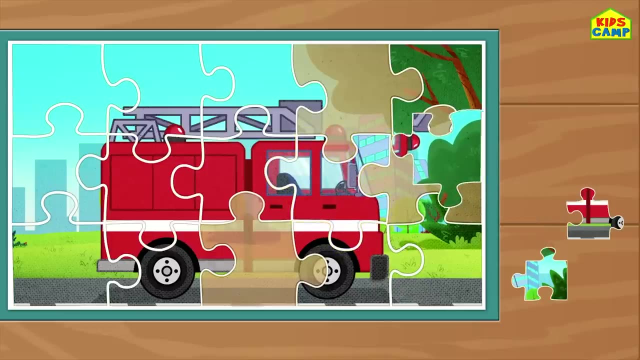 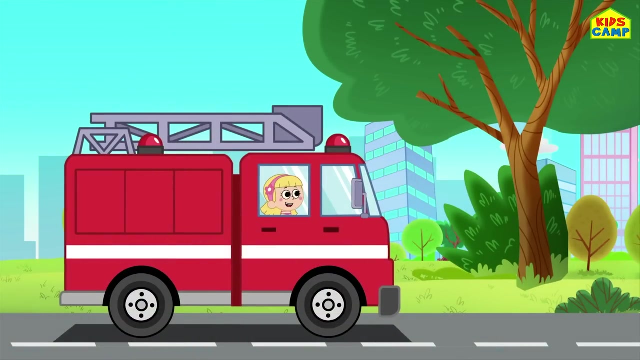 And here we go. Oh, the center piece. Wow, we almost got it. A few more pieces, That fits correctly. Oh, we gotta spin that around. Perfect, And the last piece. We did it. Our fire truck is ready to go. 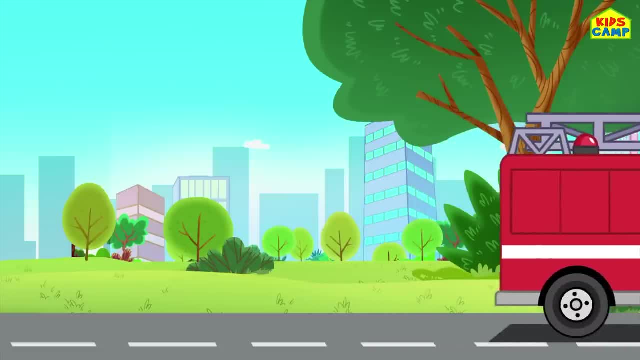 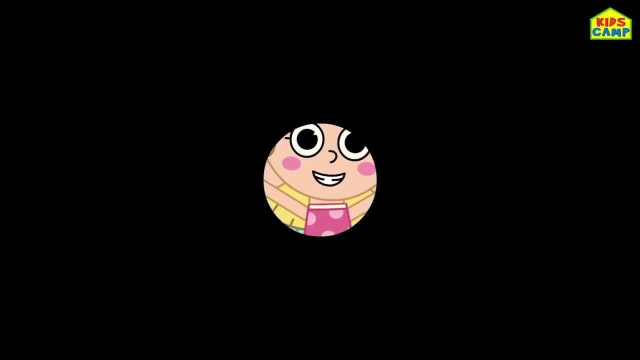 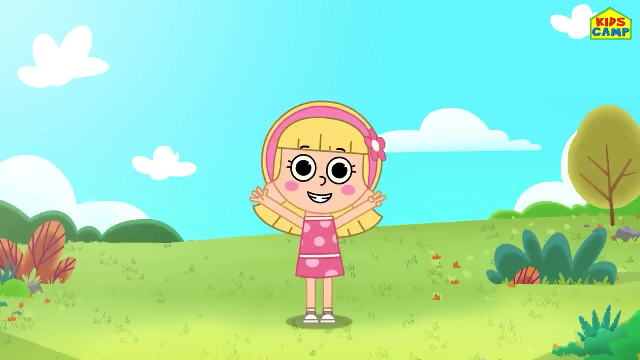 Wow, Yay. This was so much fun solving puzzles. See you soon. Hi everyone, What a beautiful day. I'm Ellie And we are going to play a new game called Find the Matching Pear. That's right, We have to find two similar objects. 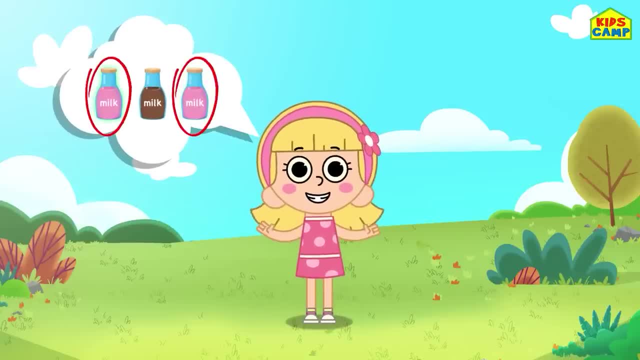 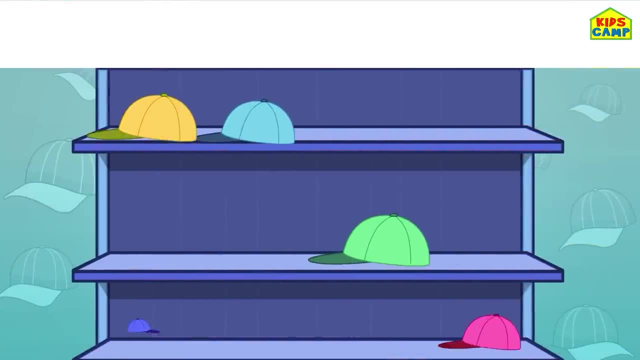 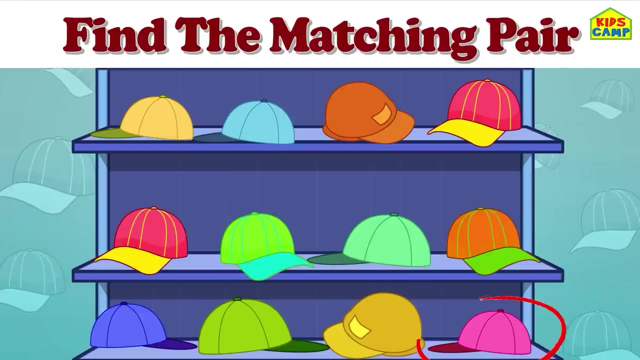 and that's the game. That's simple. Ready, Let's get started. Find the matching. pear, Can you spot two identical caps? No, they are not identical. No, Yes, Yay, We found them. They are two identical caps. 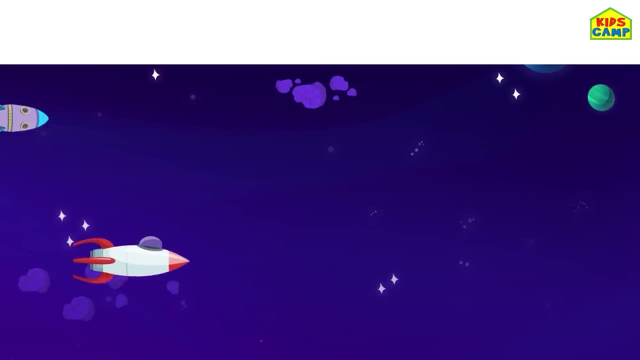 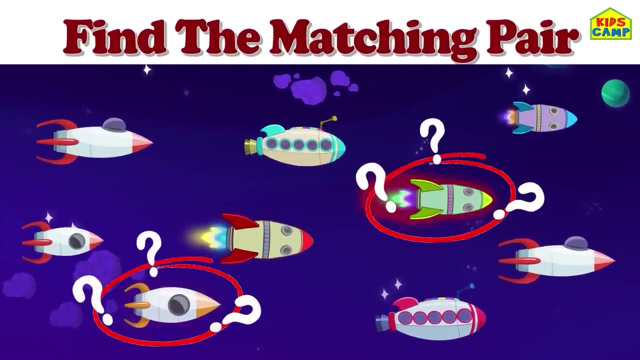 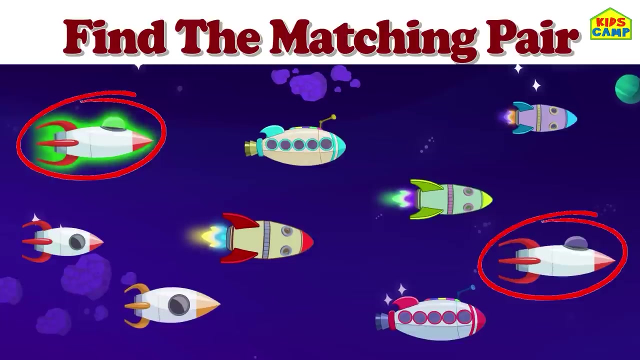 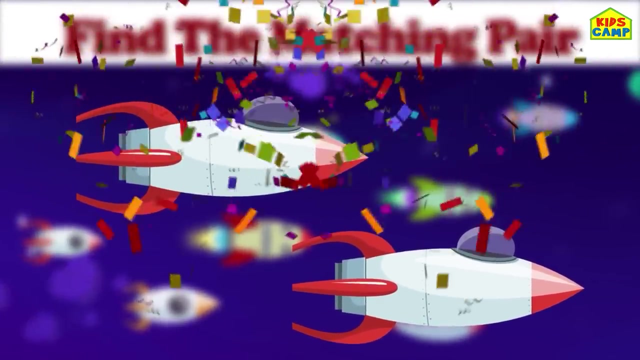 Good job. Let's find another pear, Find the matching rockets, Can you? No, not this one. No, Yes, That's right, They match. Perfect, We found them. This was easy. Let's go to the next one. 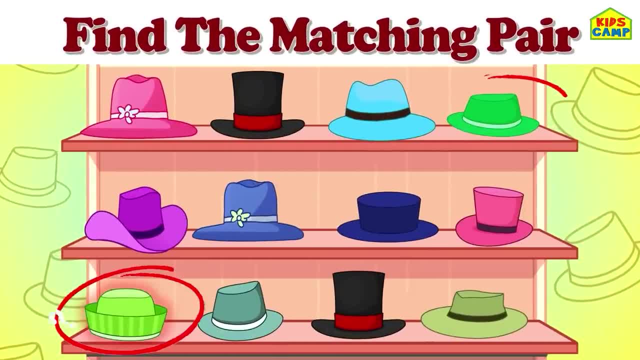 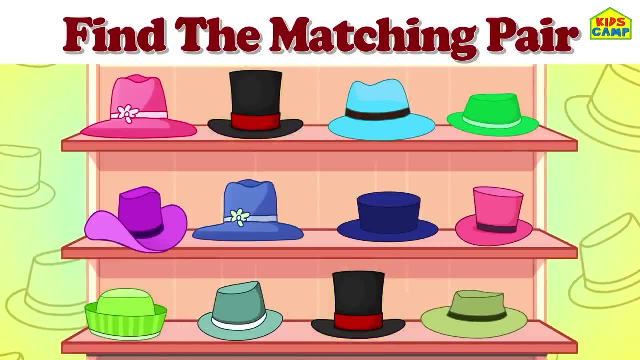 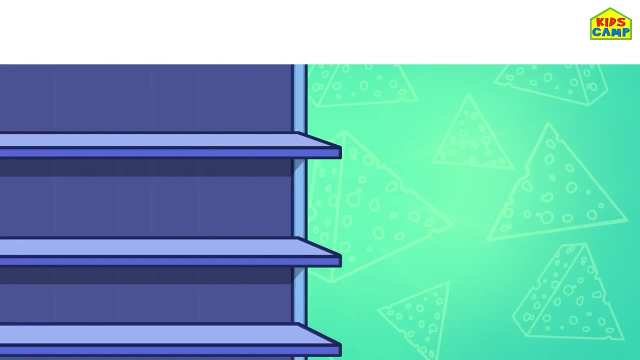 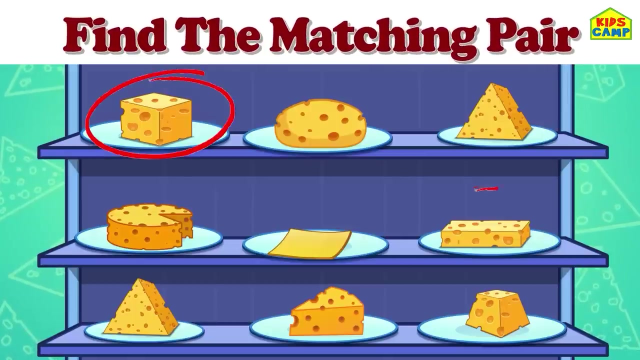 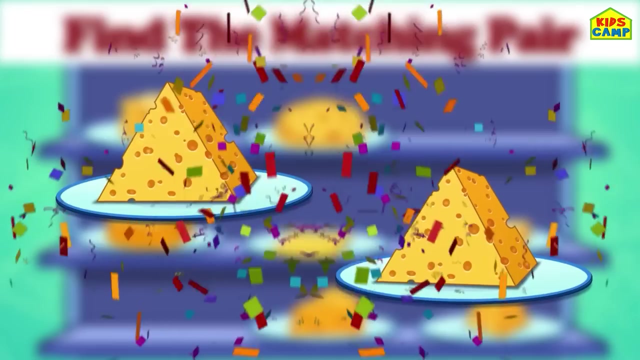 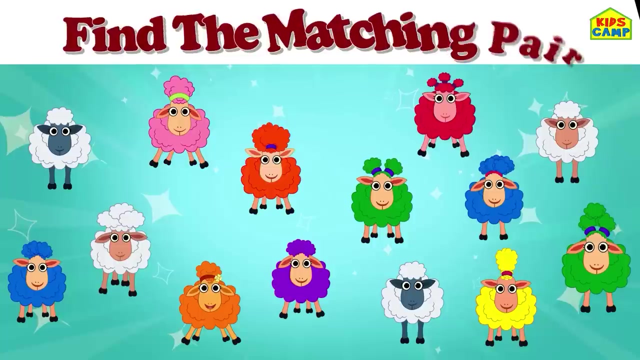 Find the matching hats? No, Yes, We found them, Perfect, pear. Good job, friends. Can you find the matching cheese? No, Definitely no, That's right. These match Perfect, Good job, Good job. Can you find the matching pear here? 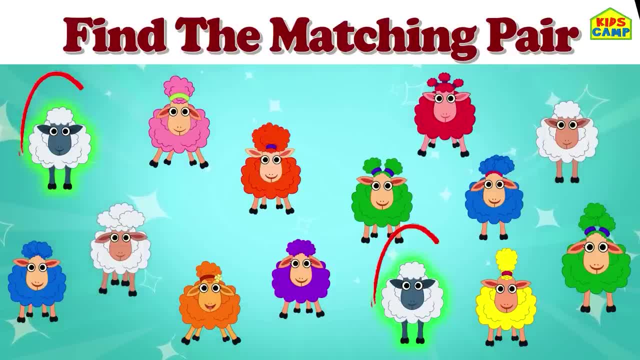 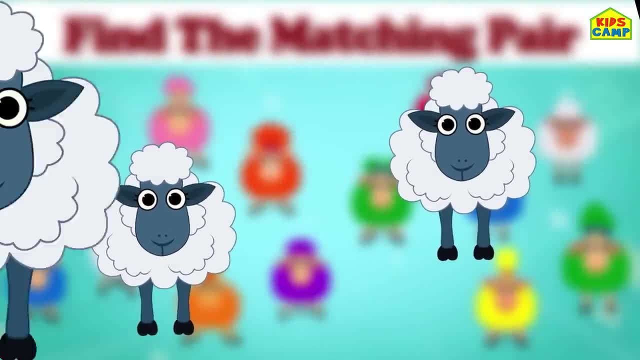 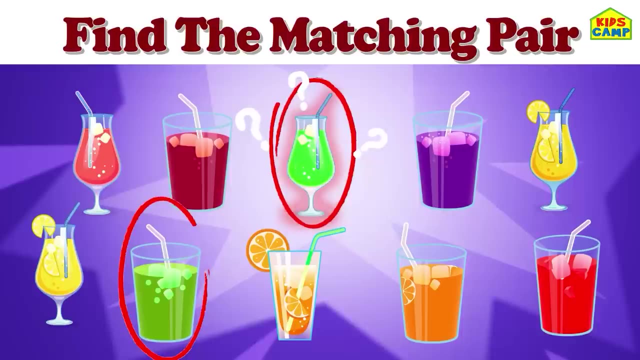 No, they are not identical. Yes, They match. That's right, These sheep match. Perfect. Find the matching coolers. Do these match? No, Do these match No. Yes, We found the pair. Good job, friends. 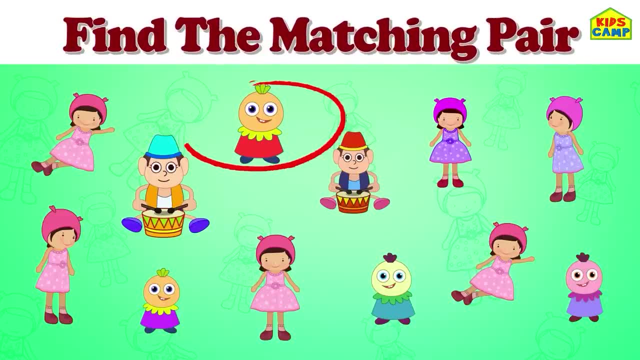 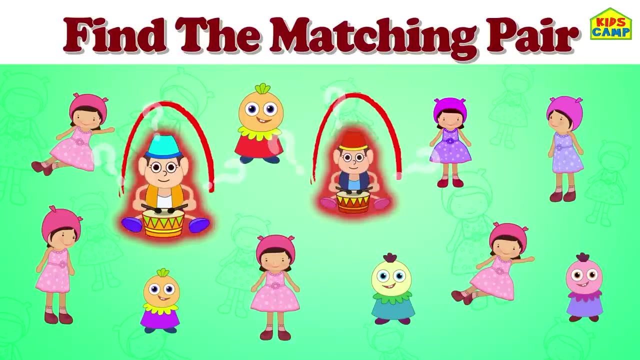 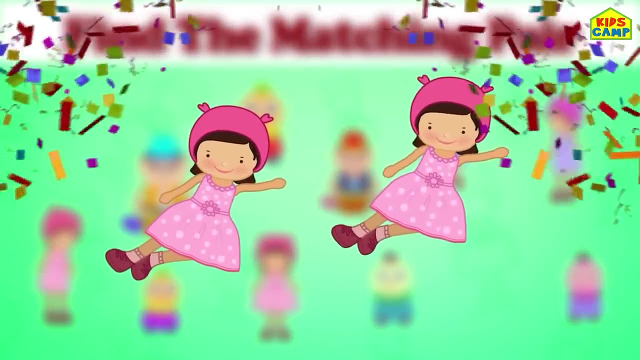 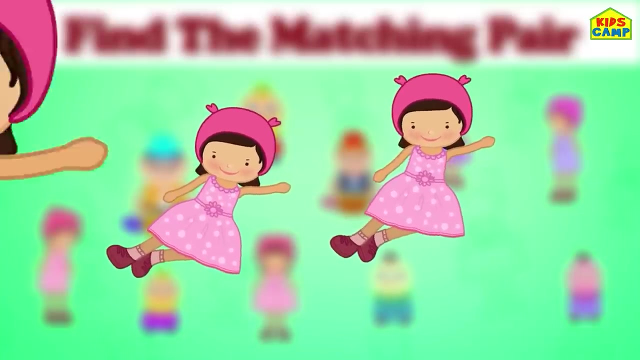 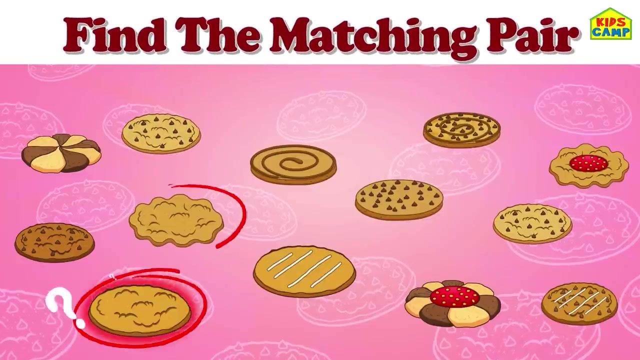 Find the matching pair. Let's look for one. No, No way, That's right. We found the pair. Yay, Good job, friends. This game is so much fun, Ooh Cookies. Find the matching pair- No way. 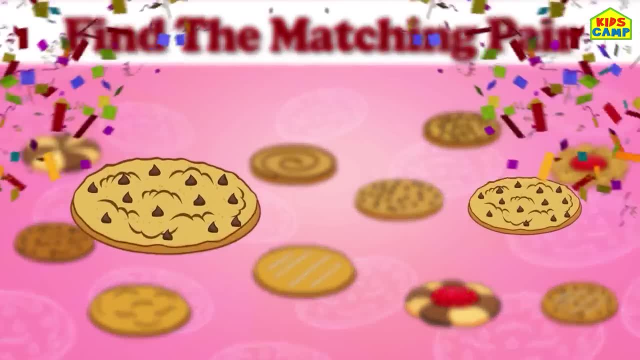 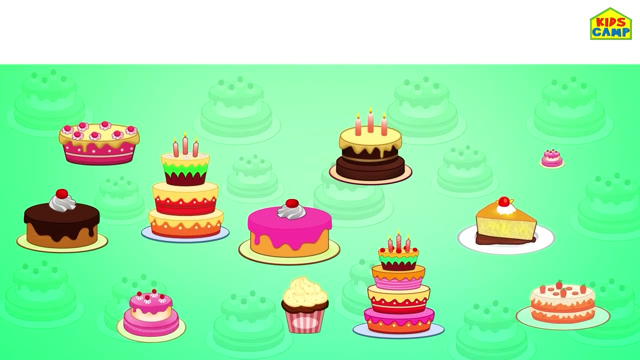 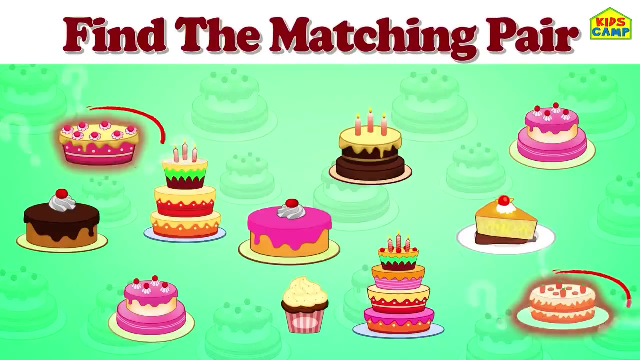 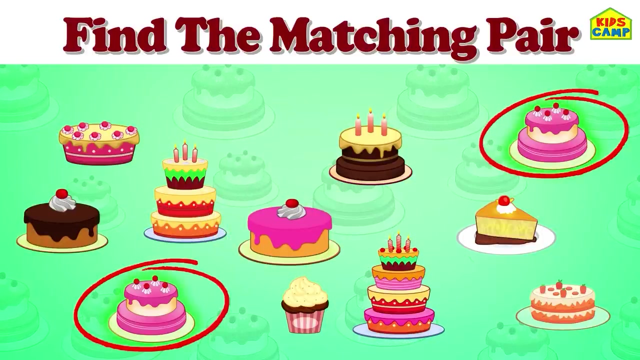 Yes, We found them. I love cookies, Yummy. Let's go to the next one, Hmm, Cakes. Find the matching pair. No, No, No, Yes, That's right, The matching pair of cakes, Yummy. 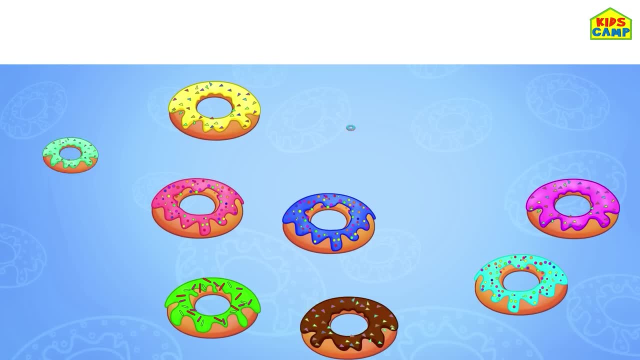 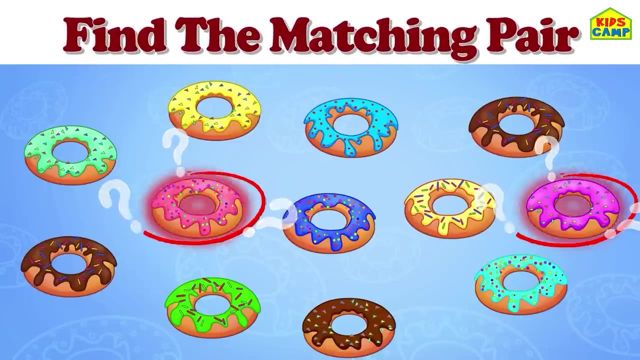 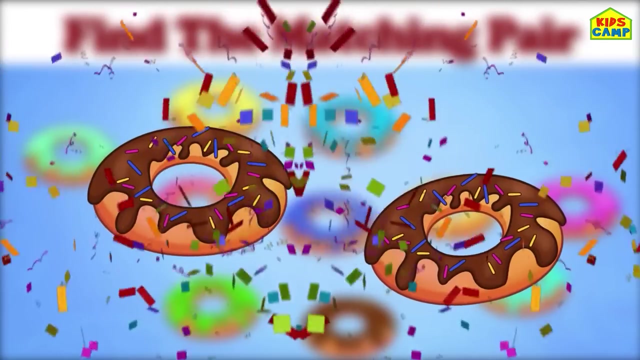 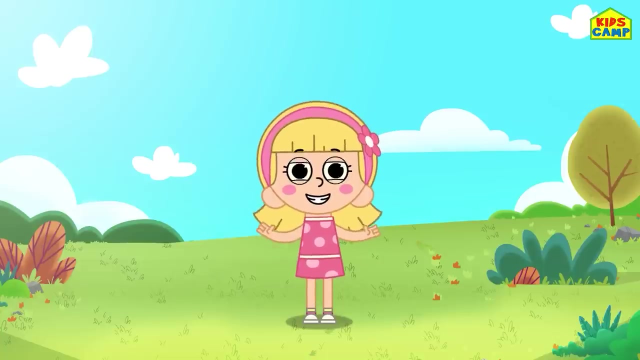 Wonderful. Ooh Donuts Find the matching pair. No, No, Yes, We found the matching pair. These match. This was such a fun game, friends, Keep watching Kids' Camp. Bye-bye, Hi, I'm Elli. 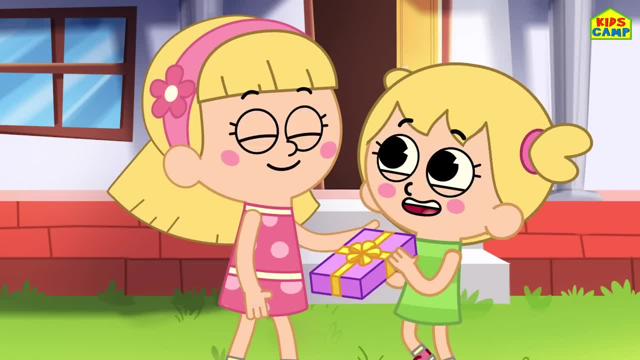 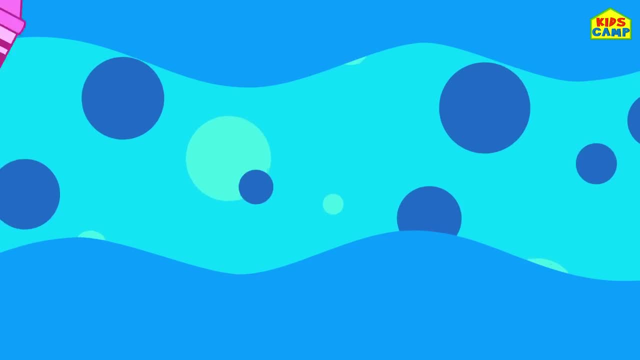 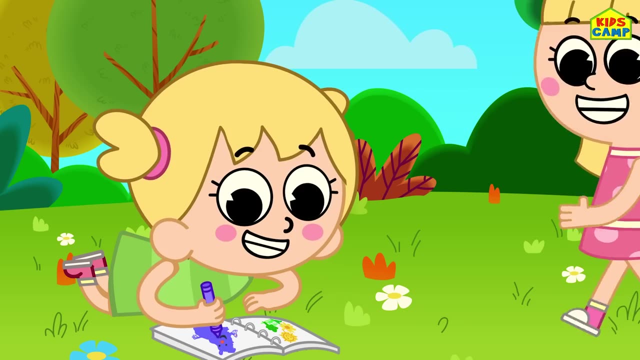 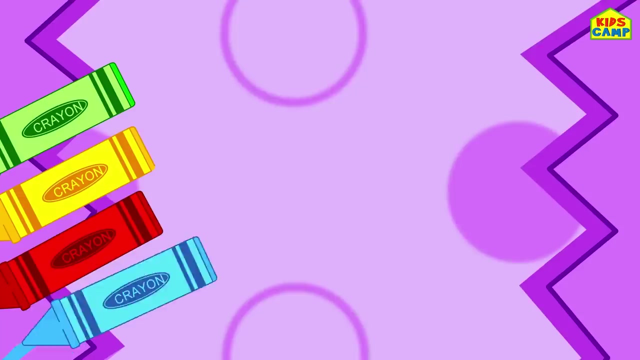 And I got Eva a gift, A gift for me, Thank you Open it. Wow, What is this? A box of crayons. Ha, A box of crayons, one for you. A box of crayons so colorful too. 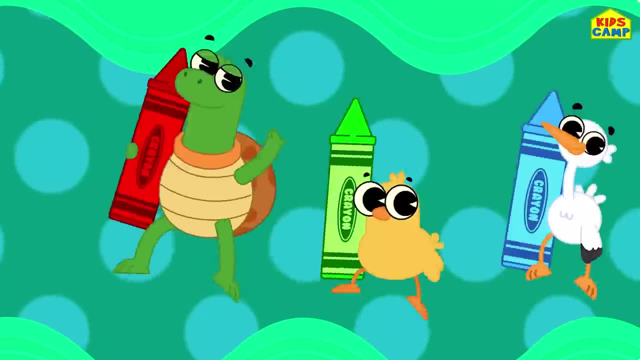 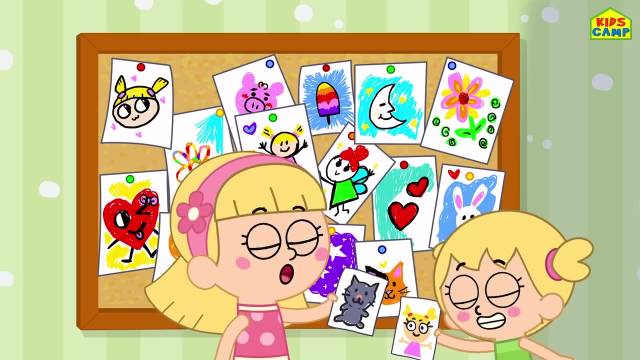 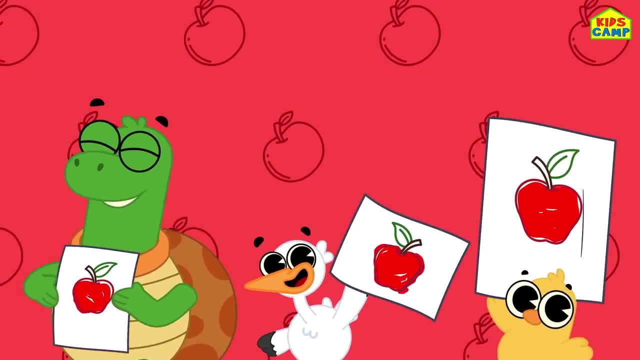 A box of crayons for me and you. A box of crayons with red, green, blue, Oh Oh. This one is red, A bright color, red Color, an apple with a color red. This one is green: A cool, nice green. 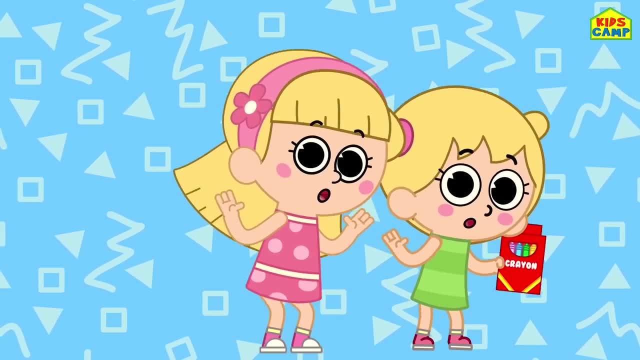 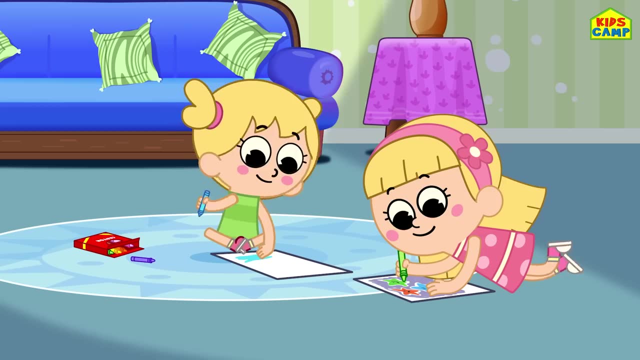 Color a leaf. Now, this one is green. A box of crayons, one for you, A box of crayons so colorful too. A box of crayons for me and you. A box of crayons with red, green, blue. 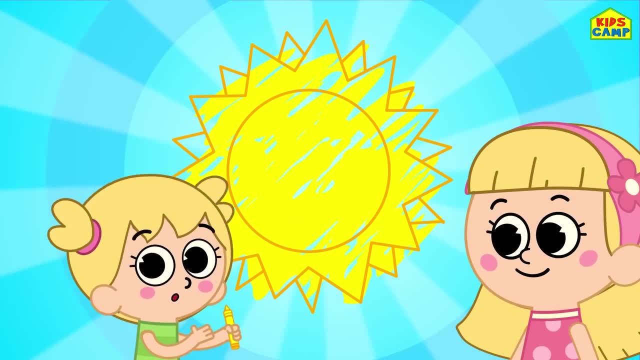 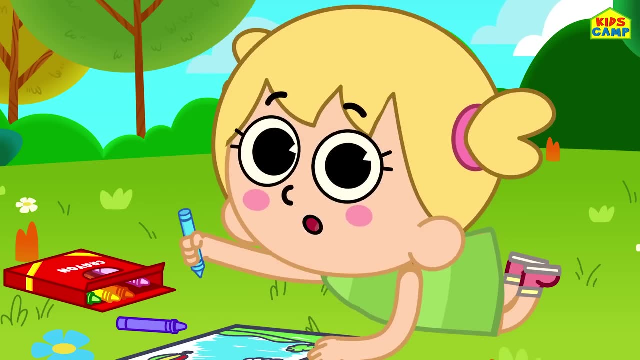 This one is yellow: A bright, happy yellow. Color the sun now a bright, happy yellow. This one is blue: Cool, cool blue Color the sky blue. This one is blue: A box of crayons, all brand new. 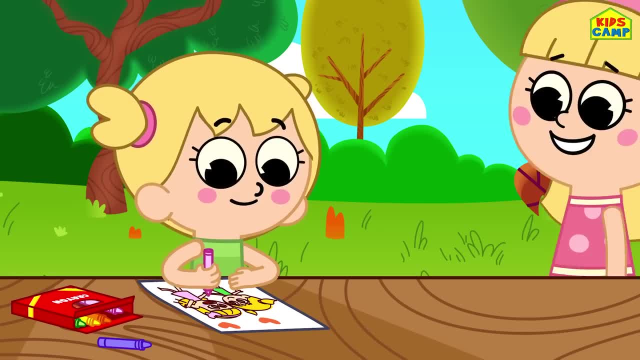 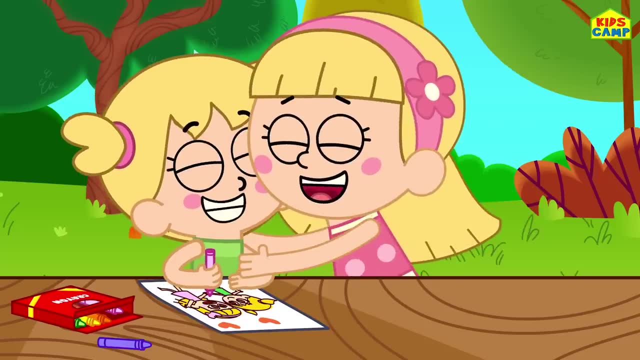 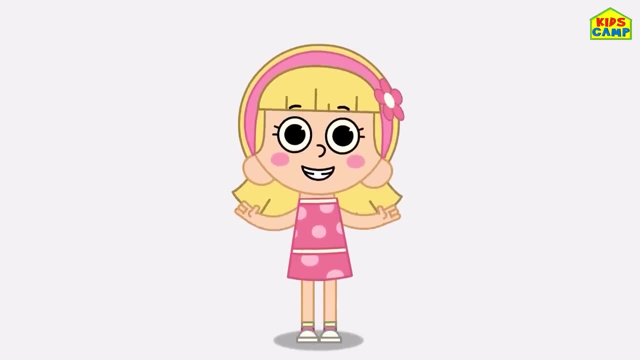 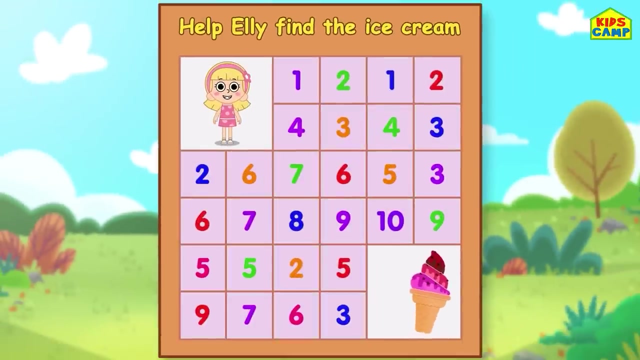 A box of crayons for me and you. A box of crayons, all brand new. A box of crayons just for you. Didn't you love them? I love it too. Let's go to the next number Two. Yay, Oh, That's not right. 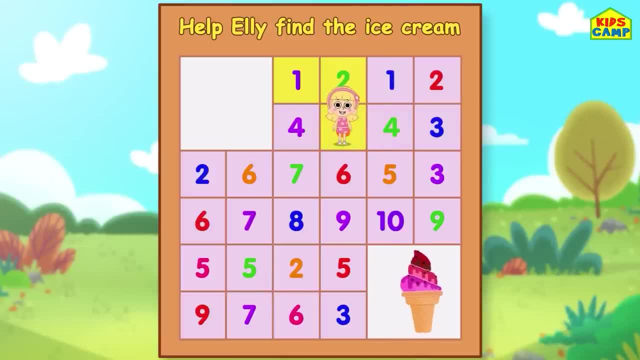 Aha, That's right. That's three. Let's go to the next one, Number four: Yay, Aha. Number five: Good job, friends. Oops, That's not right. Yay. The next number is six, That's right. Wonderful, Next seven. 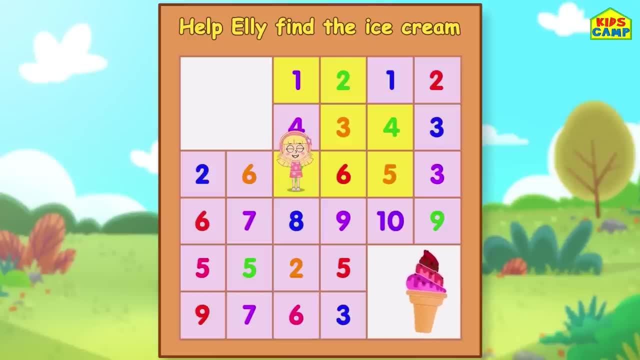 We're almost there. And eight, Yay, Uh-oh, No, That's right. Nine And ten: Yay, We did it. You helped me reach the ice cream, Thank you, Oh, It's Eva's turn now. Can you help her reach the donuts? 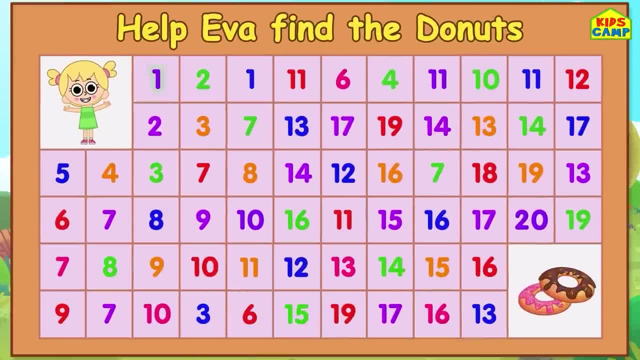 Let's get started, Yay, Yay. Let's start with number one. One, Two, Three, Good Four, Uh-oh, No, No, No, That's right. Number five: Good Six, Keep going. Seven, Eight, Yay, Oops, That's not right. 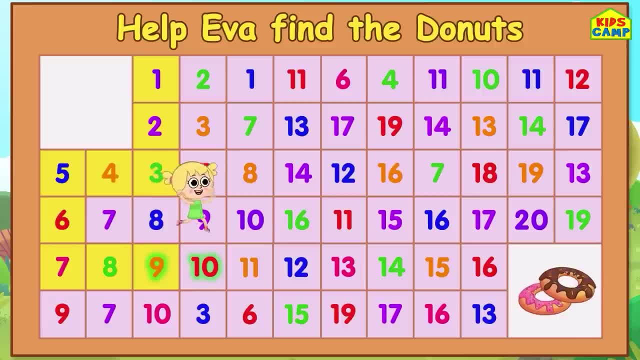 That's right. Nine And ten, Eleven, Keep going. Yay, We're on twelve. What comes after twelve? Uh-oh, No, Not that one, That's right. Thirteen And fourteen. Next is fifteen. Woohoo, Only five more to go. 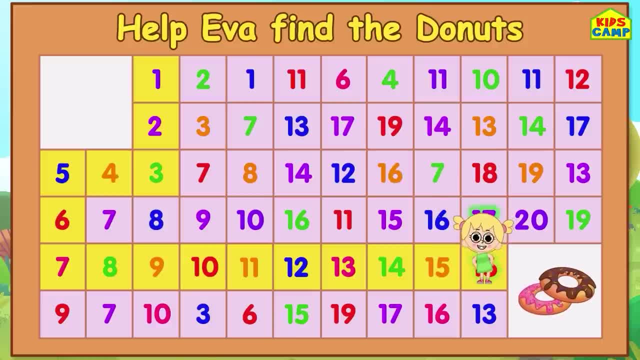 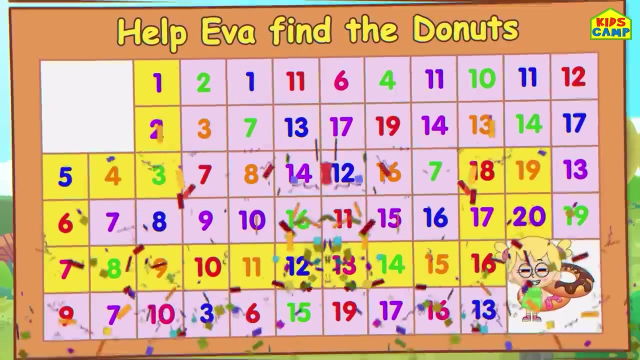 Sixteen, That's right. Seventeen. Next is Eighteen, That's right. Nineteen- We're almost there. And twenty, That's right, We did it. Woohoo, We helped Eva find the donuts. Good job, friends, Bye. 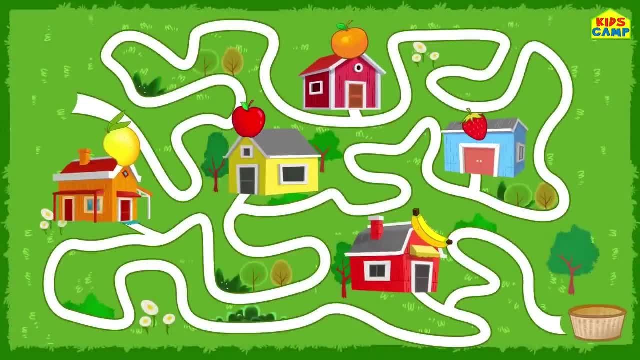 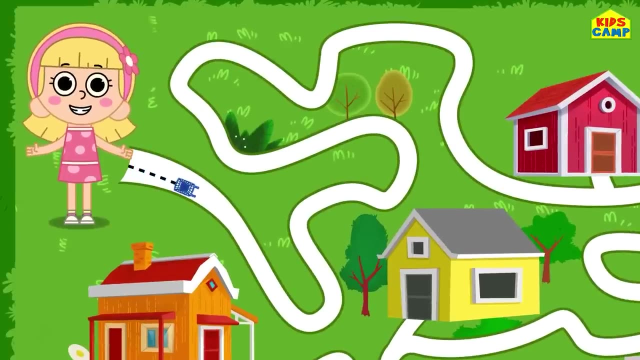 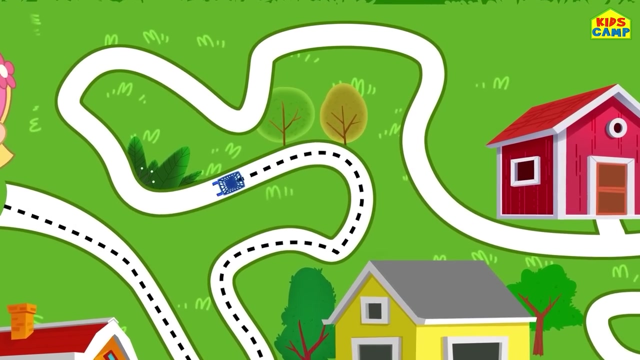 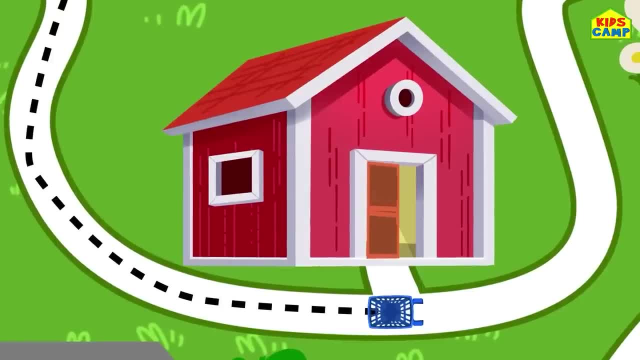 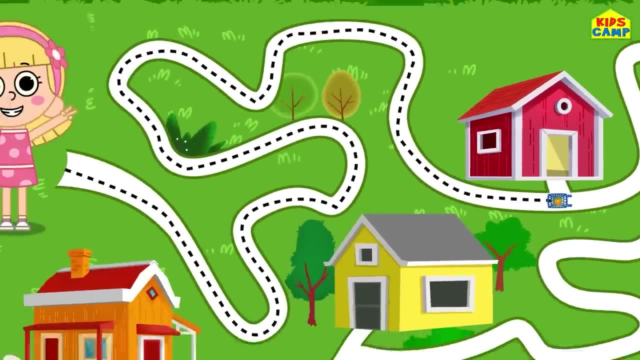 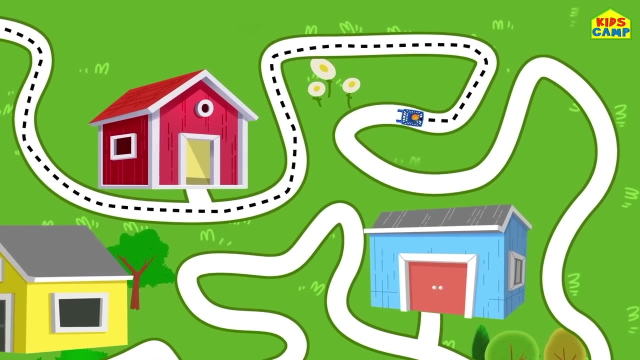 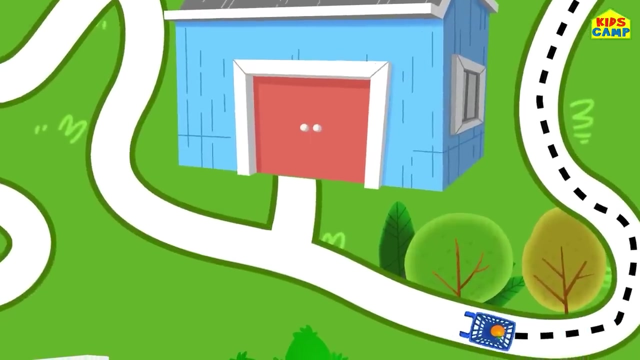 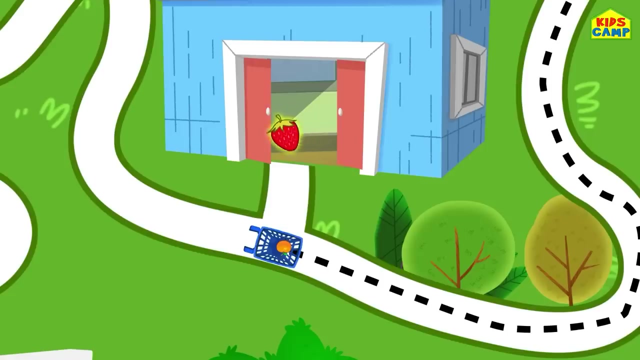 Knock knock, Hi. Do you have any fruit? Ooh, An orange Into my cart, Wonderful. Let's keep going. Ooh, Knock, knock. Do you have any fruit? Aha, A strawberry Into the cart, Wonderful. 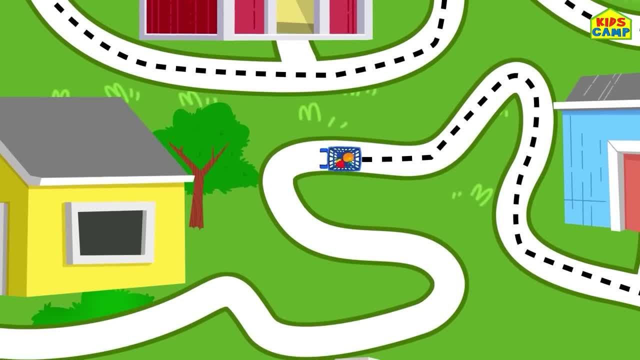 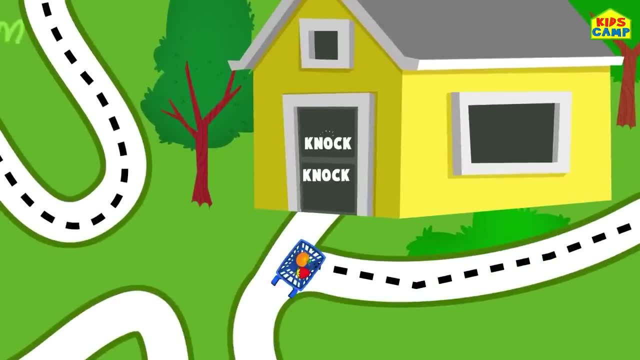 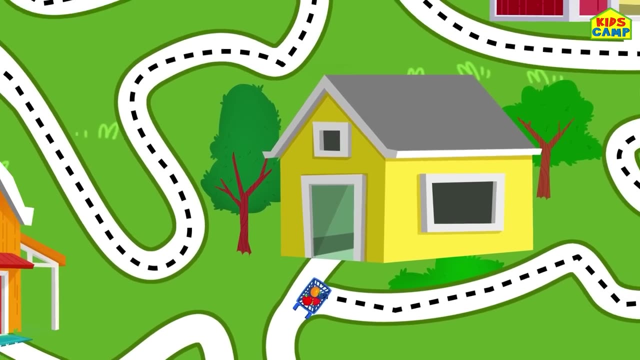 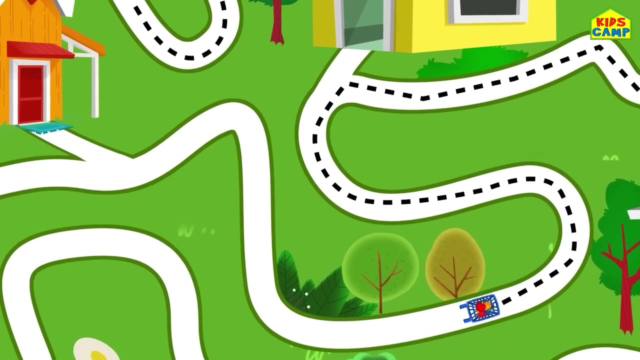 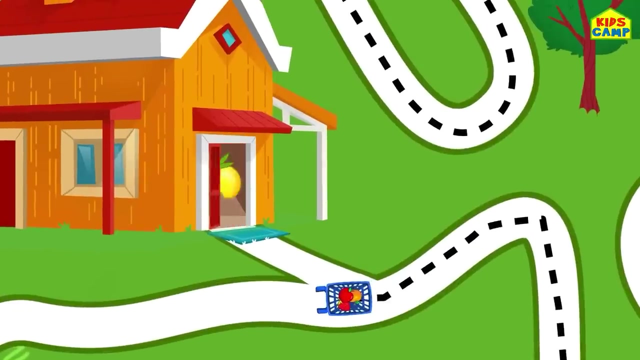 Let's get going. Knock-knock, Knock-knock. Hi, Do you have a fruit? Oh, My favorite, An apple Into the cart. Yay, Let's keep going, Knock-knock. Do you have some fruit? 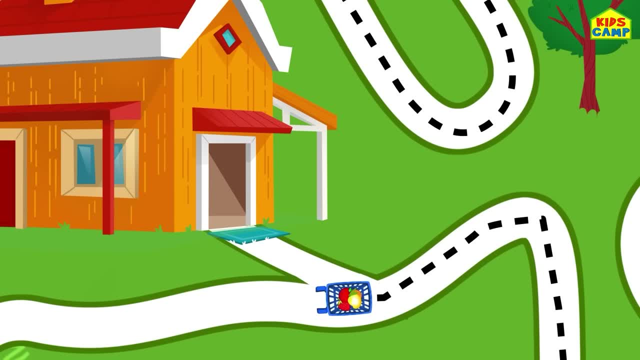 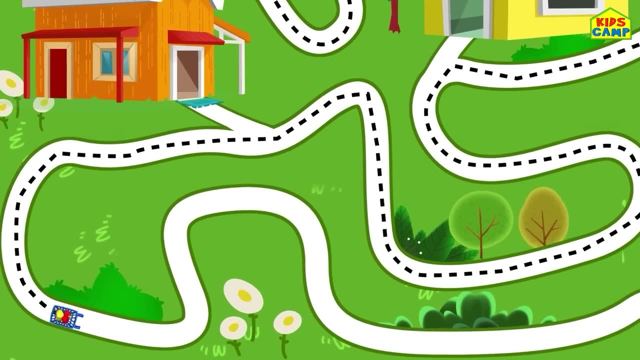 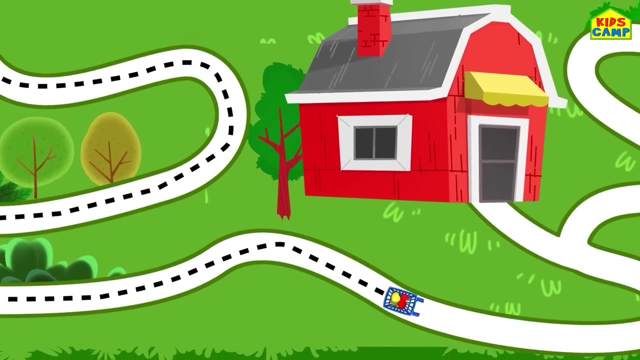 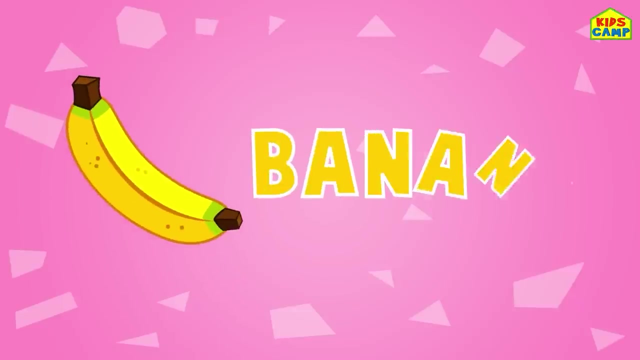 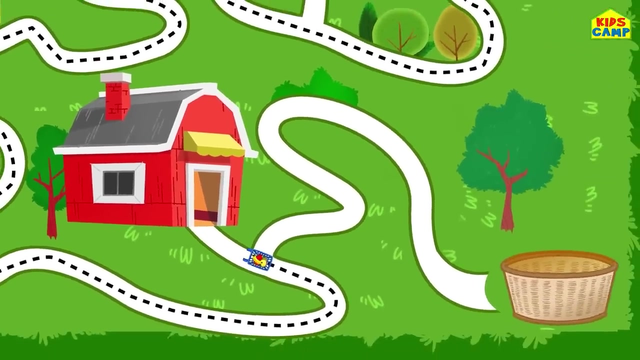 Oh, A mango Into the cart, Let's get some more. Keep going, Knock-knock, Knock-knock, Knock-knock. Hi, Do you have some fruit? A banana, Yay, Into the cart, Let's keep going. 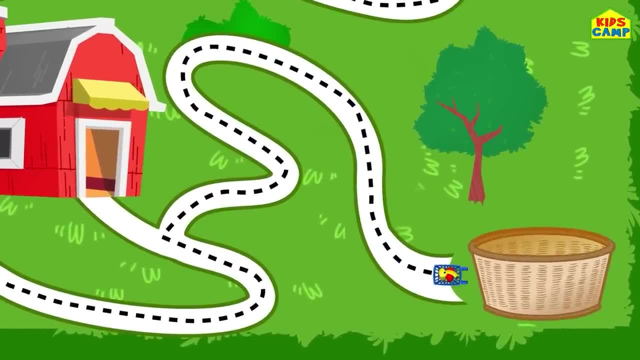 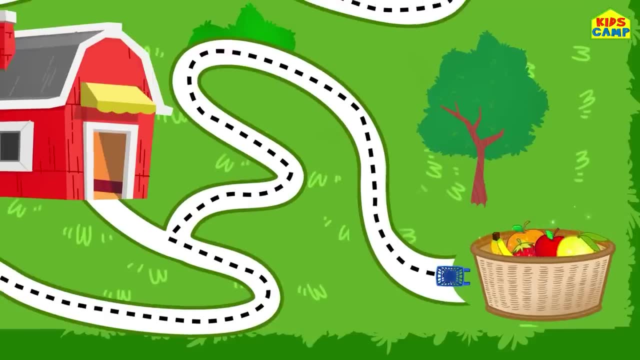 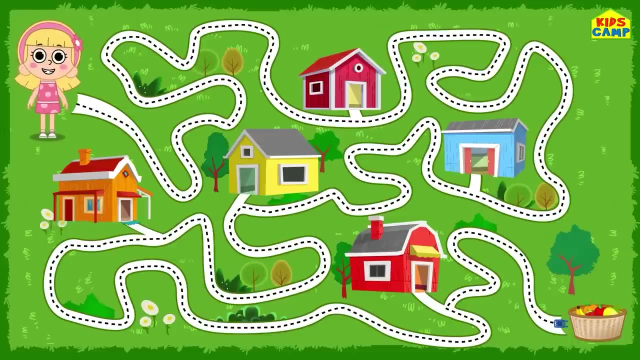 Yay, We've collected all our fruits. What did we get? A banana, a mango, an apple, a strawberry and an orange. Good job, Thank you so much for helping me find my fruits and collecting them in my basket. Thank you. 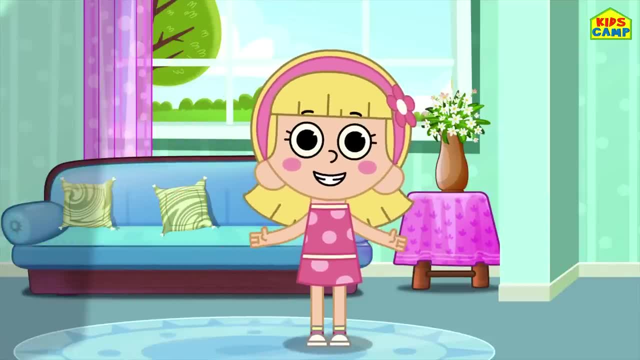 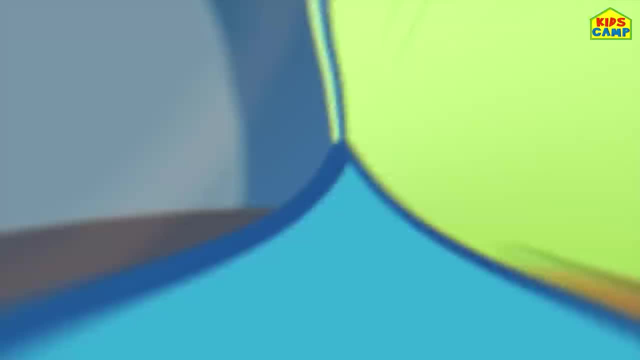 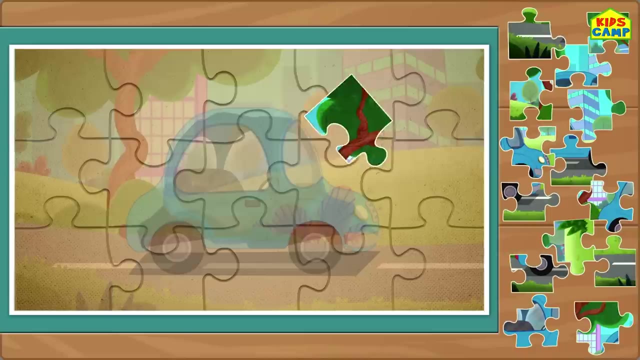 Hi kids, I'm Ellie And today we are going to play with puzzles. Don't we all love puzzles? That's right. Let's start. Oh, That's a car. Let's put all the pieces together. Let's start with the corners. 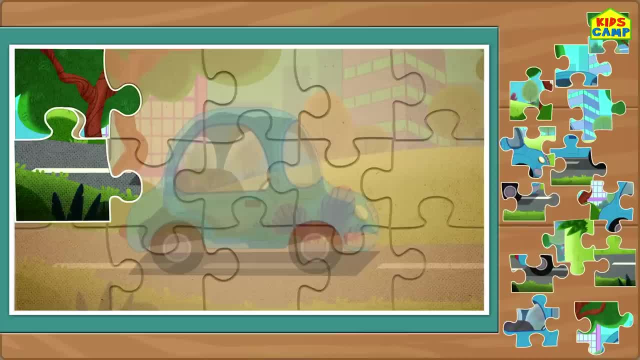 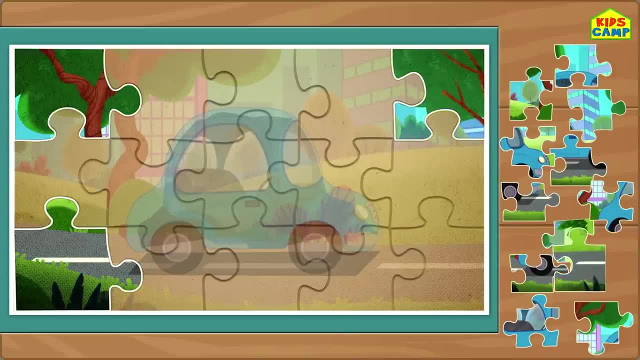 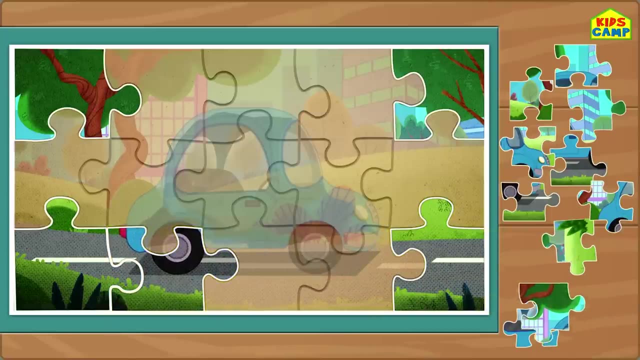 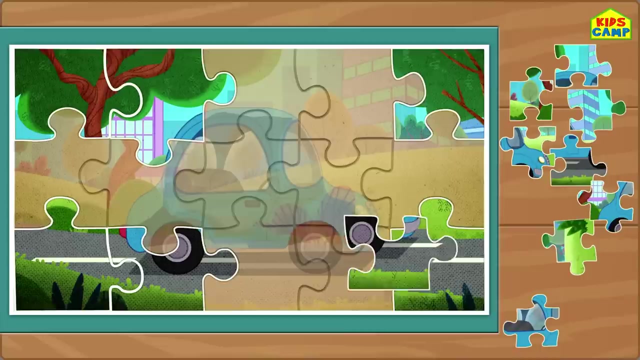 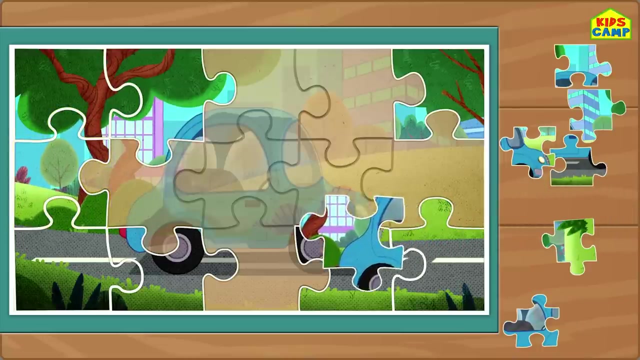 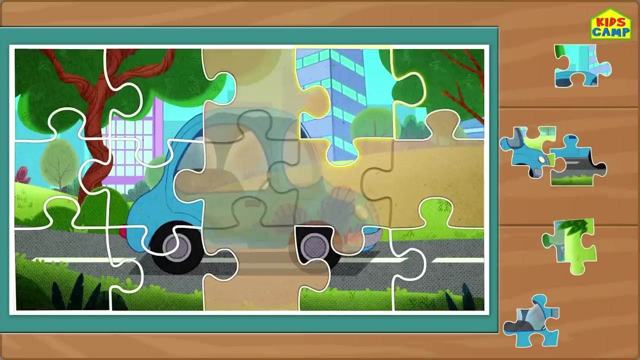 That's right, It goes right there. That's right. Perfect, We got all the four corners. No, that goes up there. That's right. Another wheel, Perfect. Great, Uh-oh, That's right. Wow, This is so much fun. 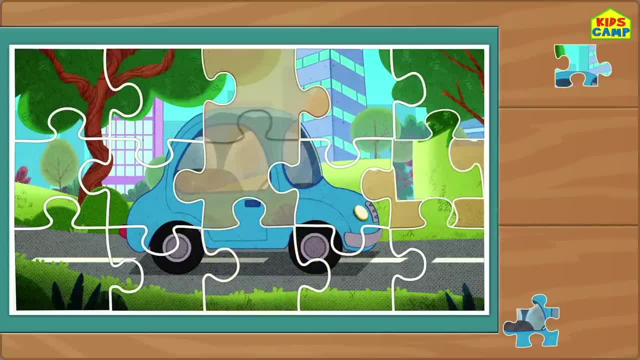 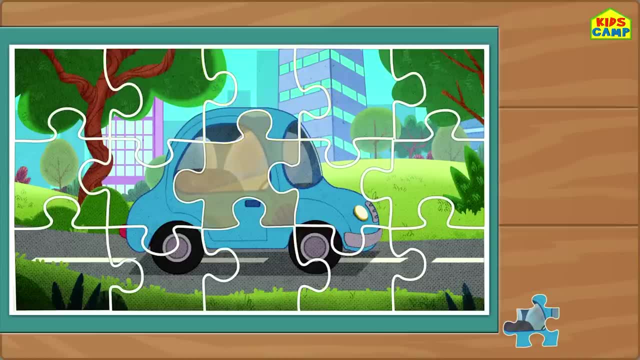 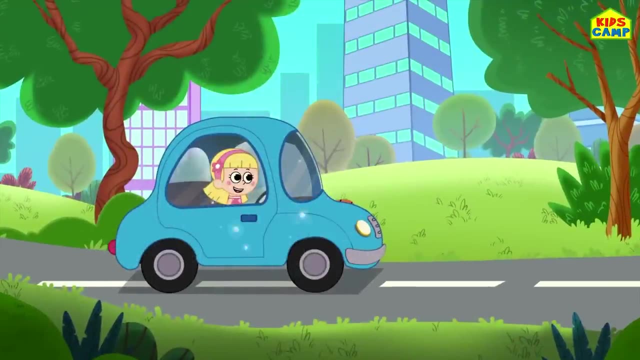 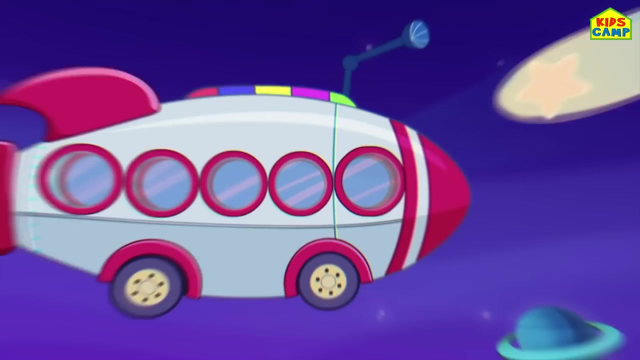 I like puzzles, don't you? No, no, That doesn't seem right Now. it is Perfect. And the last piece. Woohoo, We did it. kids, There goes my car, Vroom, vroom, And now we have a spaceship. 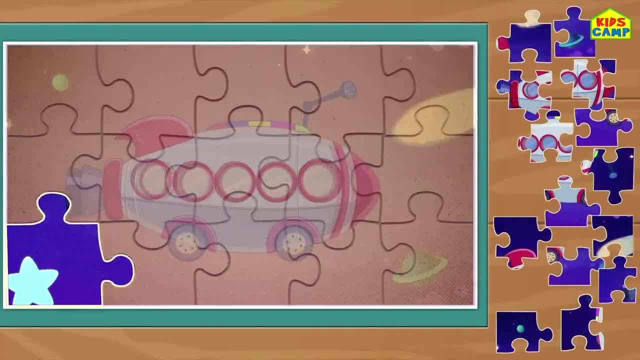 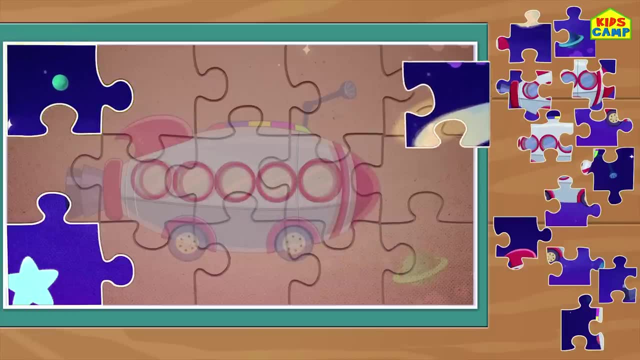 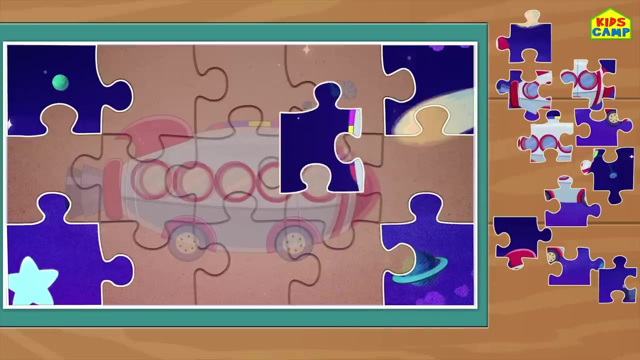 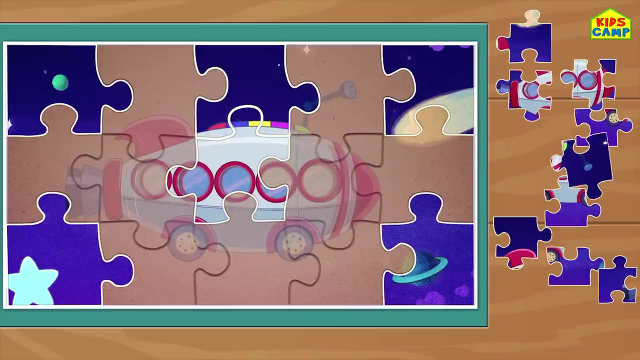 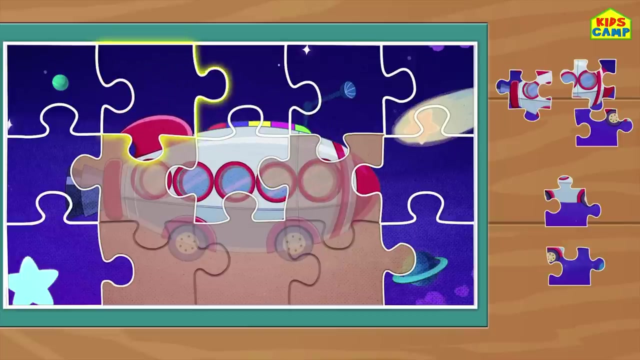 Let's start with the corners. That's right. I'm going to have a good look at all the pieces. I hope you like them. Yay, I'm going to have a good look at all the pieces. got all the four corners, yes, wow, the windows. perfect, that's right, we're. 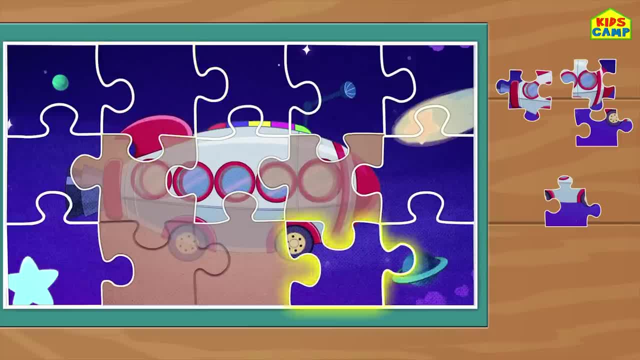 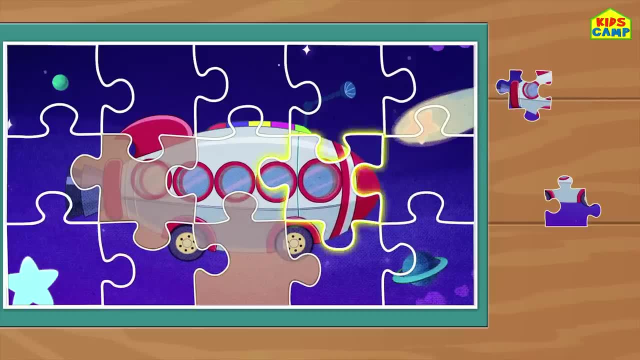 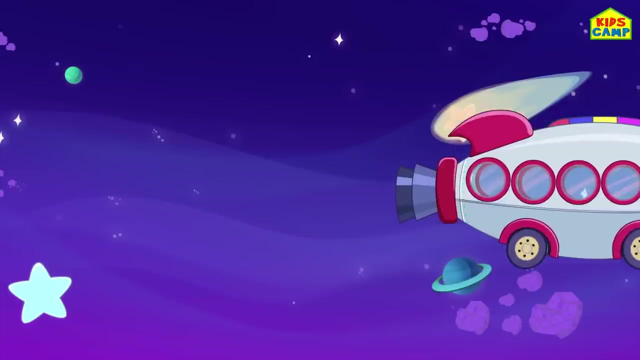 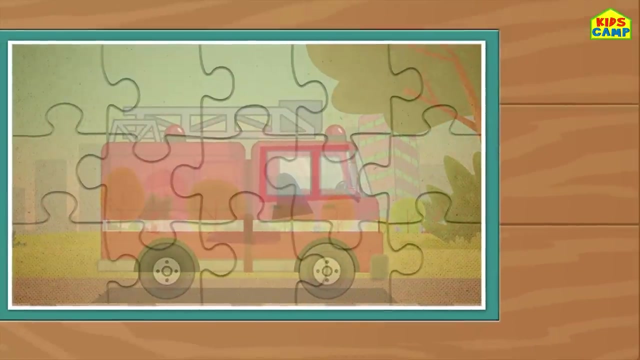 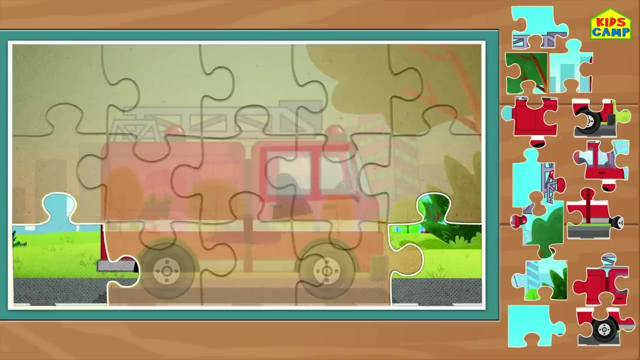 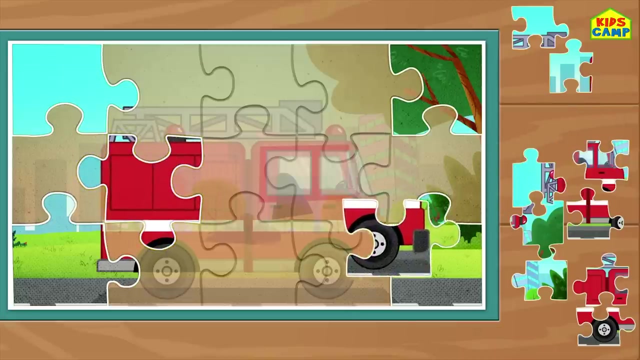 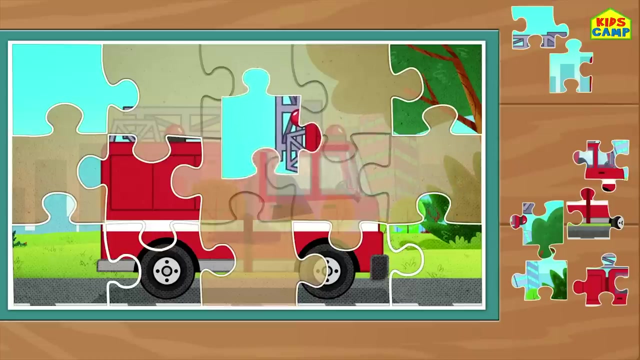 almost done. just a few more to go perfect. a few more pieces- wow, this looks so good. and the last piece: our spaceship is completed. and here I go, a firetruck once again. let's start with the four corners. good job, kids, we're learning the wheel and the second wheel. 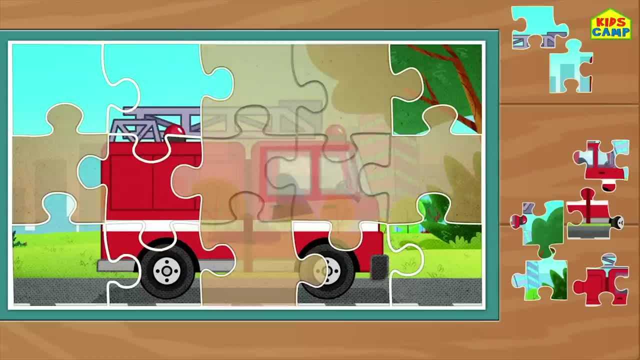 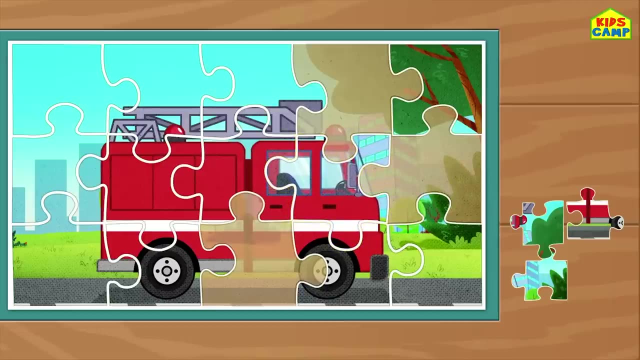 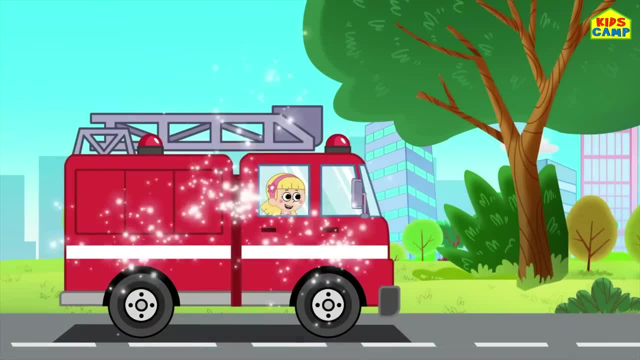 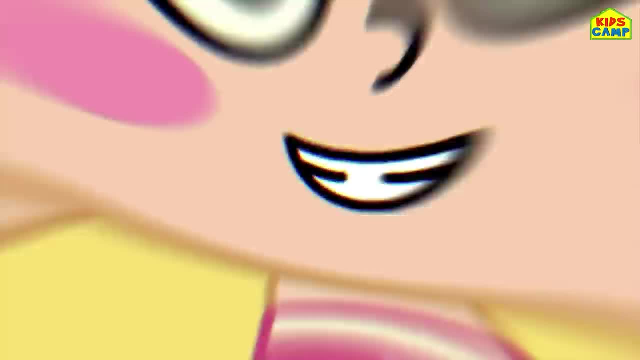 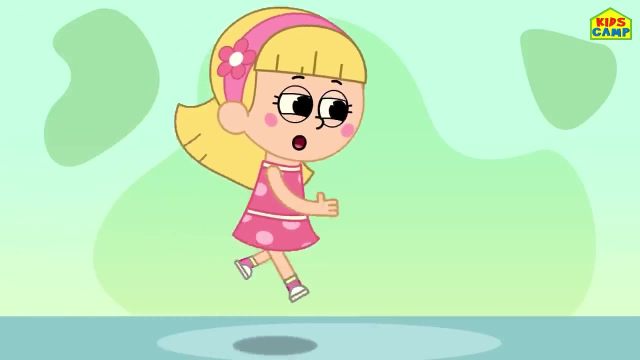 we did it. we did it. Our firetruck is ready to go. Wow, Yay, This was so much fun solving puzzles. See you soon. Hi kids, I'm Ellie and I'm going to put up some pictures in Eva's bedroom. 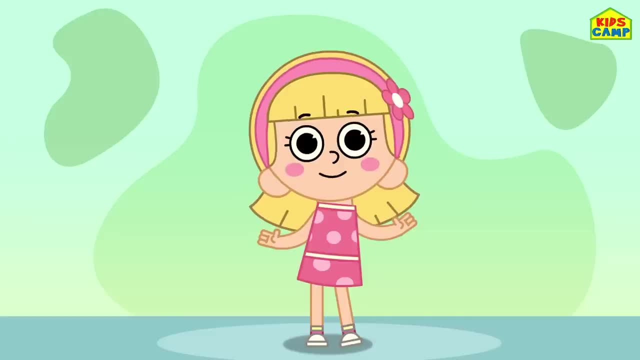 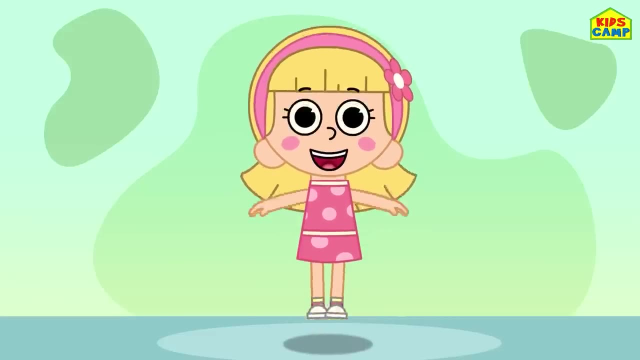 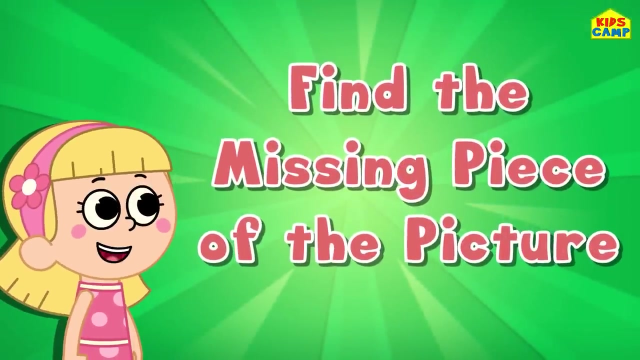 But there's just one tiny problem. There seems to be a missing piece in each picture. Can you help me find it? Woohoo, Let's get started. This is going to be a fun game. Let's find the missing piece. 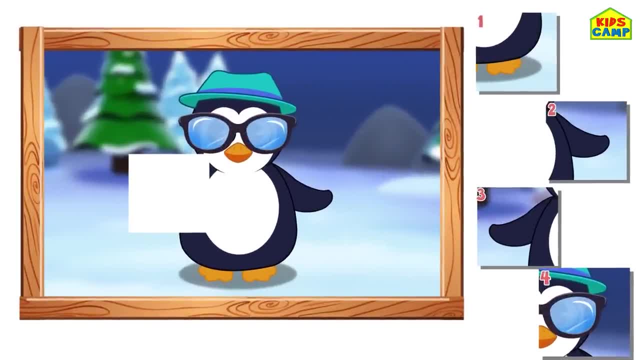 Hmm, do you know which one is the right piece? Let's try. Is number two the right piece? No, it isn't. Is number one the right piece? Uh, oh, it isn't. Is number four the right piece? No. 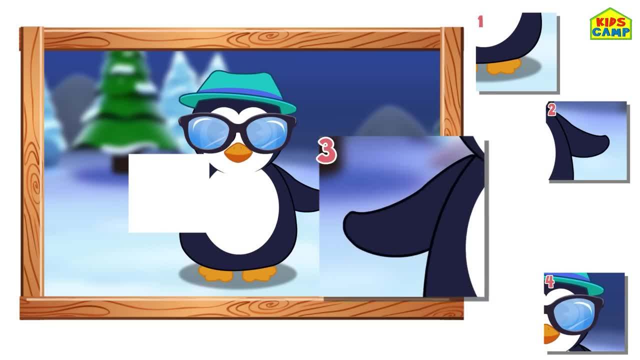 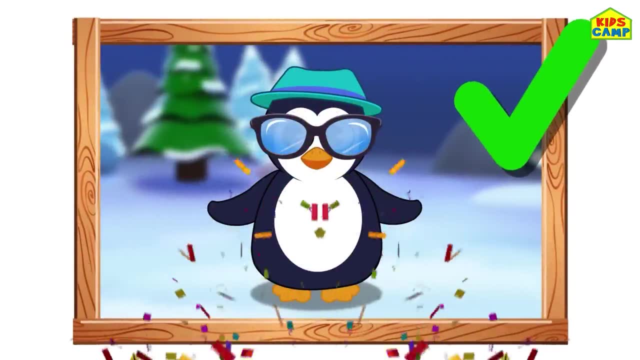 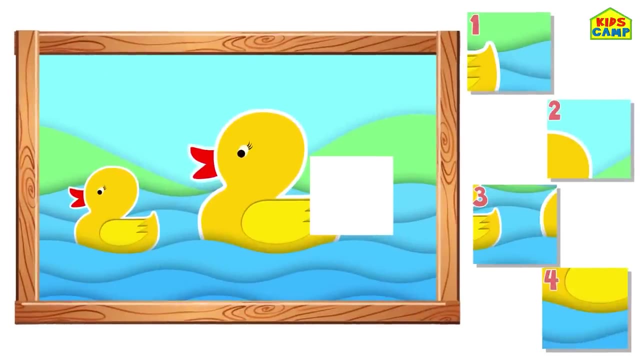 Hmm, let's try number three. Yes, We got the right one. Woohoo, Good job, kids. Let's move to the next one. What is missing from here? Let's try number two. No, Let's try number four. 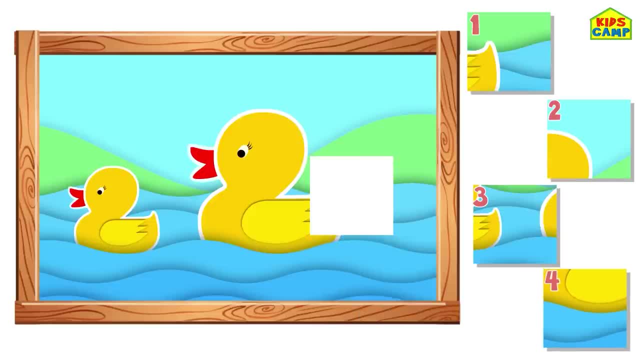 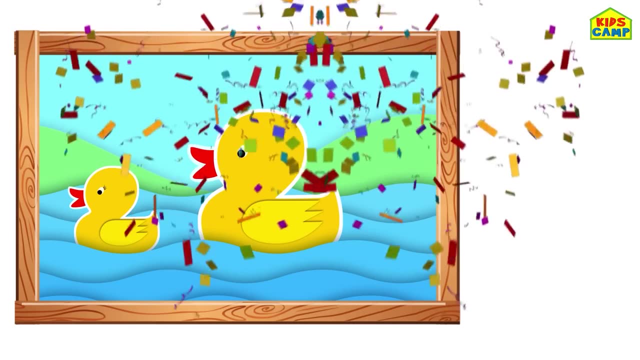 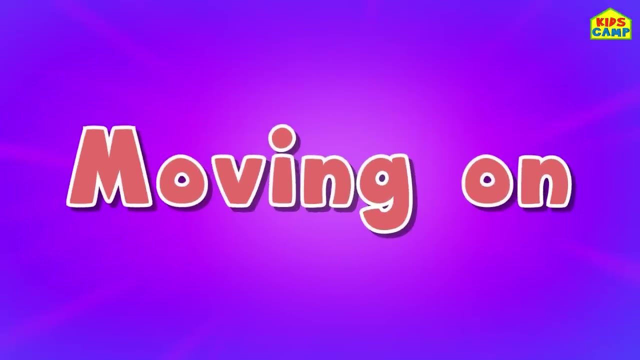 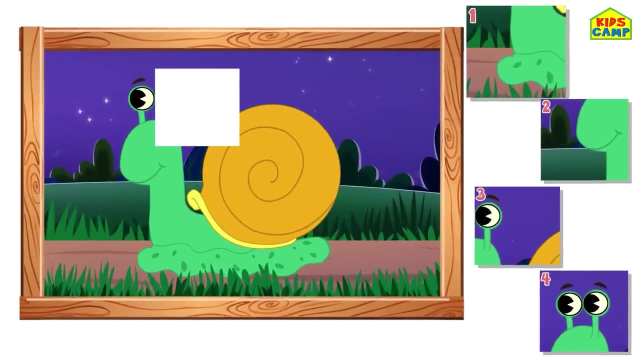 No, no, Let's try number one. Yay, That fits right. We got it. Woohoo, Moving on. Hmm, what's missing here? Let's find out. Let's try number two. No, that doesn't fit right. 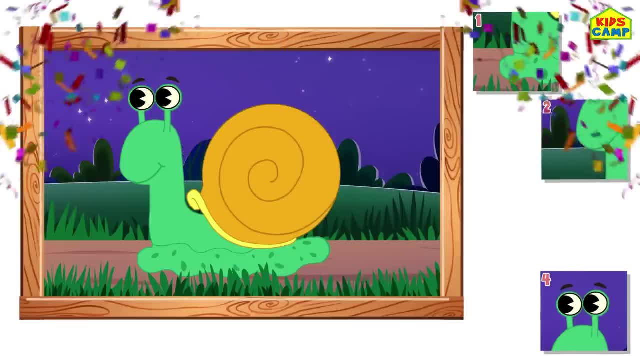 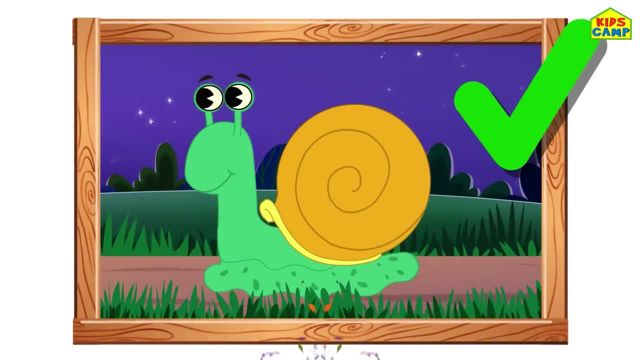 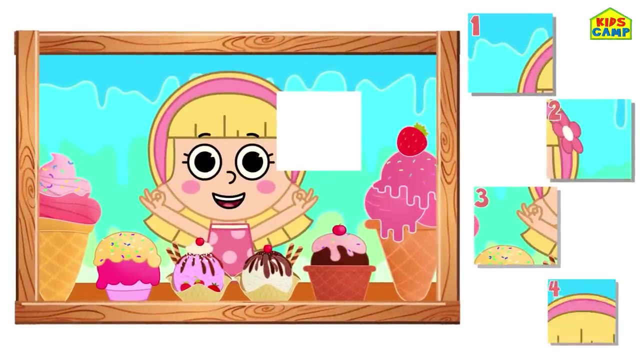 Let's try number three. Wow, We did it. We got that one right, Ready to go up on the wall Moving on. Hmm, what's missing here? Let's try number one. No, that doesn't seem right. Let's try number four. 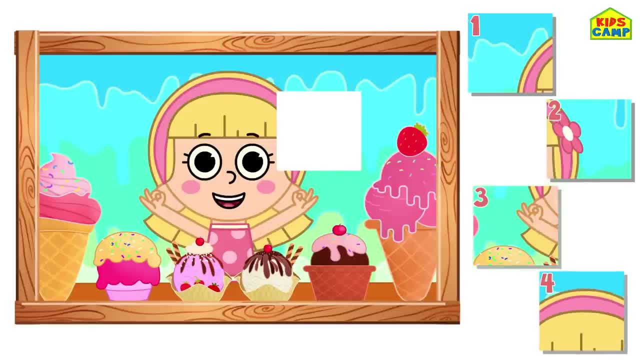 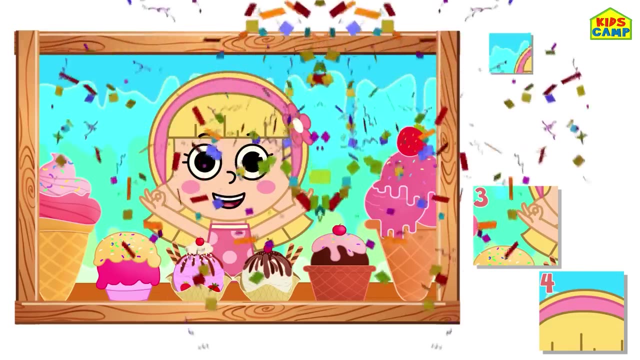 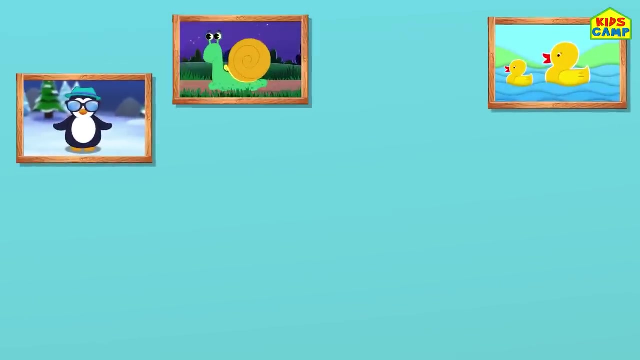 No, no, Let's try number three. No way, Let's try number two. Yes, We spitz ride. Woohoo, We did it again. Good job, kids. Yay, They already look so good up on the wall. 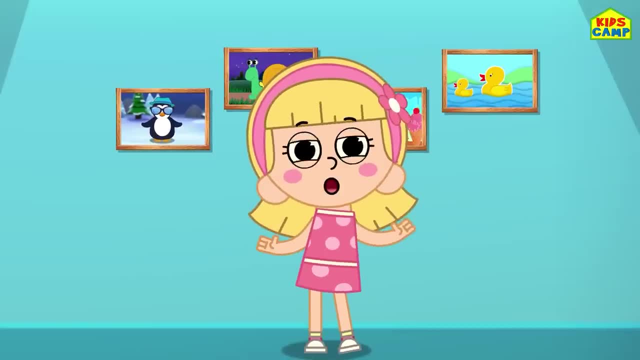 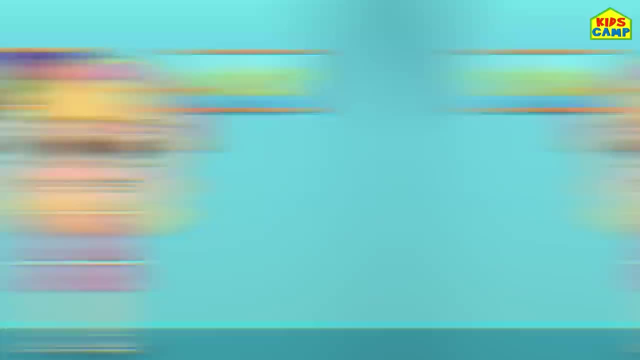 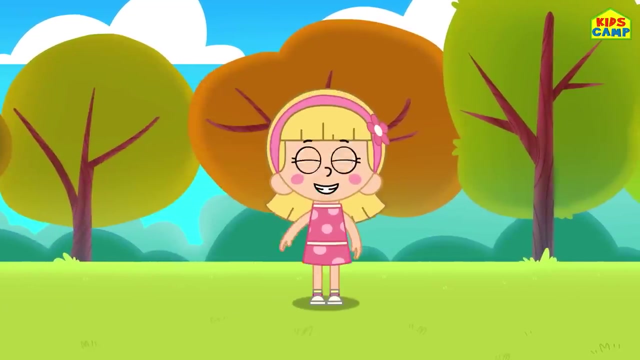 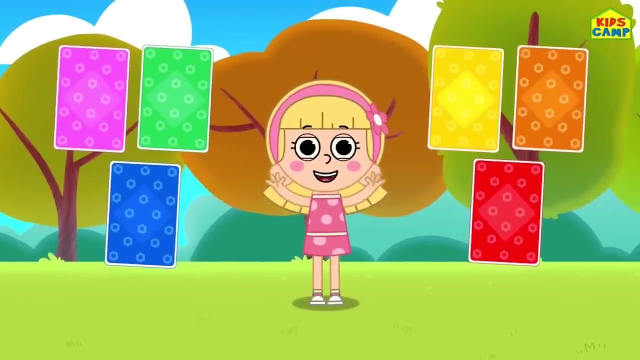 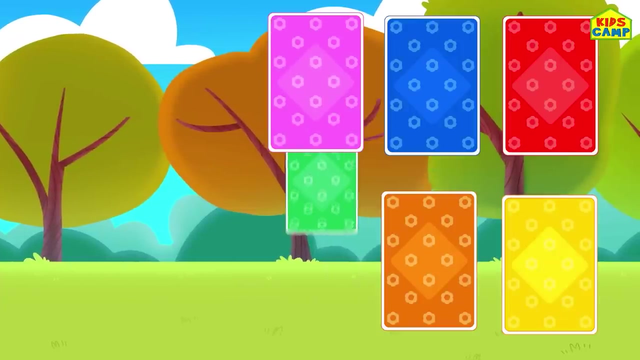 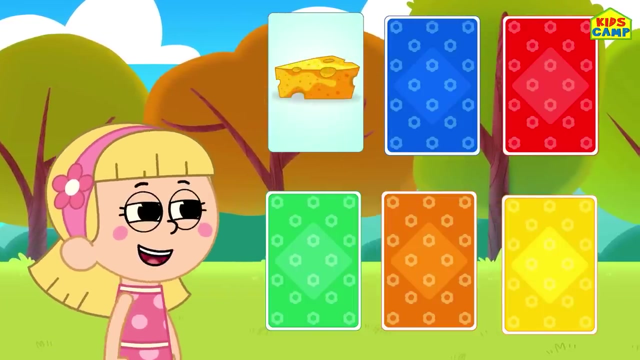 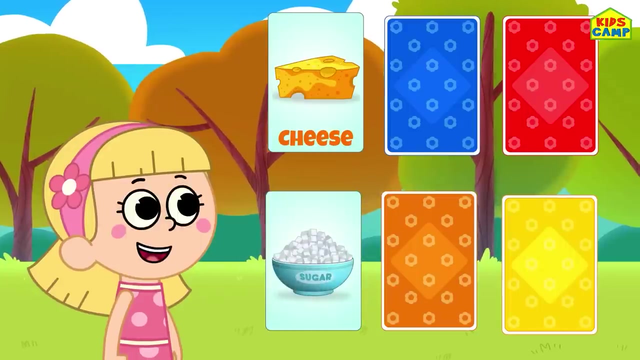 Eva's gonna love this. Thank you so much for helping me out. This was a fun game. Keep watching Kids Camp for more learning videos. Until then, bye-bye, We need to find what cheese is made of. Uh-oh. 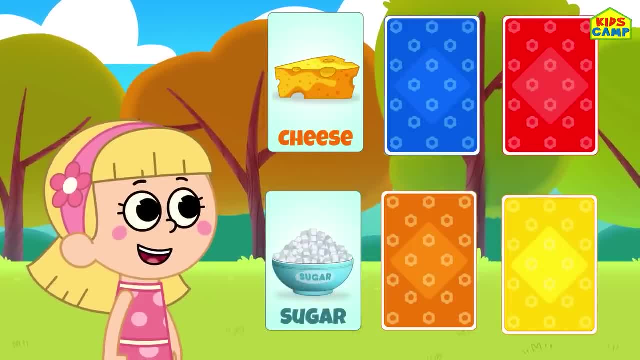 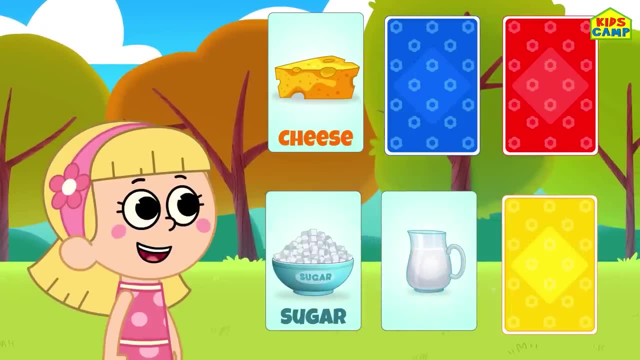 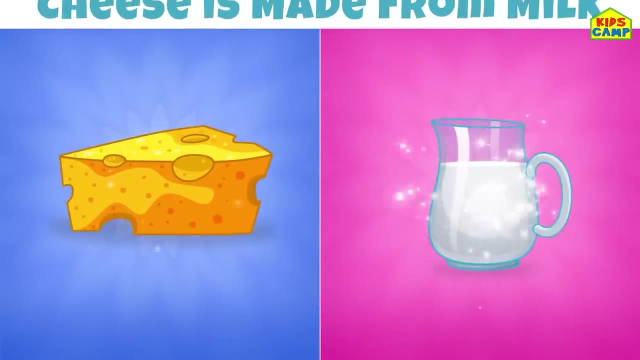 What is this? It's sugar. Is cheese made from sugar? No, I don't think so. Let's flip another card. Hmm, It's milk. Yes, We got that right. Cheese is made from milk. Yay, We got that right. kids. 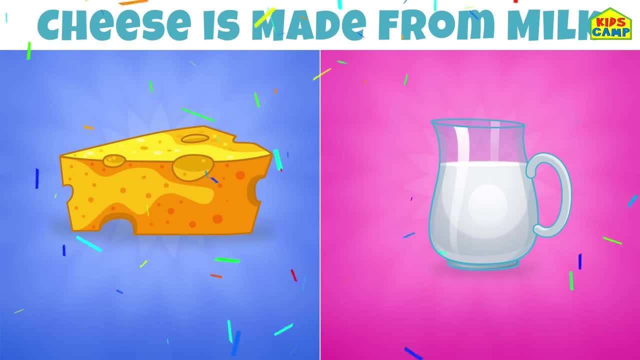 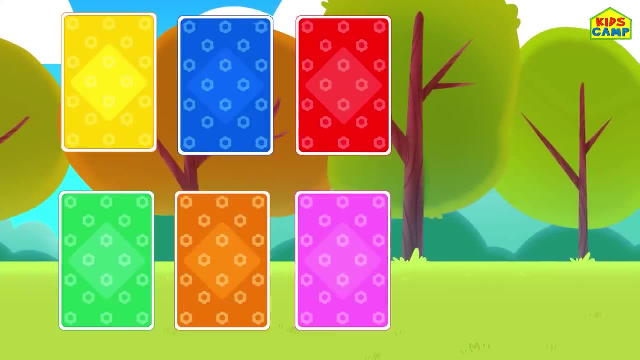 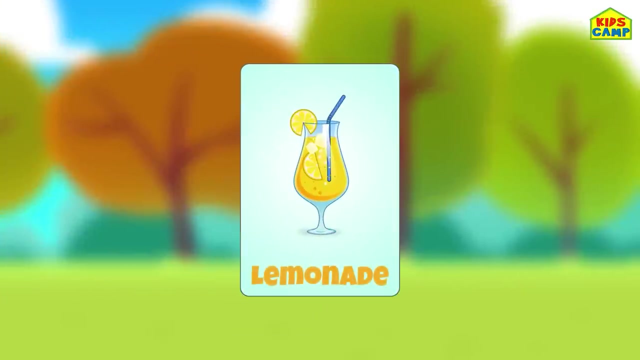 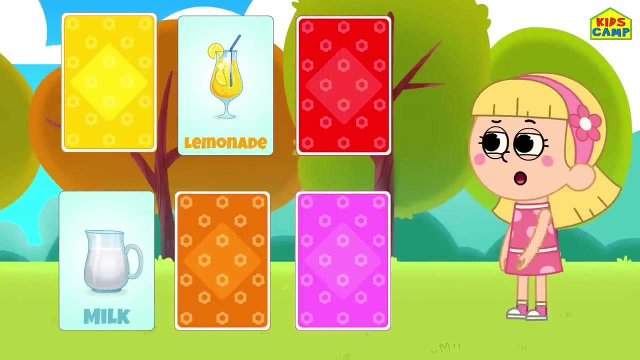 Yummy, Let's find out what's next. Let's flip the blue card. Ooh, What's that Lemonade? What is lemonade made of? Let's flip this card: Ooh, What is this? It's milk. 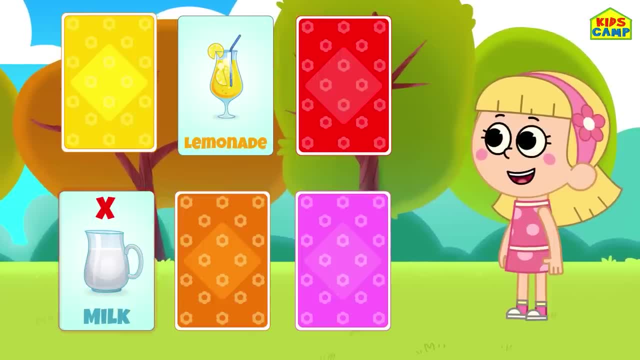 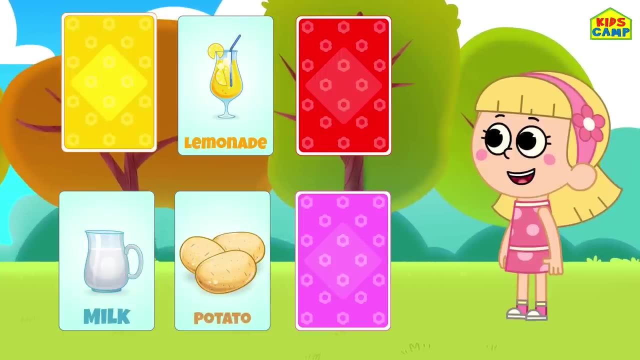 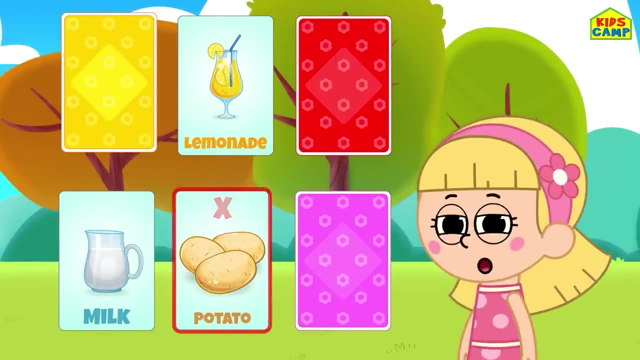 Is lemonade made from milk? No, I don't think so. Let's flip another card. Ooh, What's this? Potatoes. Is lemonade made from potatoes? No, I don't think so. Let's flip the pink card. 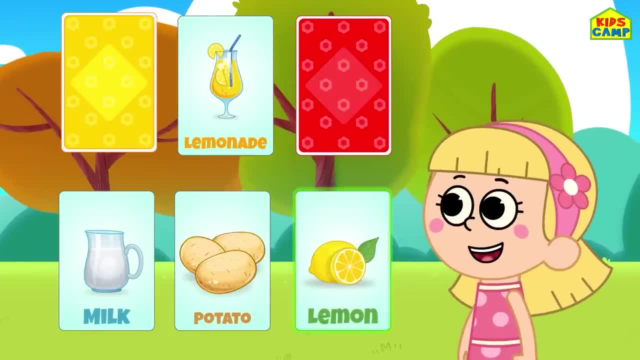 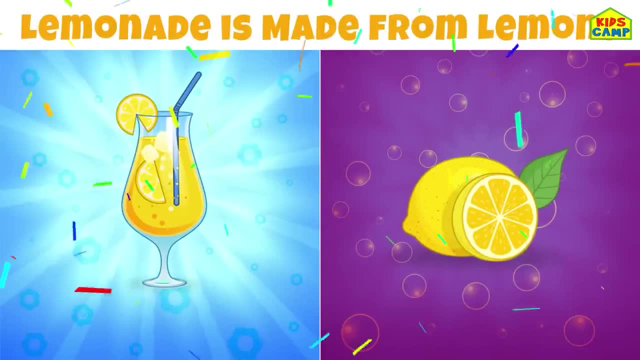 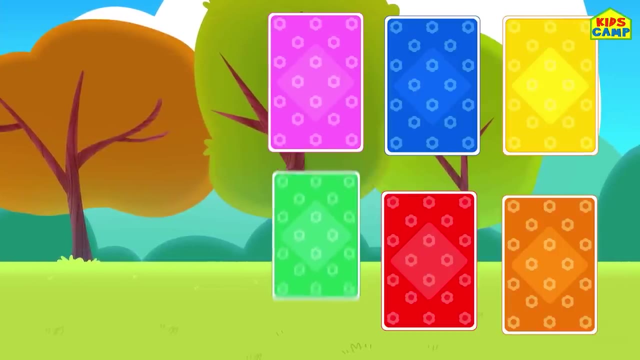 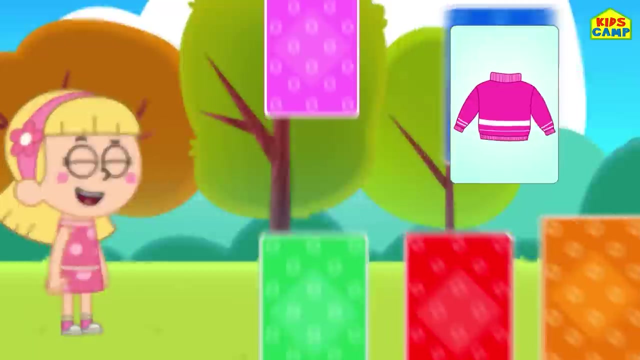 Wow, Lemons. Is lemonade made from lemon? Yes, we got that right: Lemonade is made from lemons. Yay, I like this game. Let's flip the yellow card. Hmm, what's this? It's a sweater. 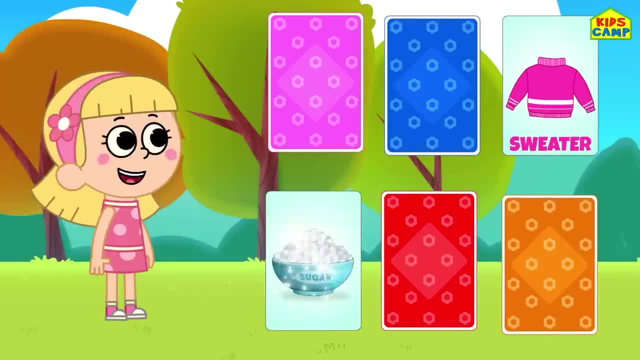 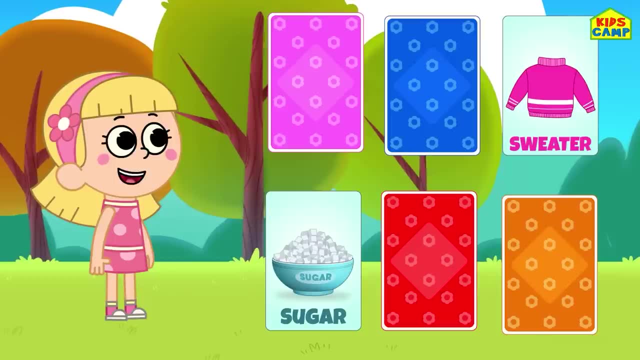 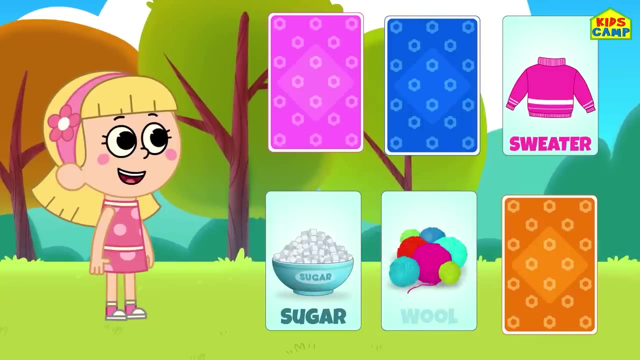 What is a sweater made of? Let's flip a card. Wow, what's this Sugar? Are sweaters made from sugar? No, definitely not. Let's flip the red card. It's wool. Do we make sweaters from wool?